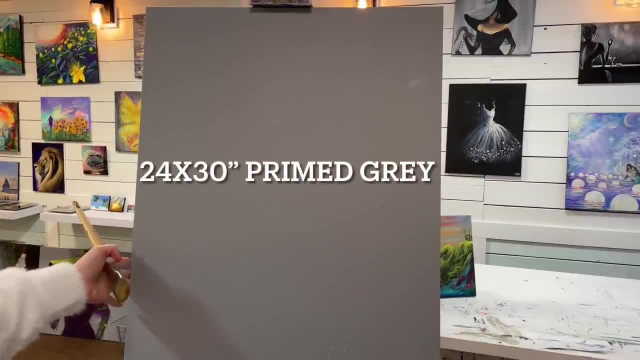 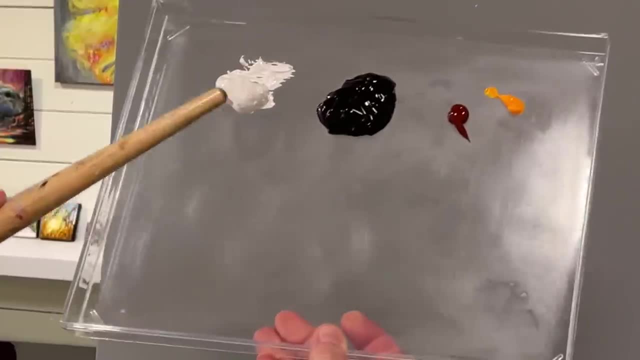 be fun, So I've got a large canvas here. this is a 24 by 30, but you can do this on any size canvas that you like, and the colors that I'm going to be using to start are titanium, white, mars, black, and for the palette I'm going to be using a little bit of all these colors, So I've got some burnt. 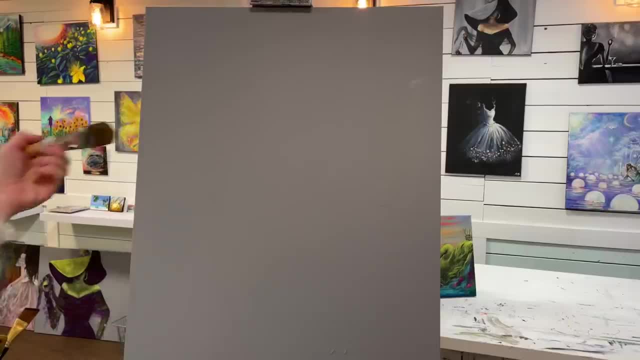 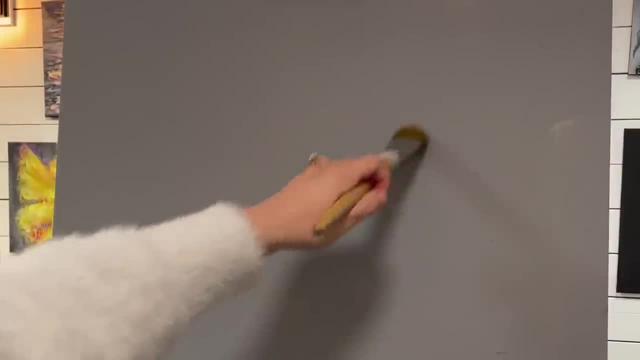 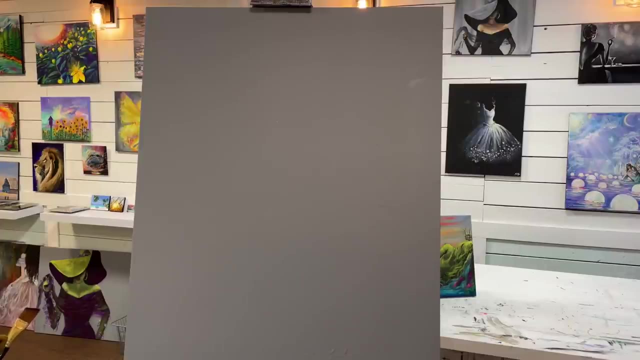 sienna and some warm neon yellow. I've got a number 30 filbert brush here that I'm going to start using to come in with the palette hat first of all. So I want to just get that a little bit wet to start. that'll help me be able to spread the paint around a lot easier. 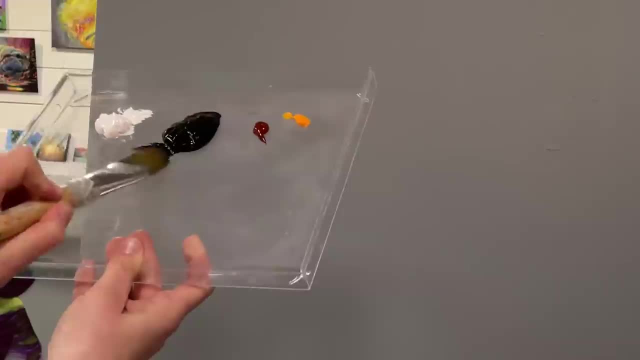 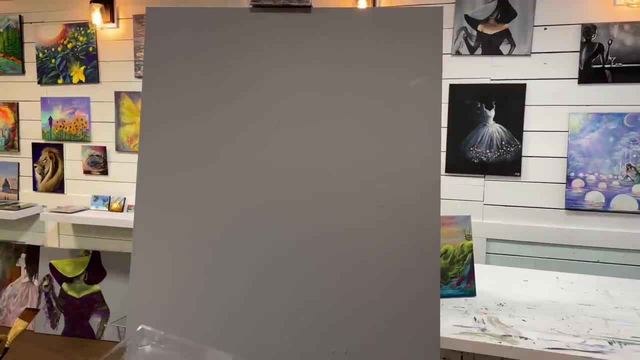 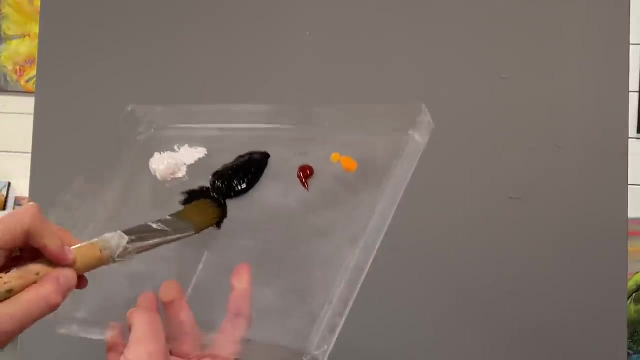 Okay, so the first thing I want to do is take a little bit of black. Oh, I should mention that the canvas I'm painting on I primed it with two coats of slate gray. So again, I'm just going to take a little bit of water on my brush and black paint and I'm just going to think of like a frisbee. 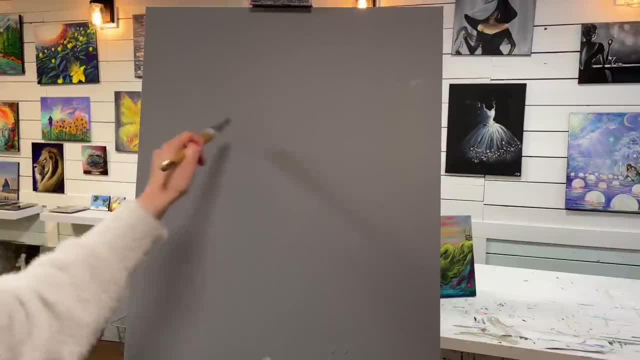 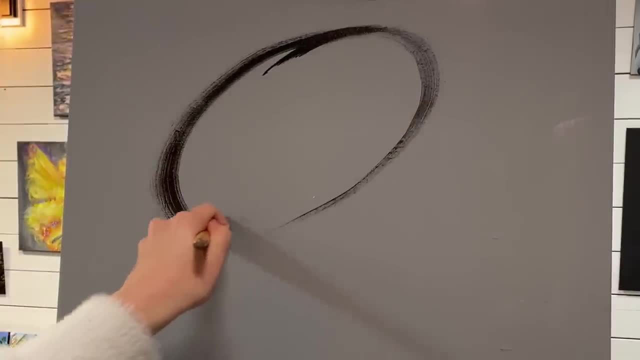 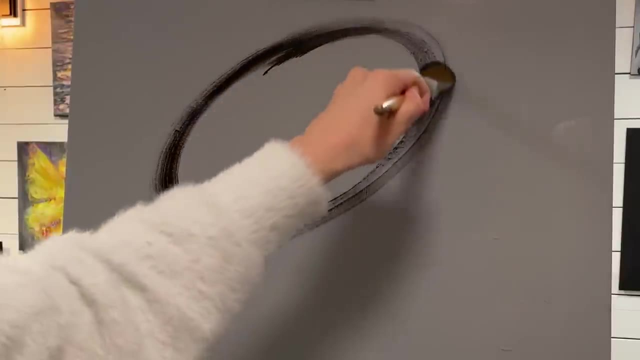 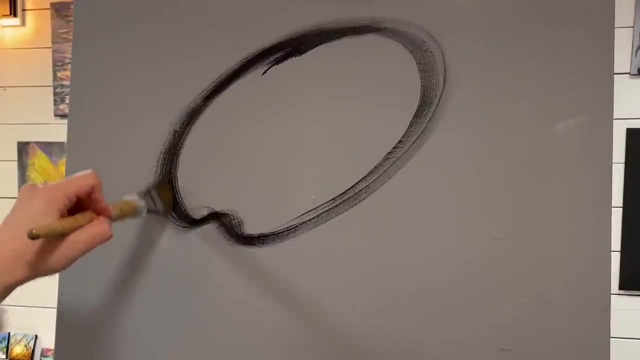 or an oval shape on slanted for a dramatic effect on her hat or for her hat, And then I'm going to go like that, so you're going to bring it in and around, So of course, where the palette goes right there, and then we'll have a little hole right about there. 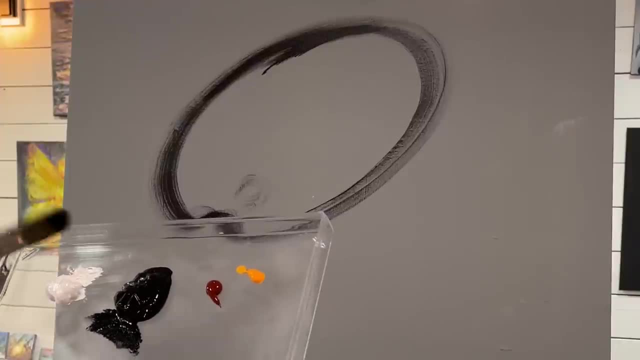 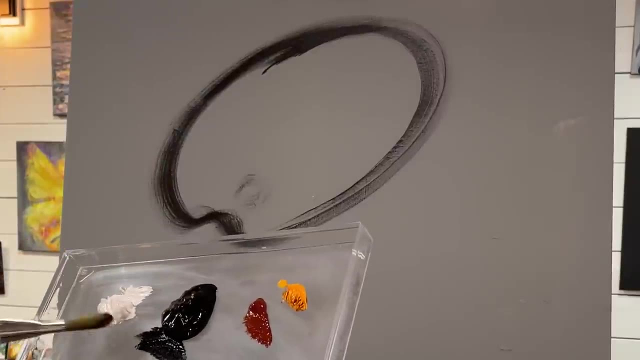 Now the next thing I want to do, without washing my brush off, is just take some of that burnt sienna: a little bit of neon yellow and a little bit of white. I'm not going to mix them all to make one color on my palette, I'm just going to take all of them. 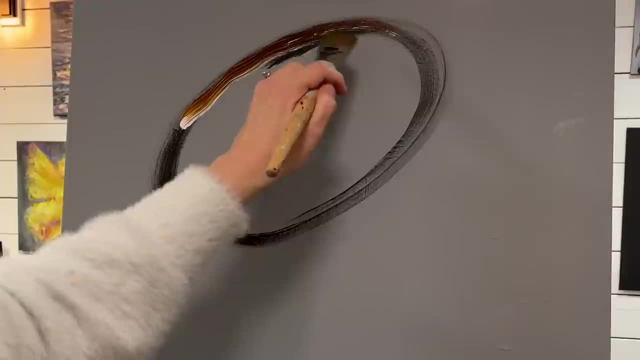 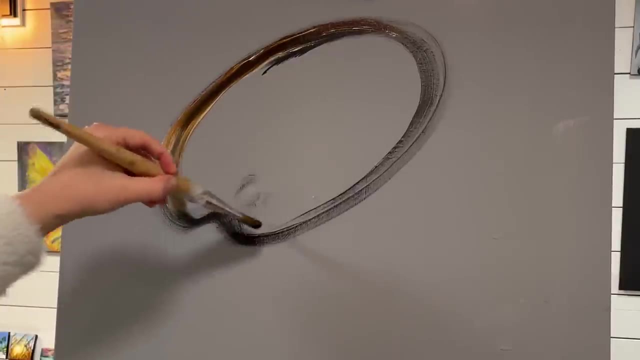 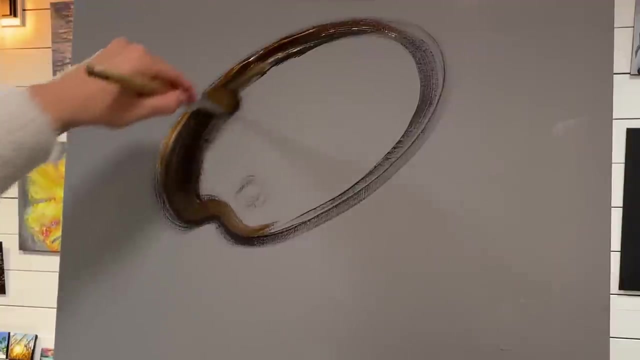 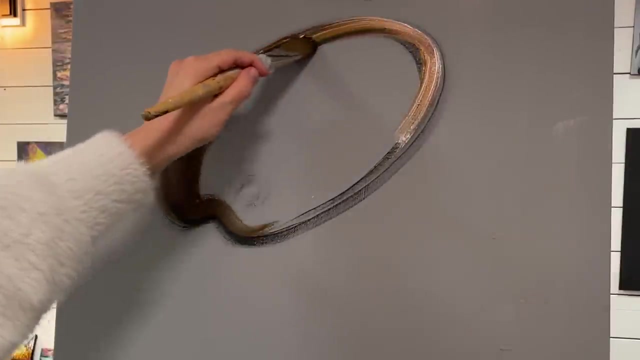 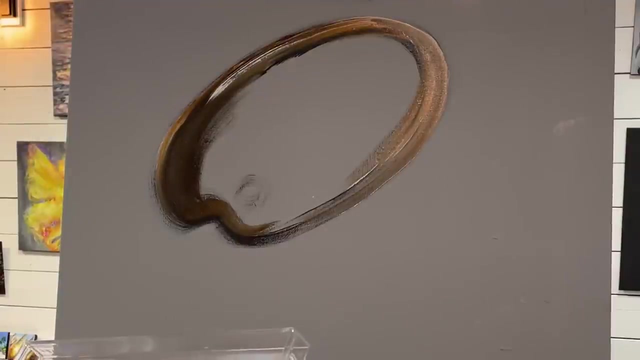 and just start by going around the edge and following that line or that outline. So I'm going to go ahead and go over that browcare back over here, this portion. So I'm going to go in this second bowl here and just actually just repeas to put a little bit of a. 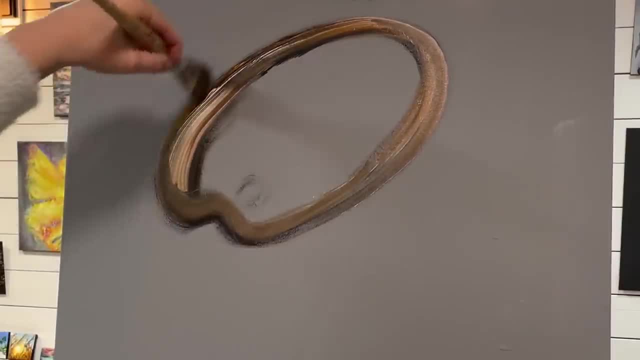 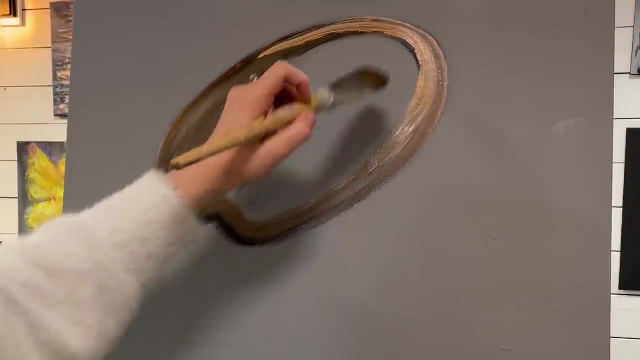 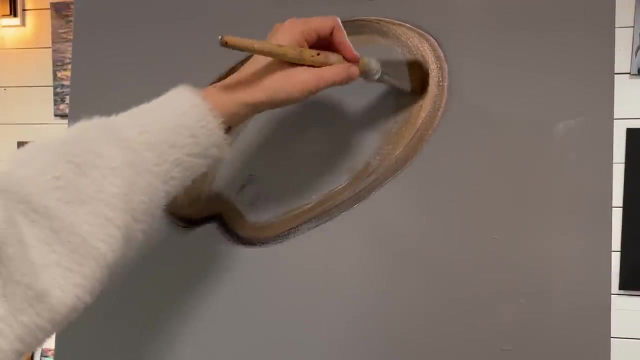 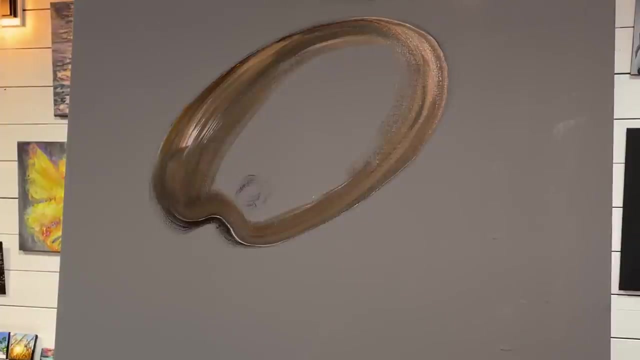 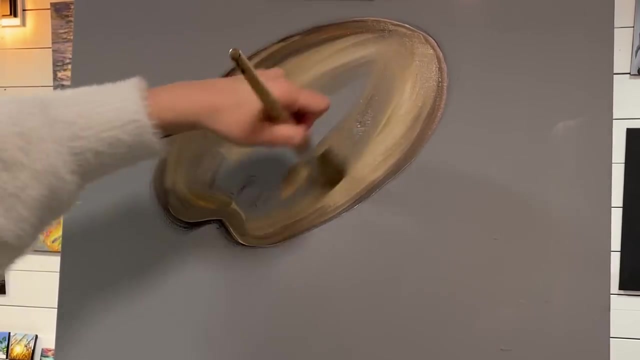 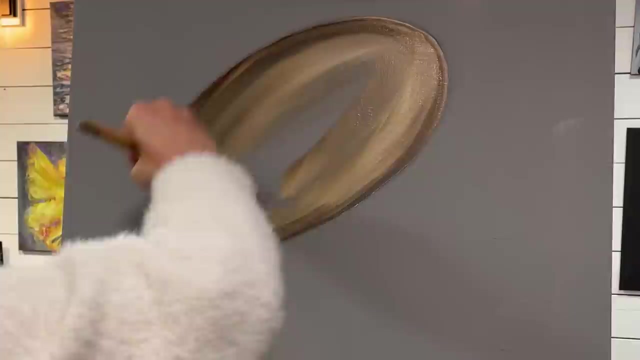 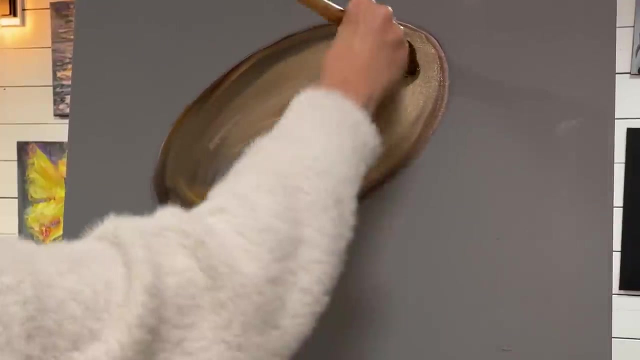 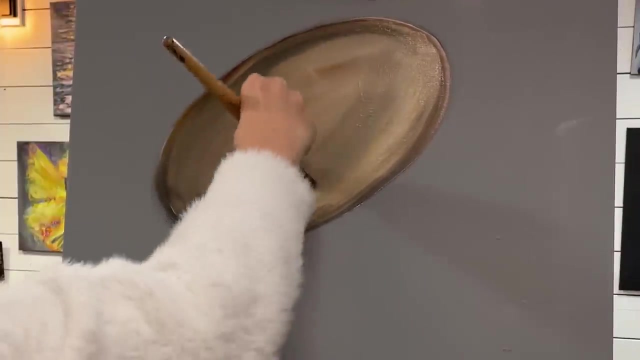 So by having that dark base with the black first as an outline, it's just going to make our palette look more 3D. All right, so we're going to go ahead and get started. All right, so we're going to go ahead and get started. 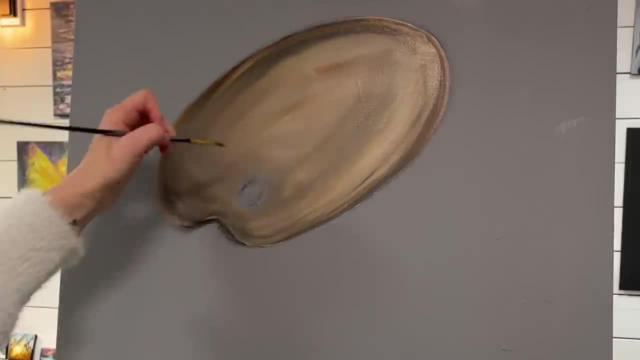 All right, so we're going to go ahead and get started. I'm going to get a little bit wet, take a little bit of black and then just add a little opening right there. Of course we've got that little hole here that you put your thumb through so you can hold the palette. 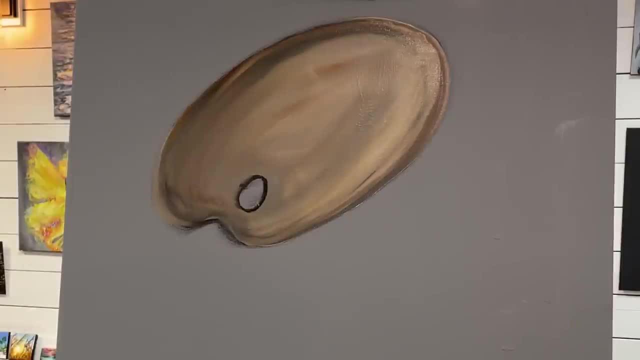 I don't know how many people out there still use a palette like this. They're not that easy to find anymore. I'm going to take my number. I'm going to take my number- nine filbert now, and I'm going to go around the outside. 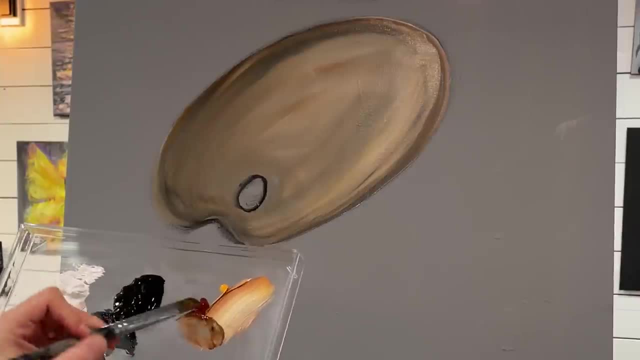 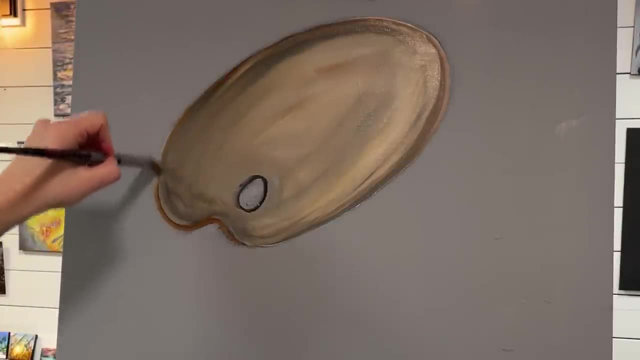 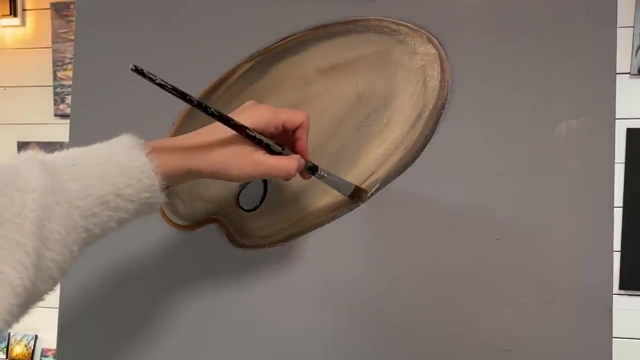 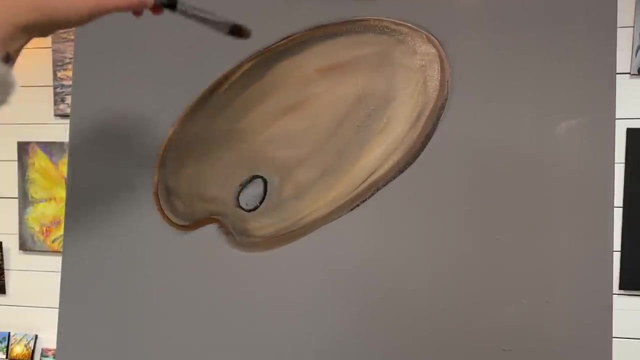 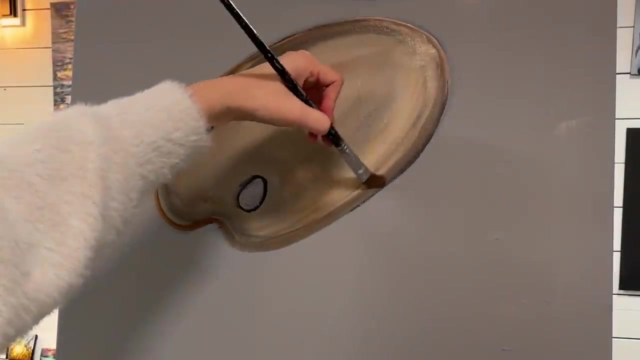 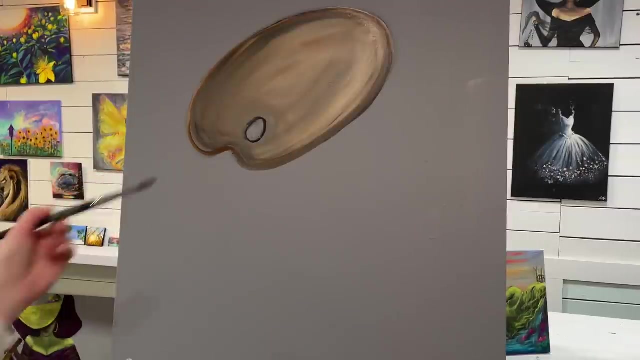 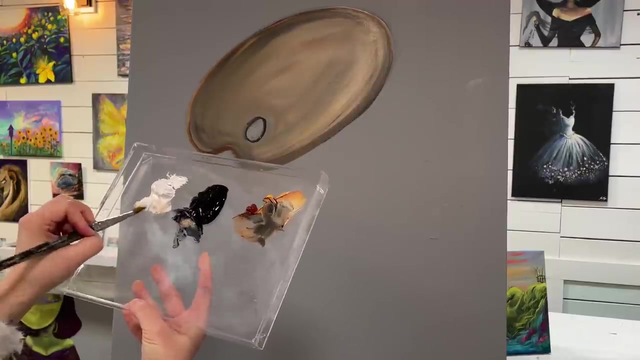 A little bit of all those colors, a bit of black, the white, yellow and the burnt sienna, And I'll just outline And I'll just outline And I'm going to continue using my number nine, filbert, here. so what I'm going to do is take white. it's tinted a little bit with that brown tan color, that's okay. 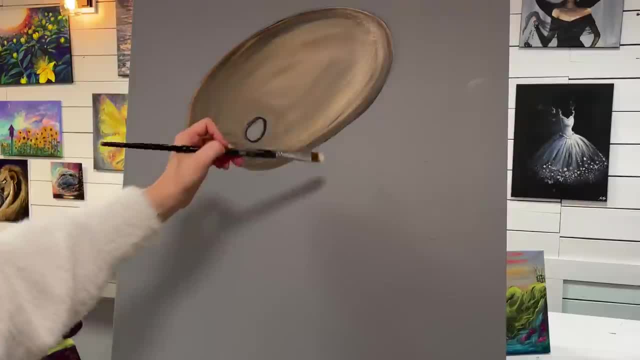 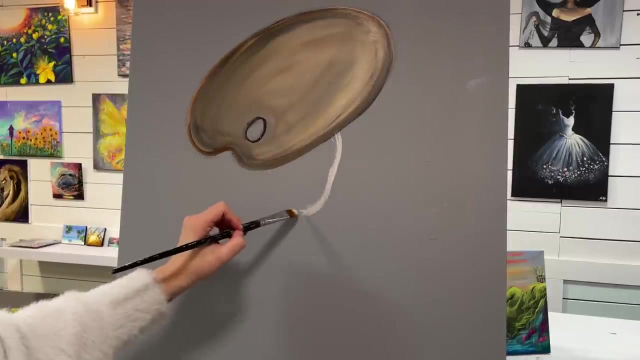 though, and I'm going to start off the edge here- about halfway across the hat, kind of in the middle area here. so we've got our cheekbone that comes out a little bit and then it gets narrower right here we'll go across for her chin and then up. I'm going to scumble. 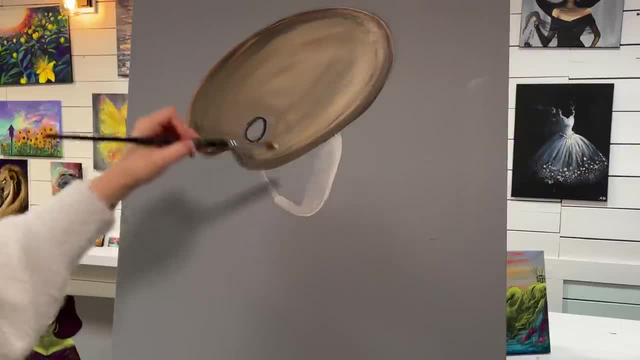 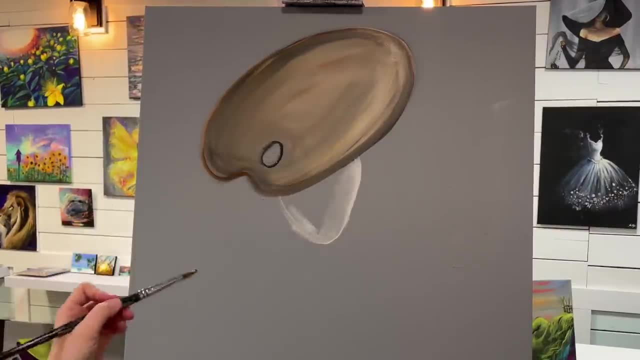 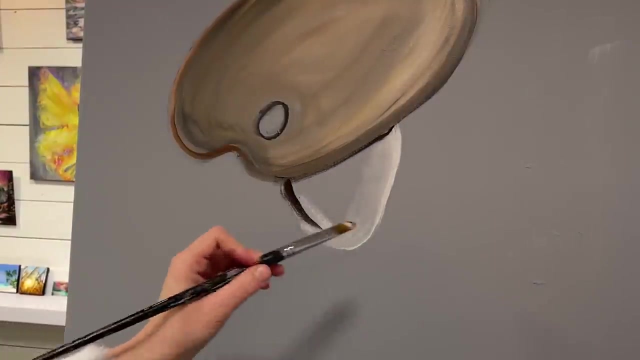 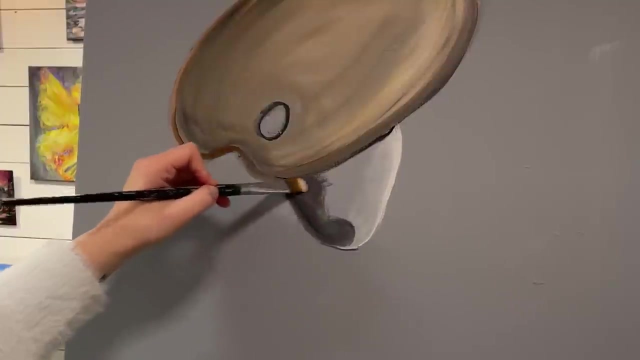 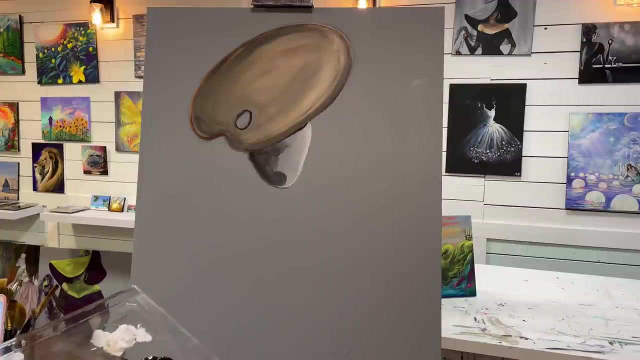 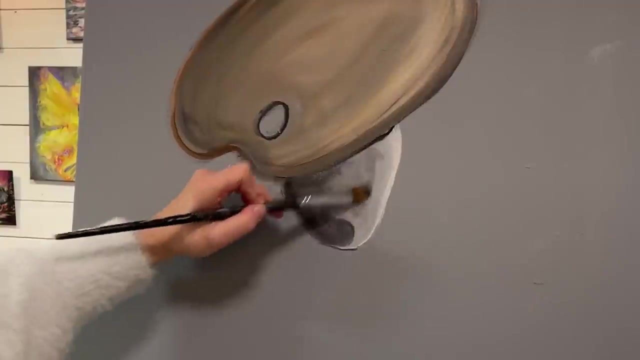 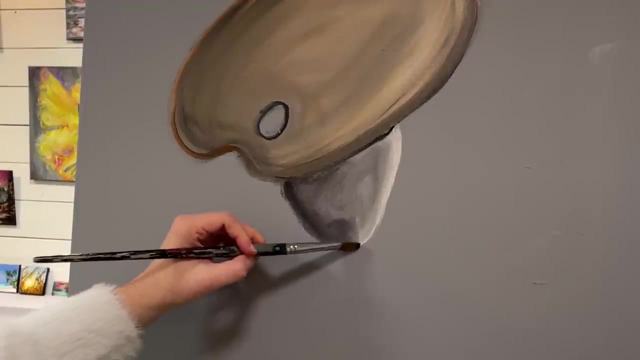 okay, I'm going to take a little bit of black now shadow on this side. so I'm gonna go right under, come down here, right under her chin, bring it over. I'm gonna wash all that paint out of my brush and then just soften when gently right down here where it comes down underneath her chin. there. 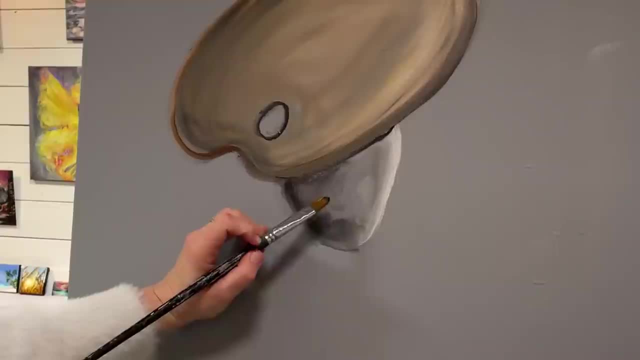 I'm just going to take off a little bit of paint right around her mouth and also apply the light to some of the important spots where she needs me to be. so after she's done spraying, she will use a white color shades from our figura black powder palette palette. you can find this off in the ebay stores also, and also i'll put a link to the. 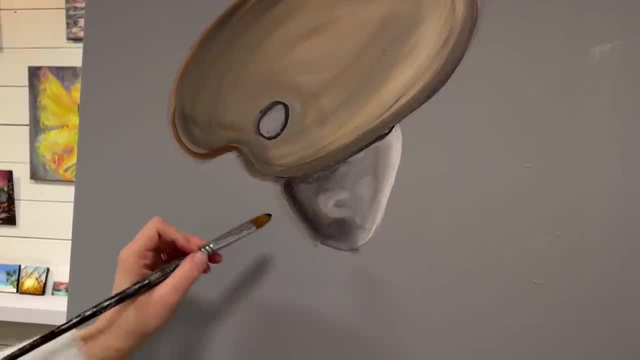 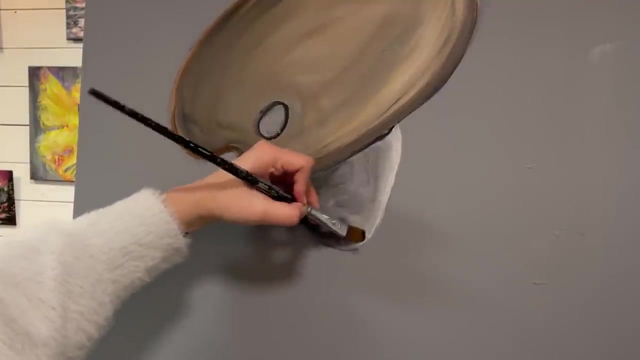 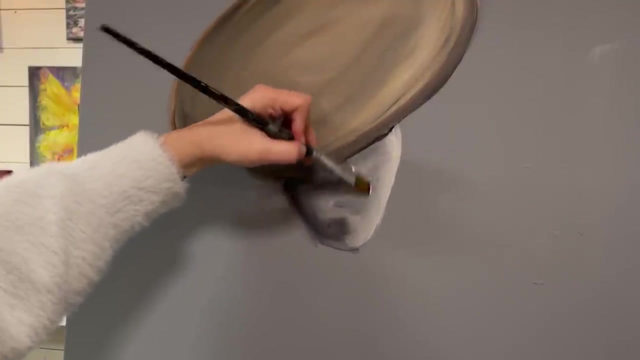 add a little bit of white to help me do that. all about adding those light spots and dark spots for the shadows and just kind of shade in the basic outline of the features. and if you approach it like this, then before you know it you'll have a face without even trying too hard. 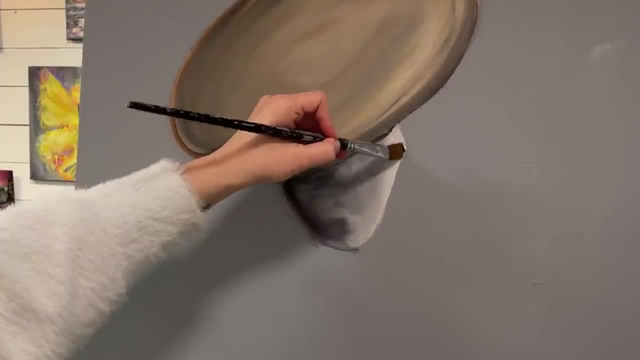 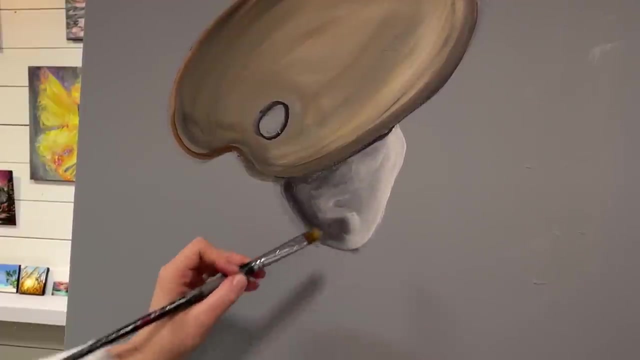 bring the cheekbone out a little bit here on the cheekbone to come out a little bit and then have it go in like that, where it goes in towards her eye, right under her nose, under her lip. it's gonna be a little bit brighter there and then just graze. 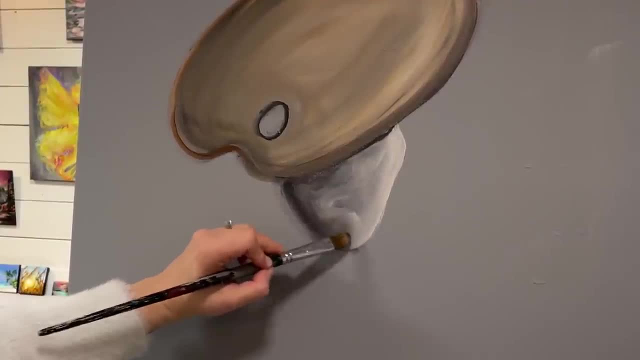 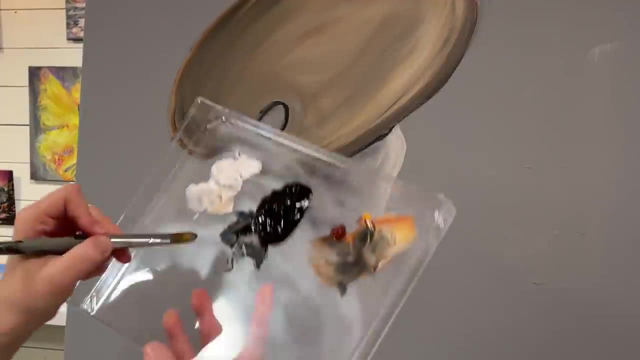 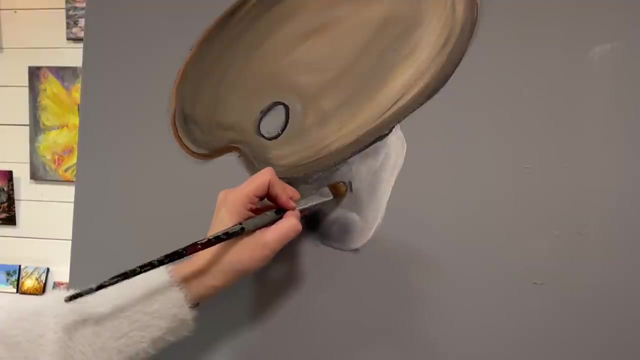 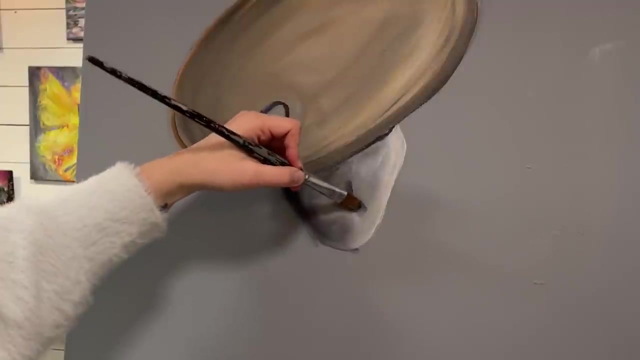 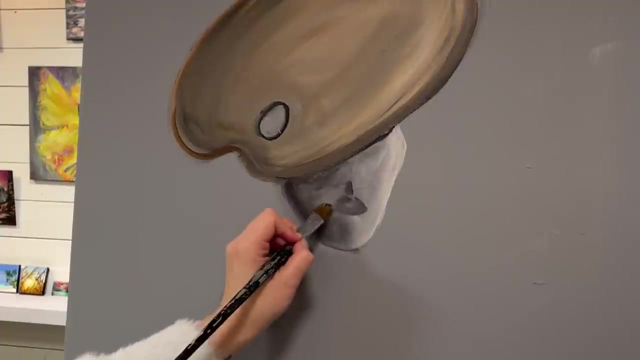 over, just soften that area. I'm gonna make a dark gray color. I have a little teardrop shape right here gonna bring all of that back in here, go down on either side. for the top lip. we're going to take a little bit of white, kind of go around, outline the little. it's just a little divot. 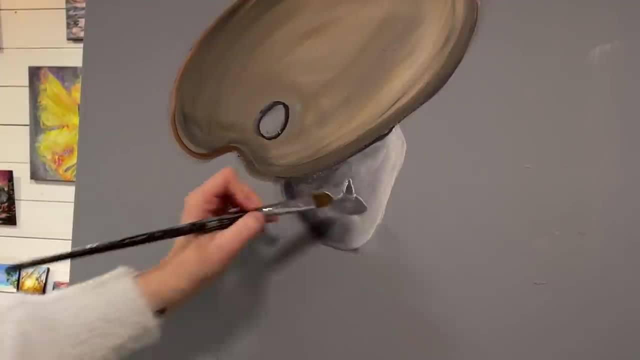 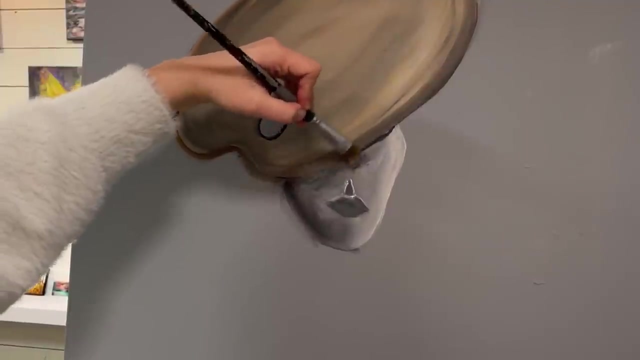 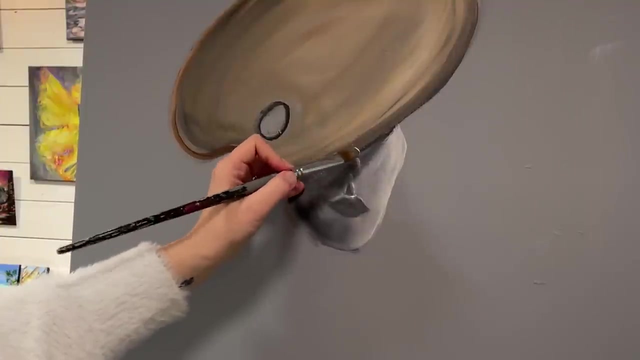 in between her nose and and her lips, then this is going to be in shadow here and we'll just see a little bit of her, her nose area. so we'll just have a little bit of her nose area. so we'll just have a little bit of here. 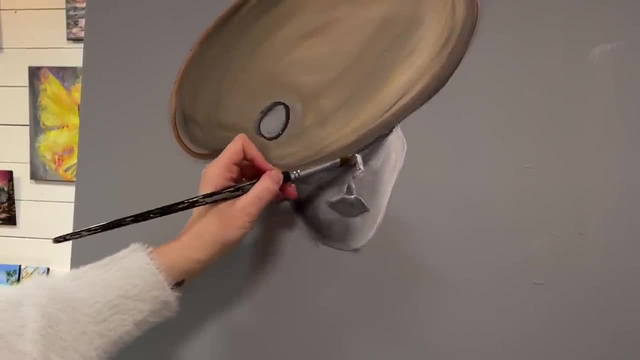 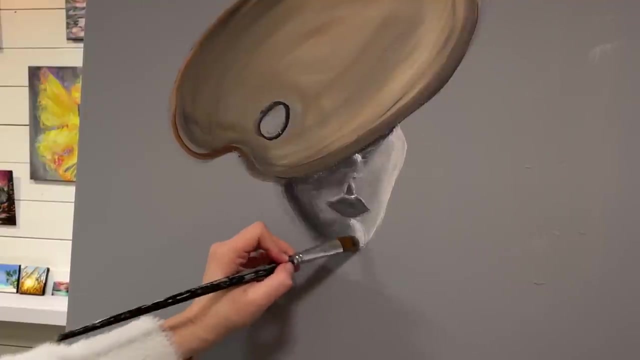 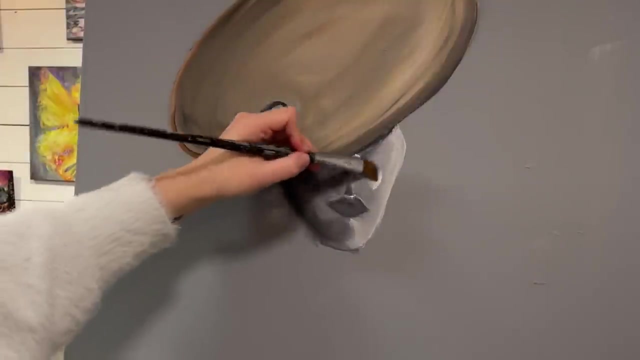 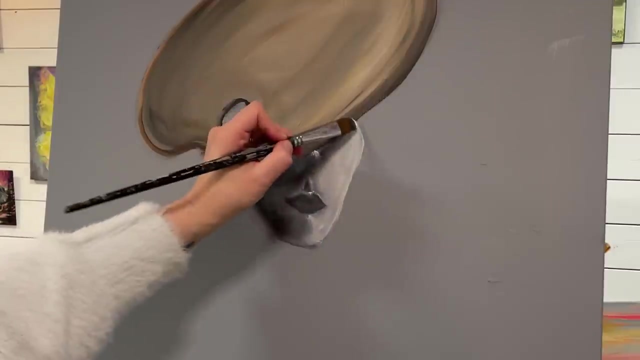 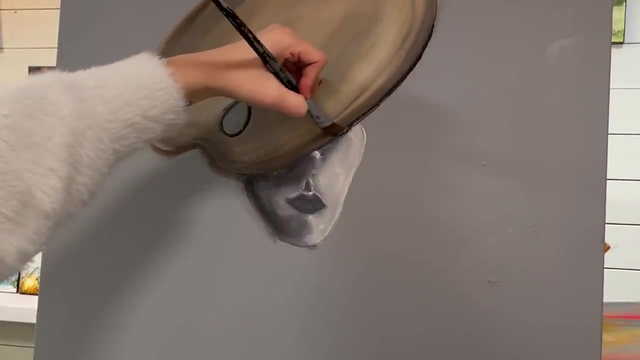 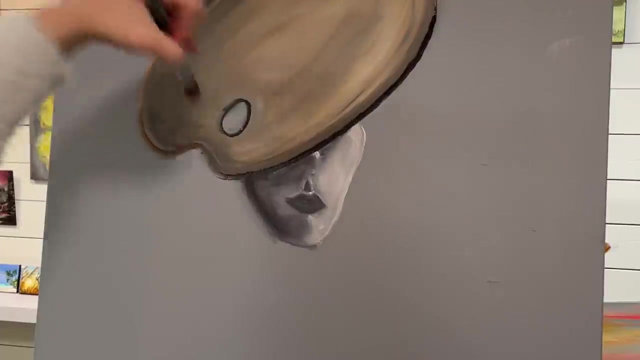 here a little bit more white, and i'll just reapply these highlights. as they start to dry, they get a little bit darker. I'm just going to bring the hat down a little bit more now so we can clean this up over the face and have it look like it's more in shadow in this area here. Okay, I'm just going. 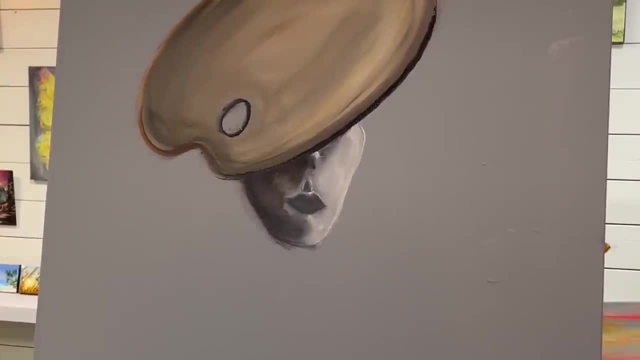 to wash my brush off. Soften a little bit more white. I'll just dab some white inside her mouth. lighten it up a little bit. Okay, I'm going to keep going. some white right here under her jawline and neck. 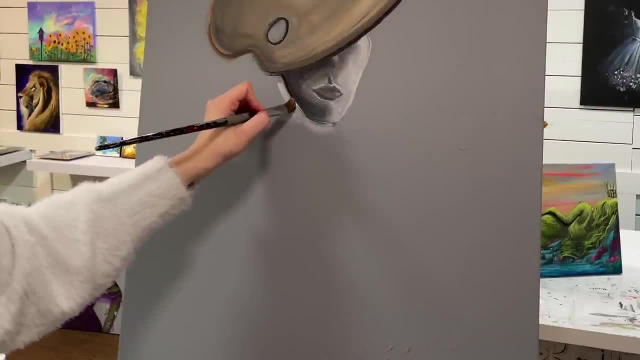 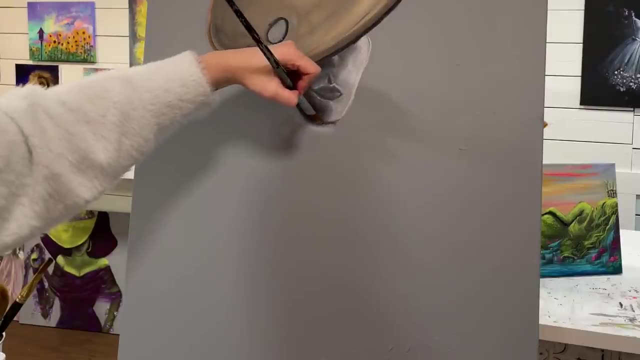 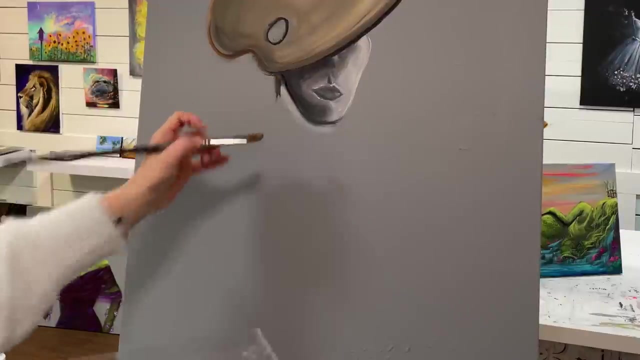 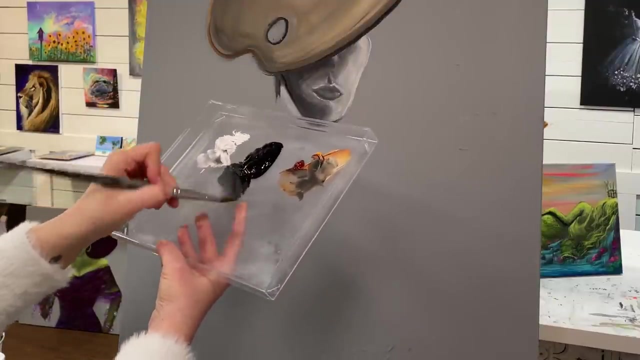 Okay, And a little bit of black Smooth that out. Come in with her neck right here. That's going to go on a slant. I'm going to get a little bit of water and white on my brush. Make a dark gray, as long as it's darker than the background. 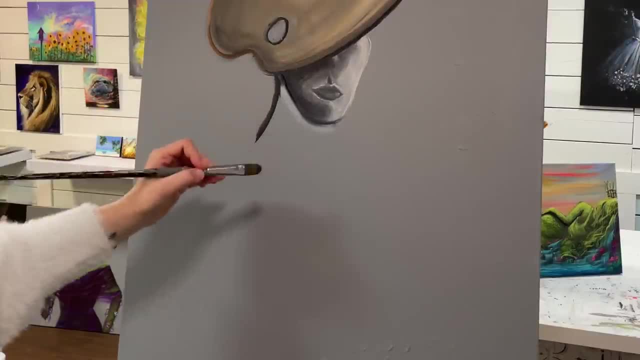 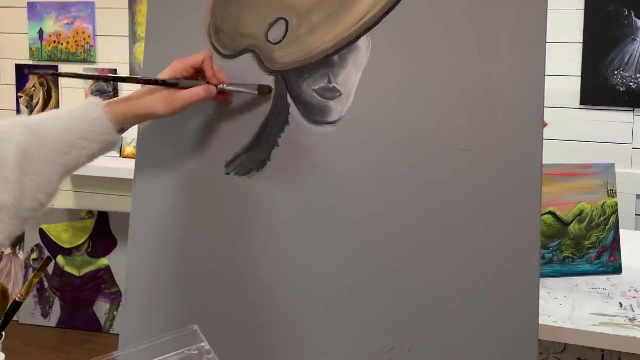 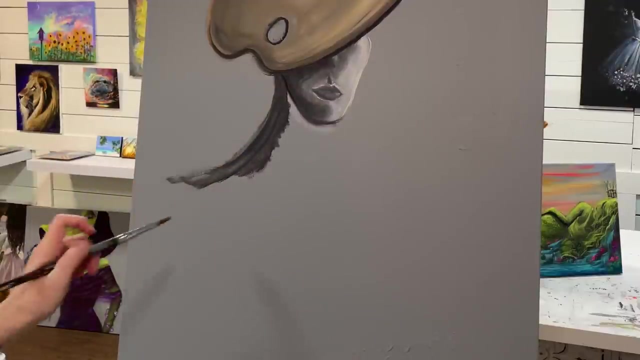 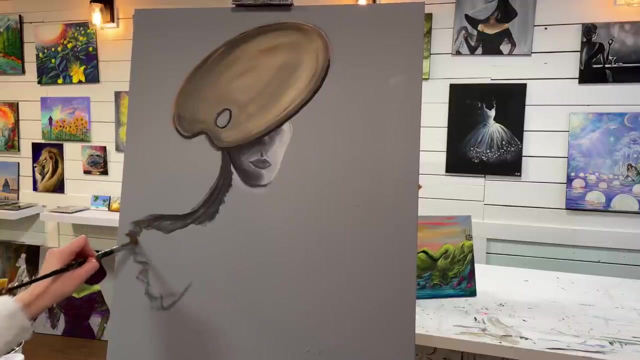 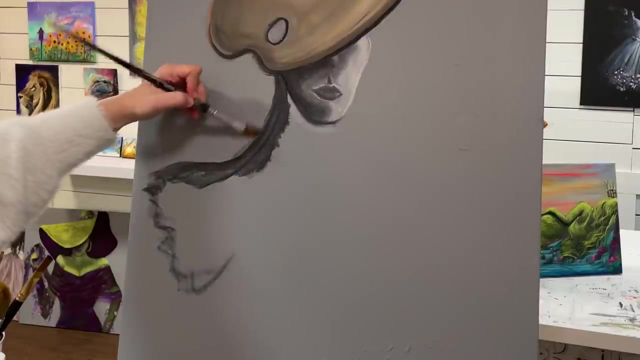 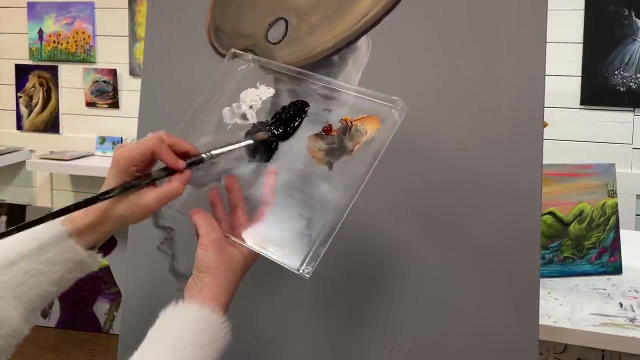 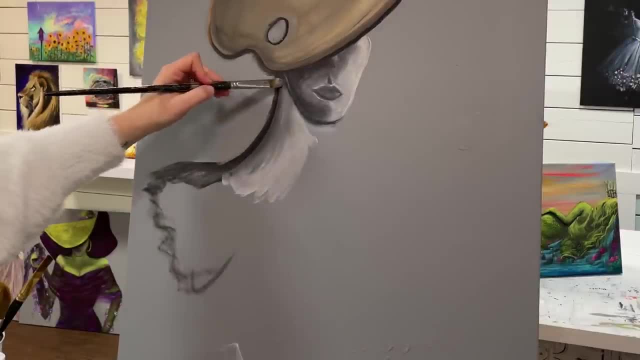 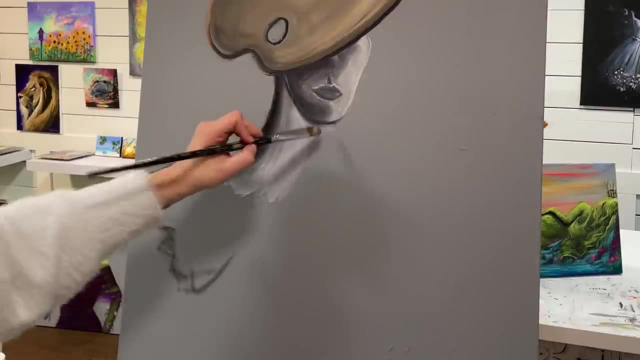 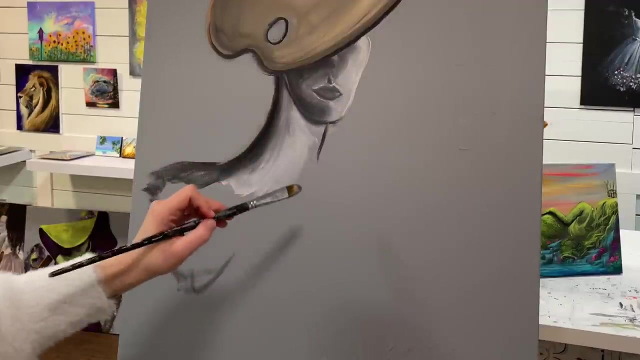 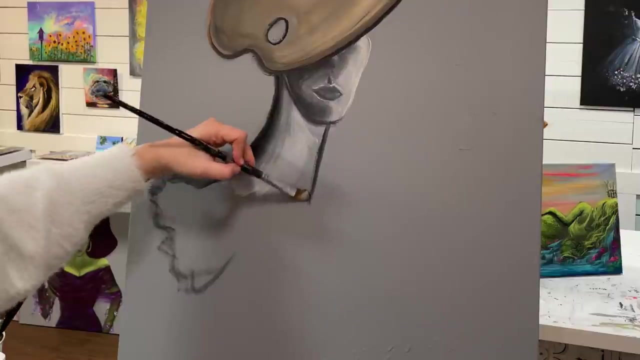 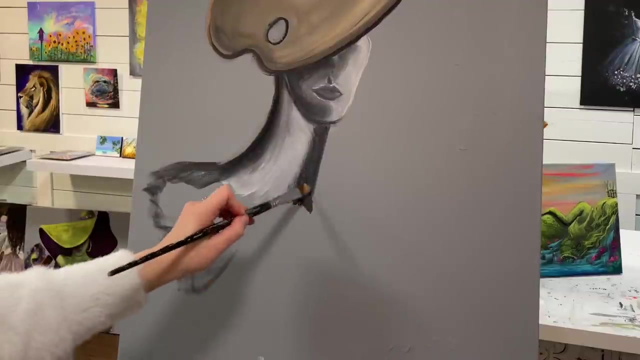 We're just going to come in with this light shadow, gradually build it up in the middle Multishades and tones of grey. So right about here, halfway across her chin, we're going to go across like that kind of on an angle here for the rest of her neck. 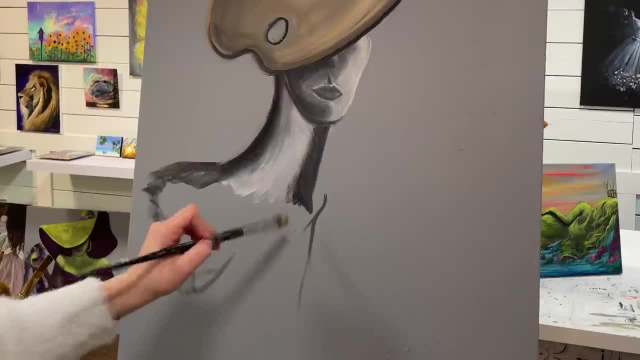 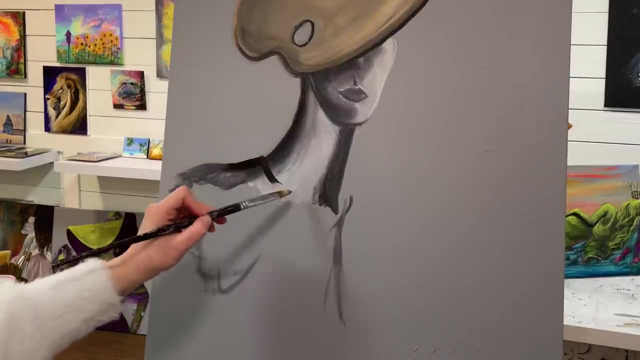 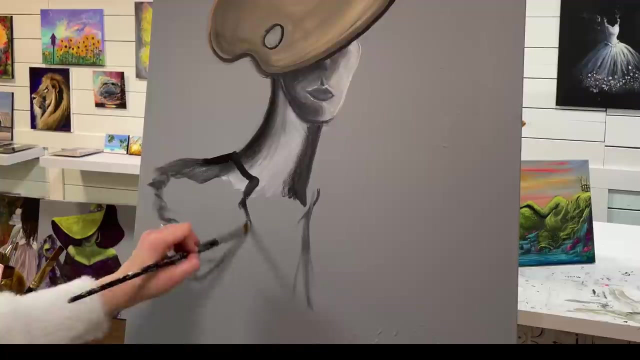 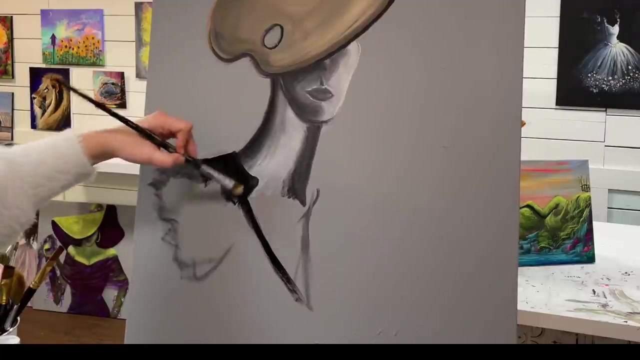 Okay, We're going to come in with the collar of her shirt right about here, so I'm going to go above the skin scoop, then come down here for the collar and then the v-neck. Okay, We're going to take some water help thin this paint out. 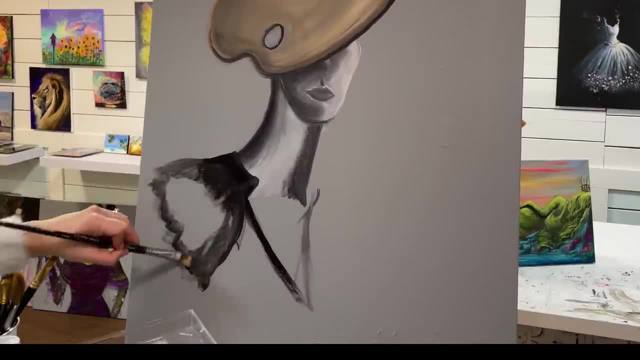 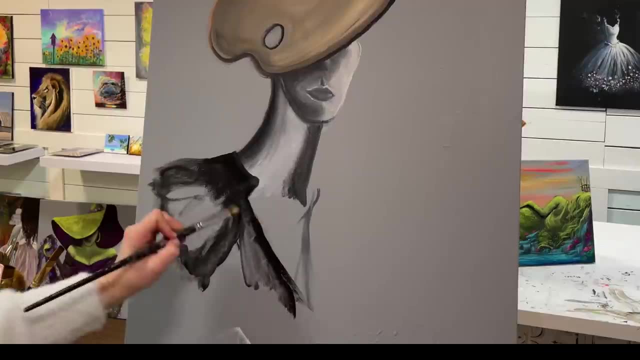 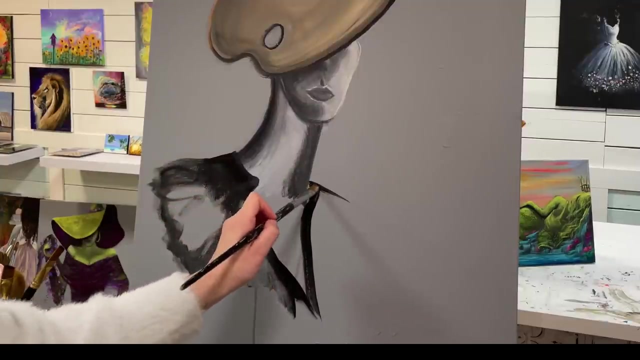 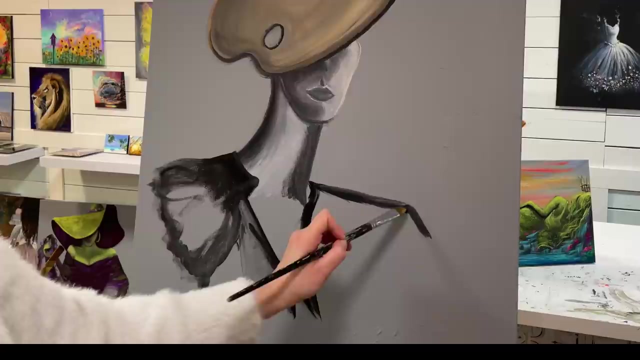 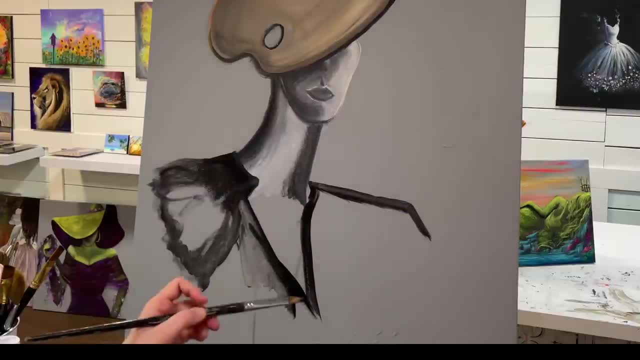 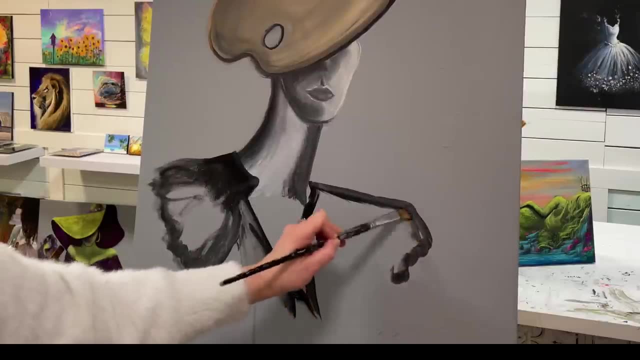 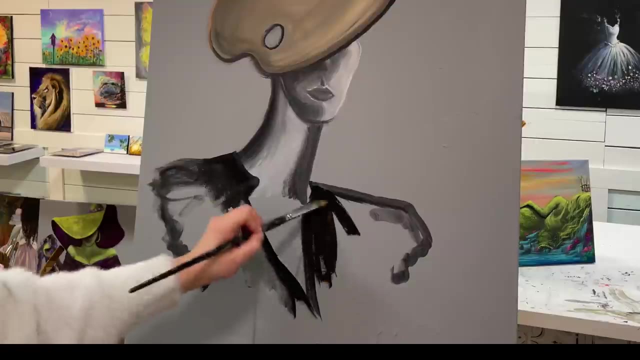 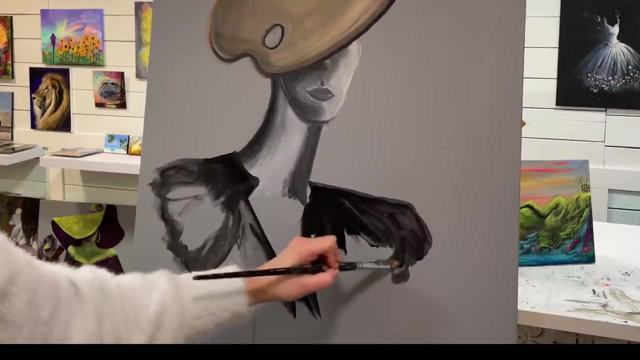 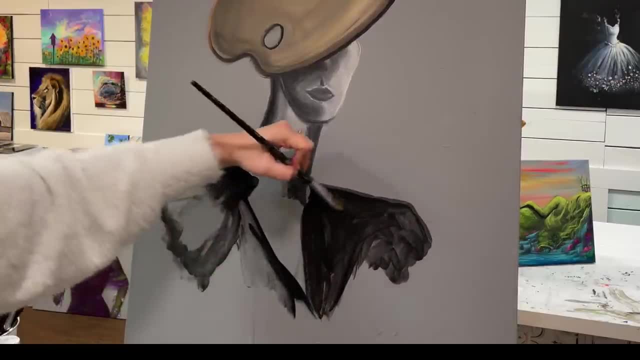 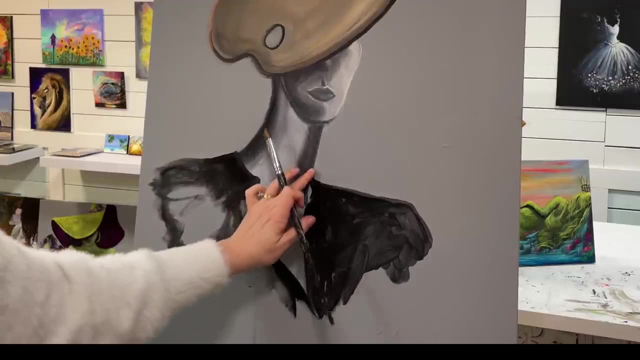 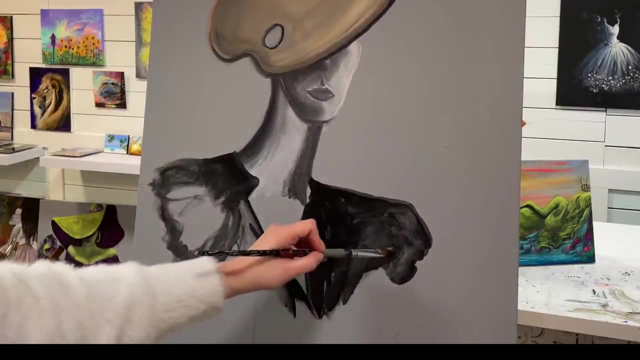 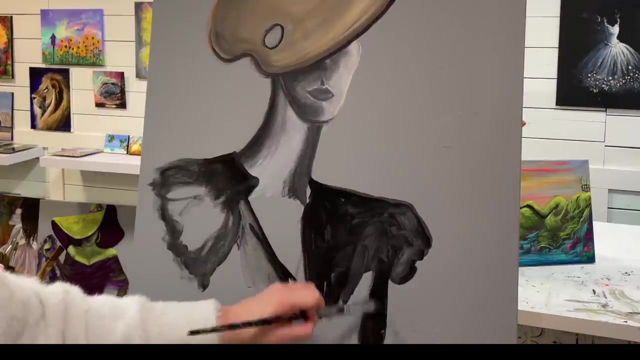 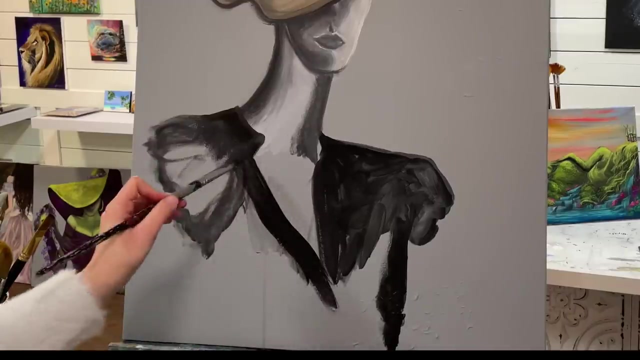 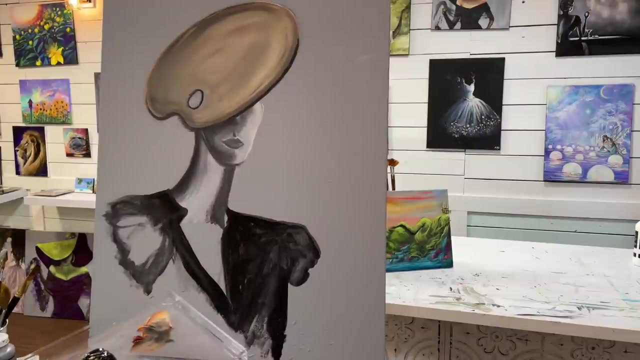 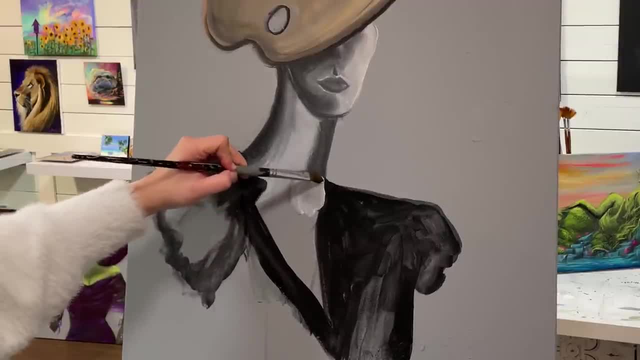 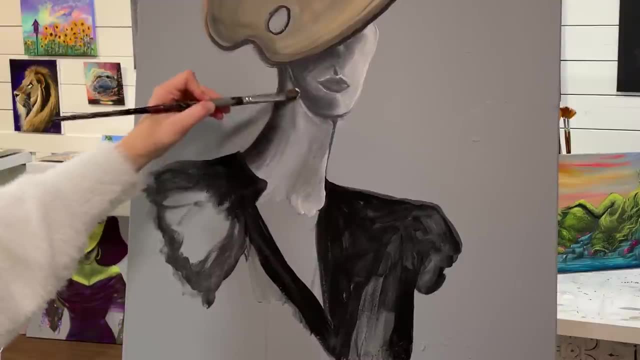 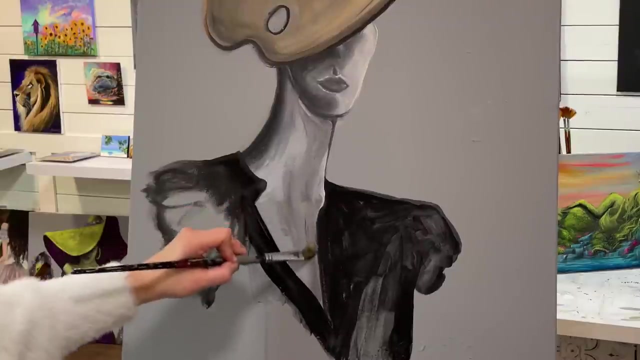 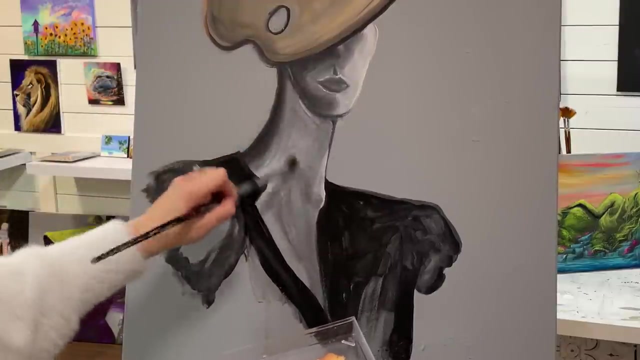 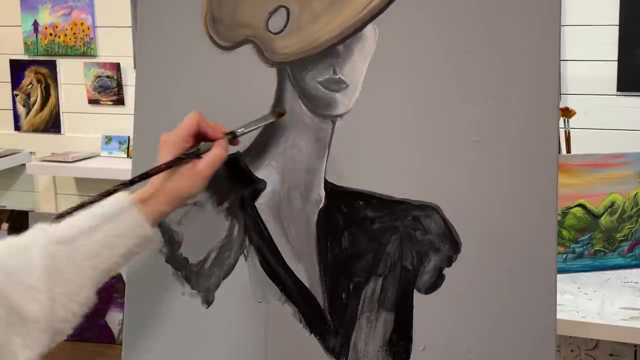 dries too much. It's important to make your brush strokes go kind of scooped like that sometimes, When you're painting something that's, you know, roundish like the neck, Put that light area in here, Then under the chin. 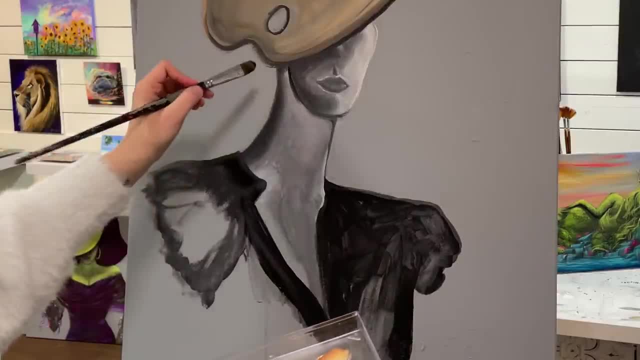 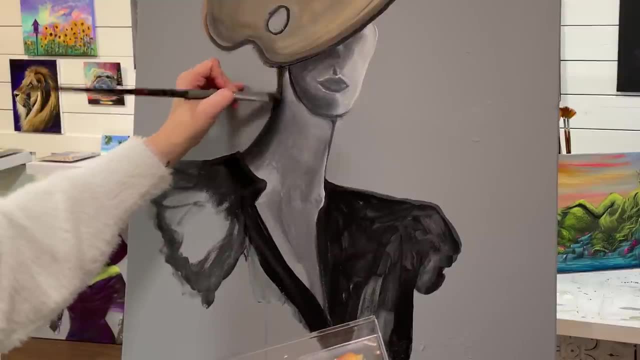 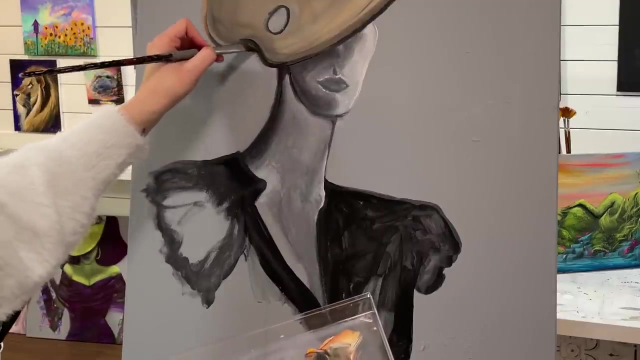 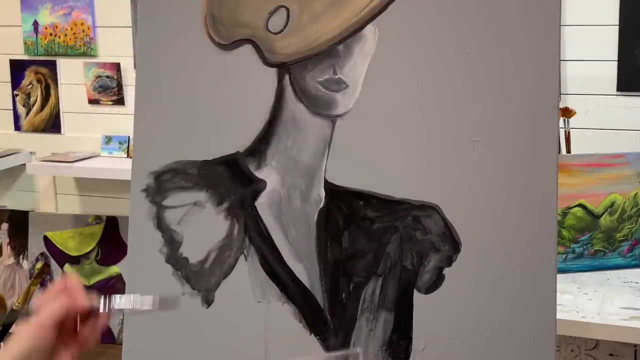 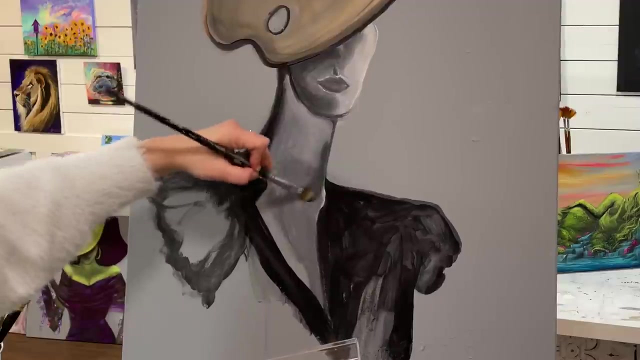 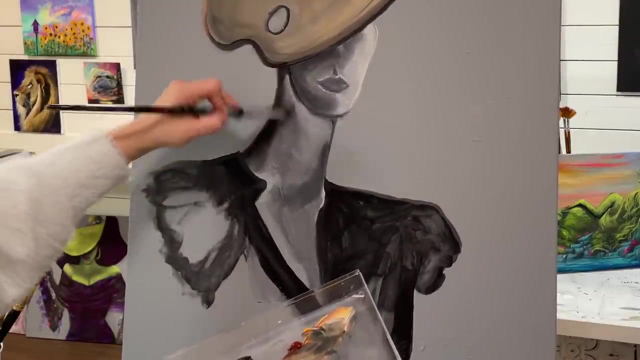 So some more shadow starts over here on the right. So take a little bit of white from her hand holding that paintbrush. Take a little bit of white So it helps me blend when I pick up more white in a way that it's not going to be too watery. 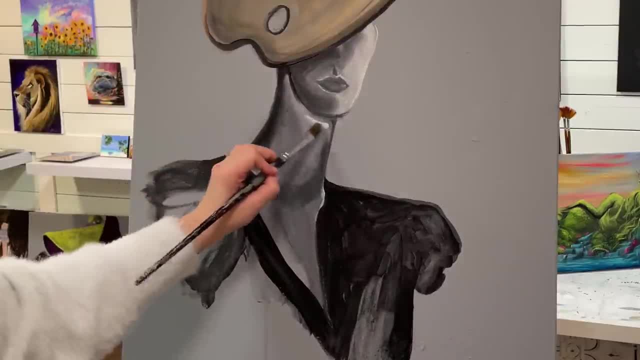 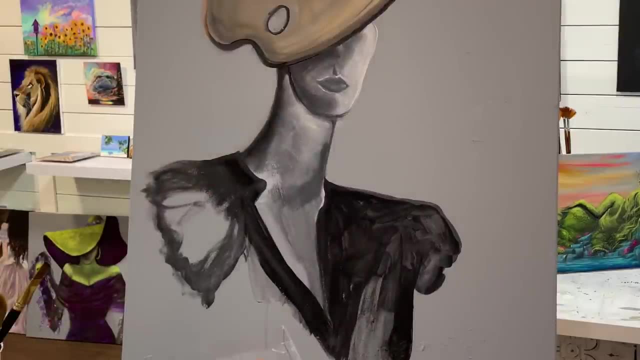 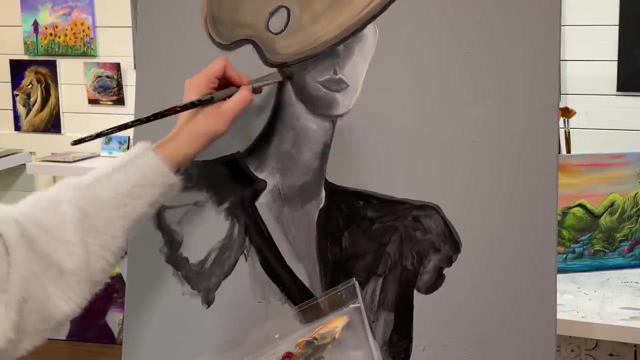 If I was to add a little bit of water to my brush, it might be a bit too watery, But it doesn't matter. I'm just going to take my brush and I'm just going to take a little bit of water. I'll bring it up to the neck and I'm going to do a little more water. 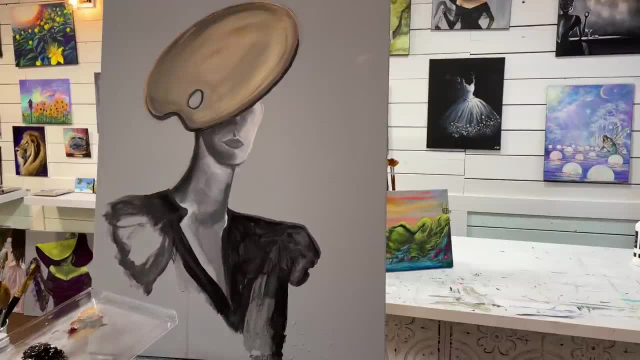 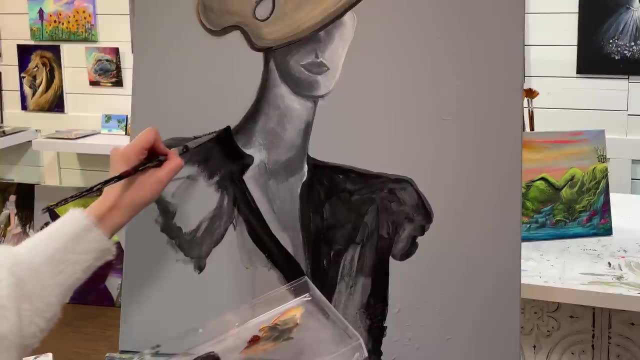 I'm just going to come back up here And then I'm going to go back and outfit there And I'm going to go back to the neck again and hit it a little bit higher. So I think this is my first time that I'm going to go back to the neck. 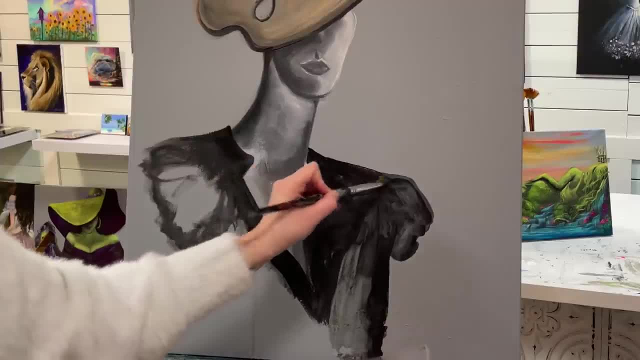 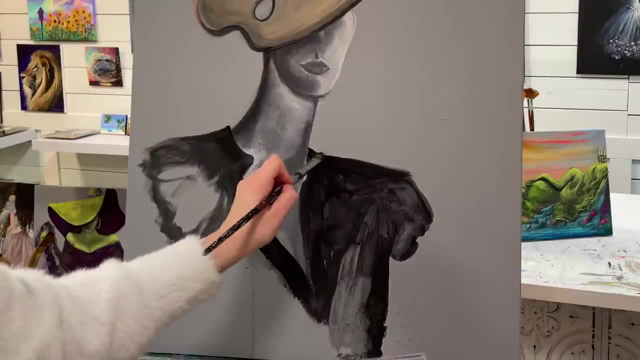 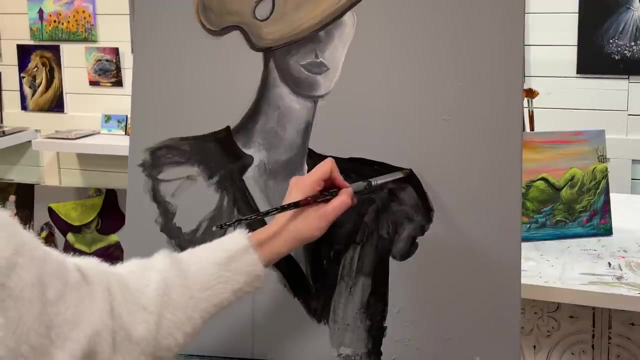 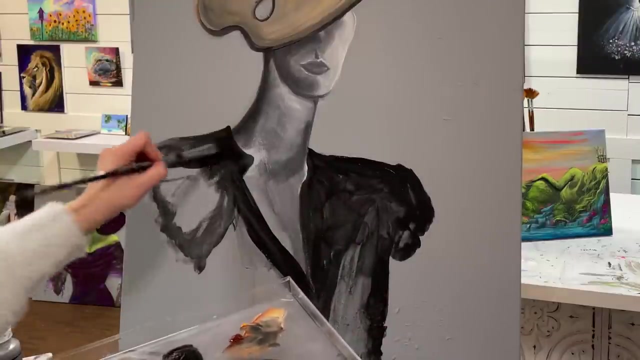 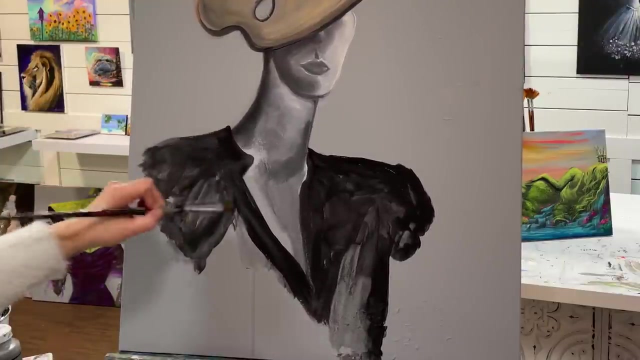 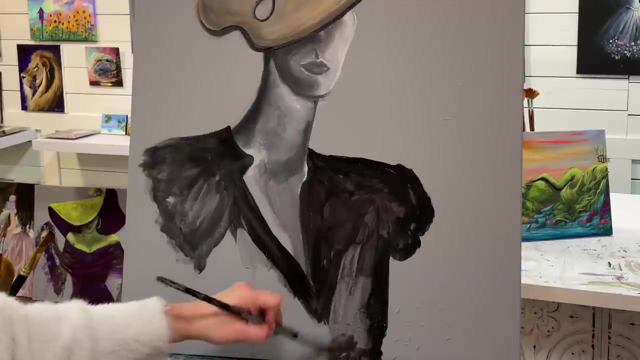 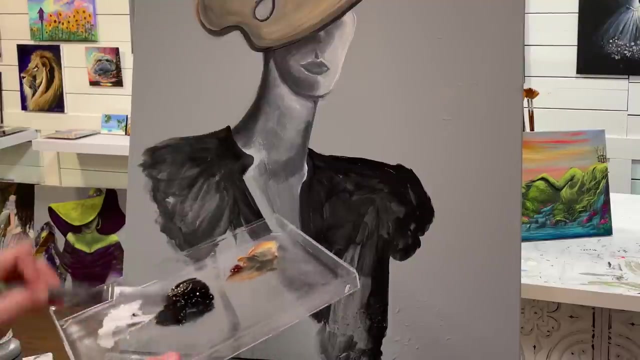 Which is going to bring the color of her shirt up And her shoulder area here a little bit higher. you square it out a little bit more here and then right in here. we're going to go around like this and then pull it in water and black. 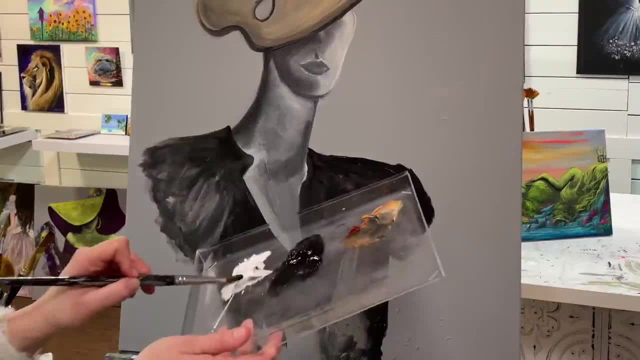 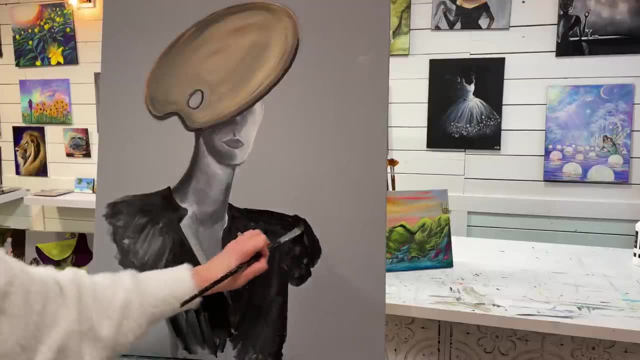 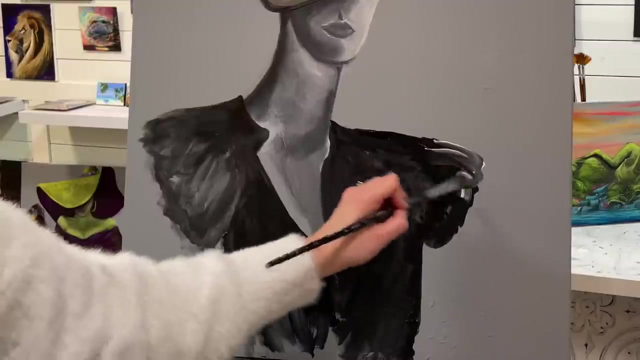 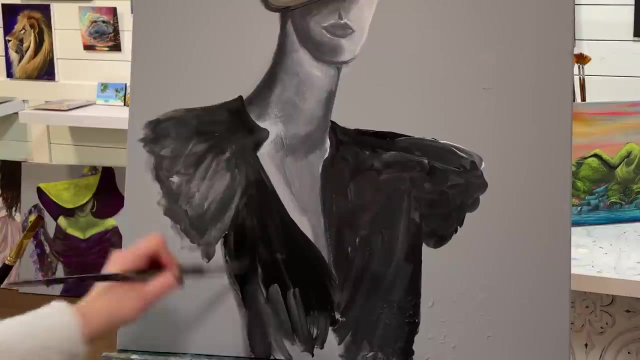 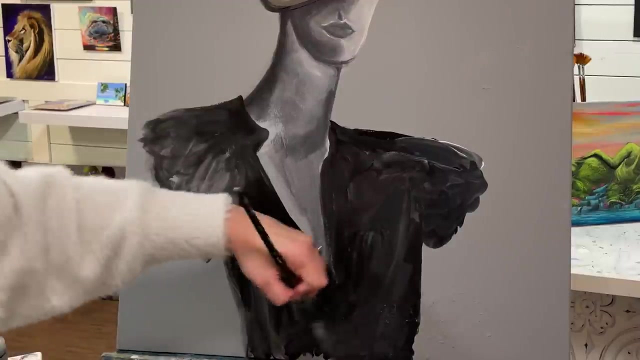 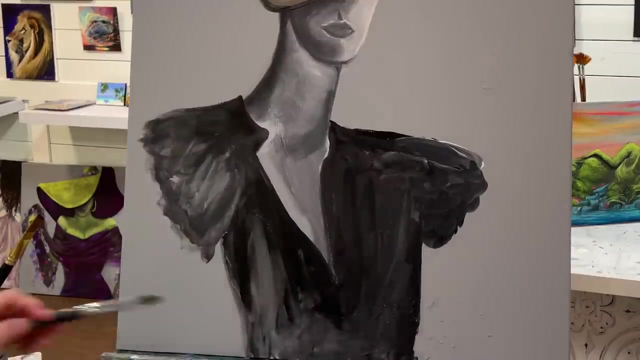 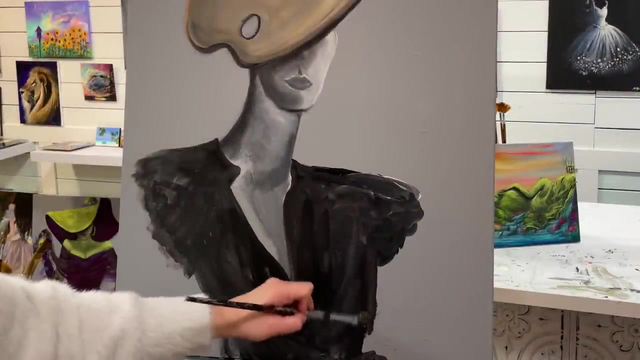 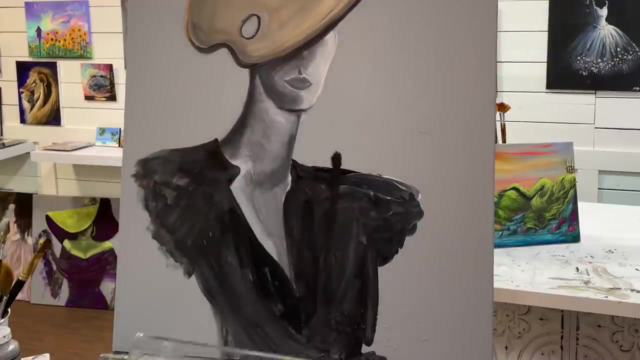 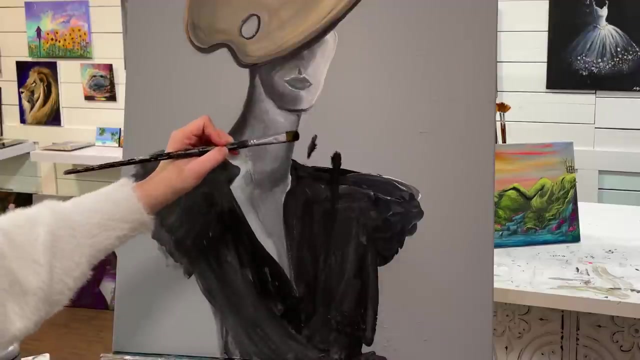 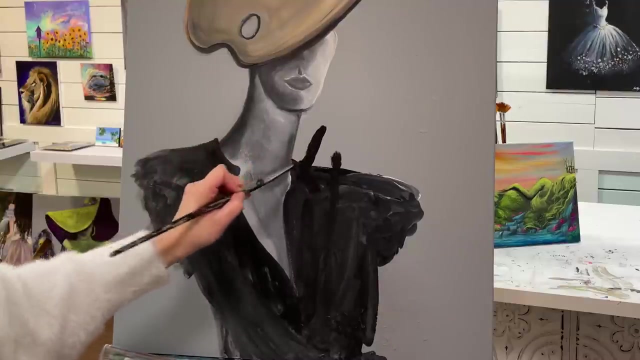 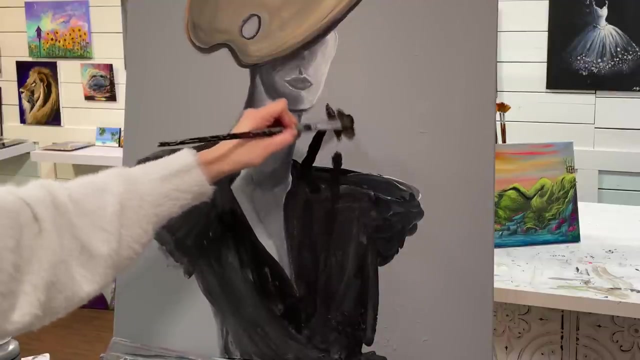 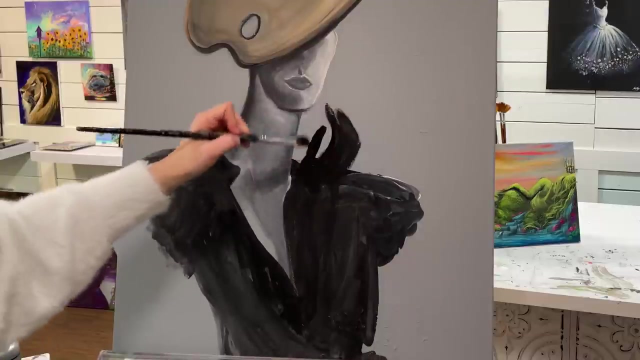 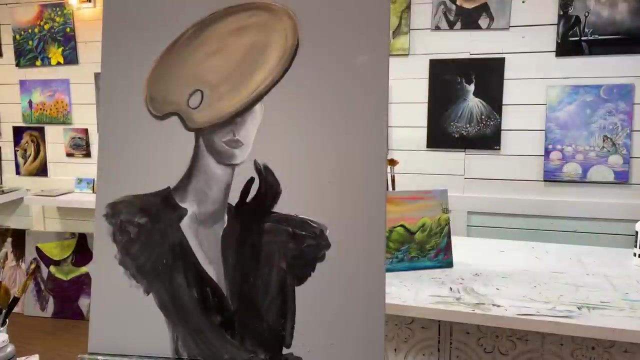 a little bit of white, bit more water. and then her elbow comes out, comes over here up indo, here here. a little bit of white, bit more water, and then pull it out a little bit more. We have a thumb And then her gloved hand. I'll just take a little bit of white. 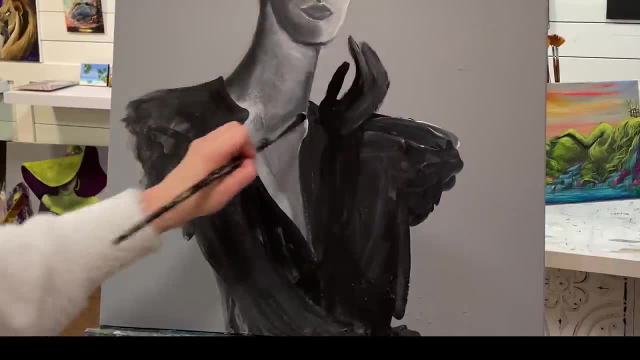 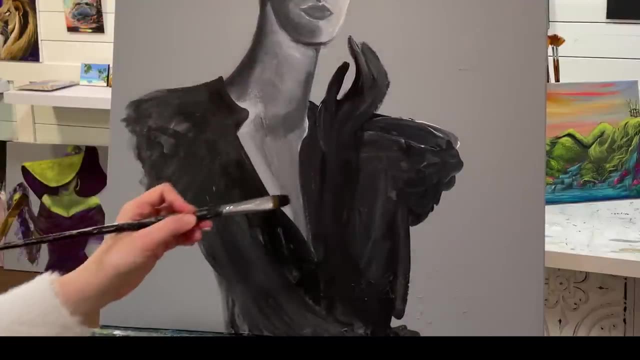 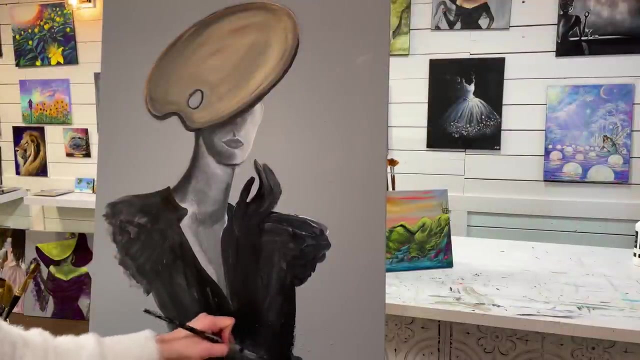 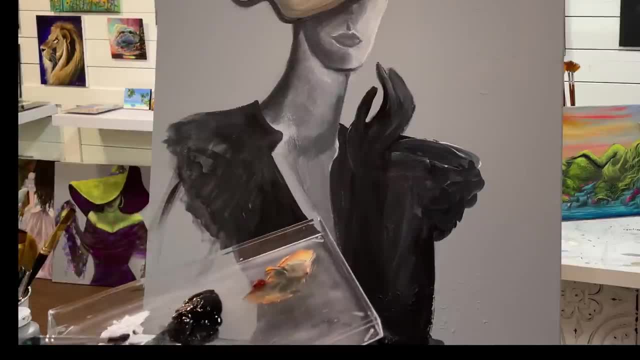 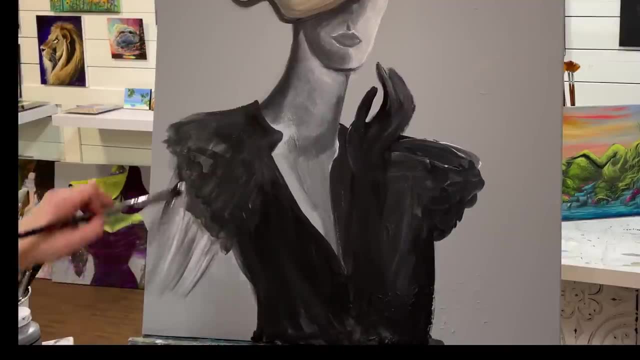 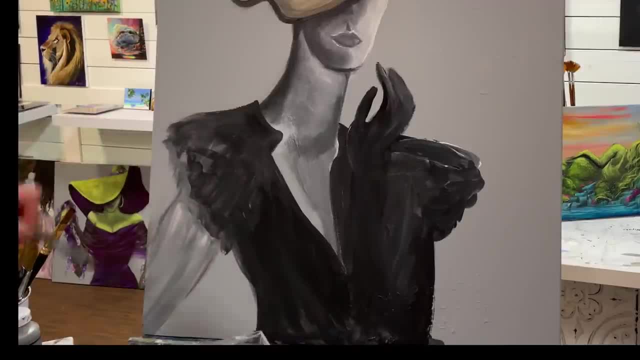 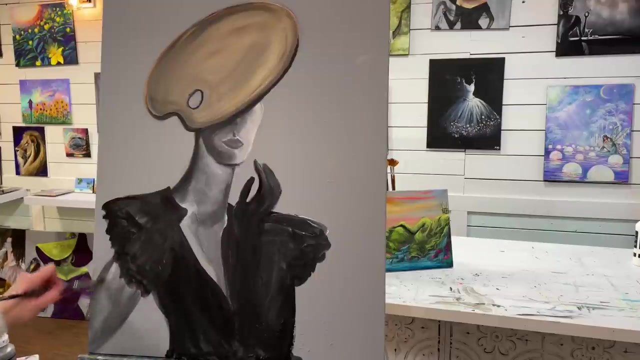 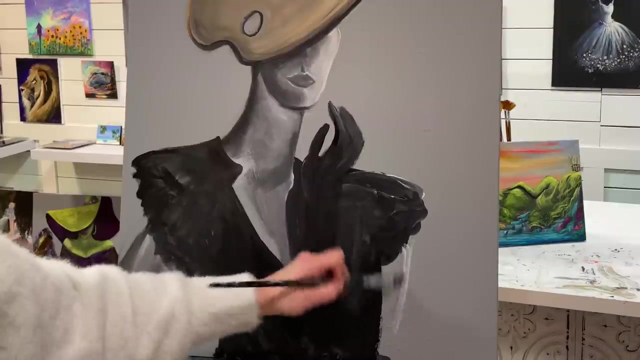 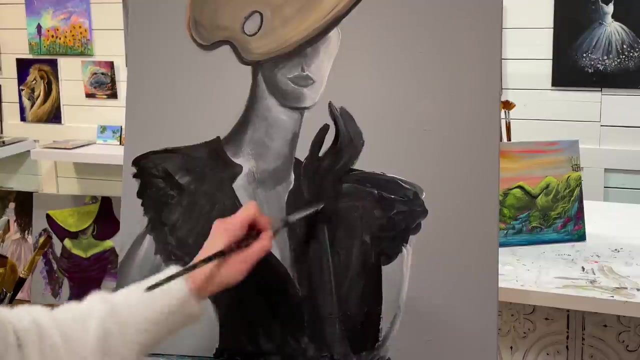 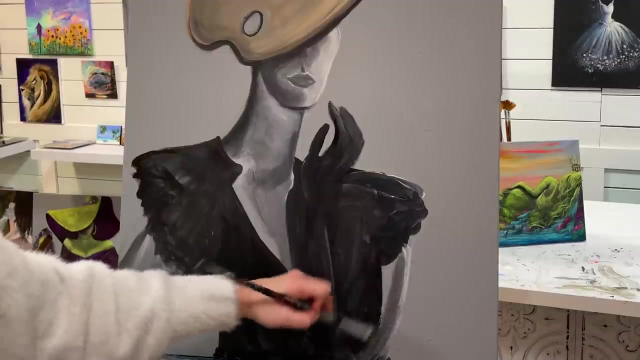 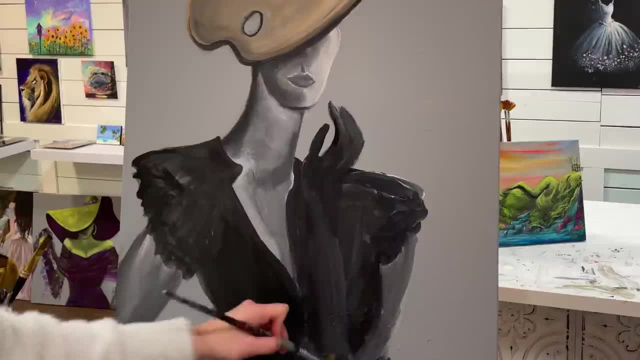 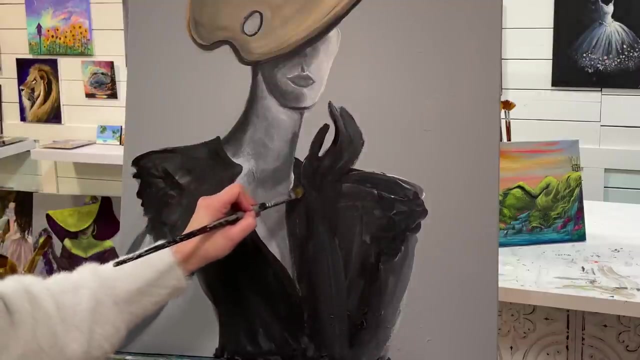 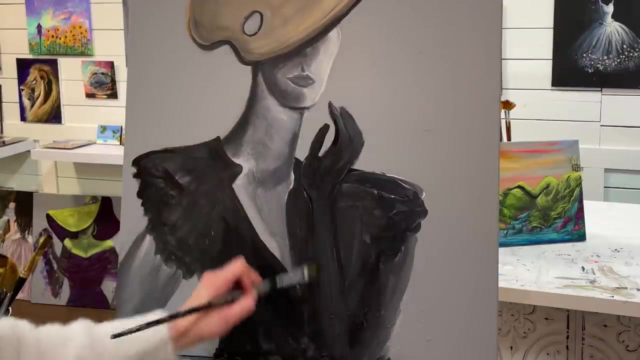 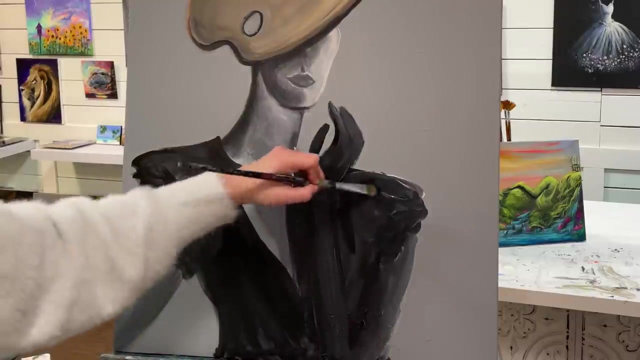 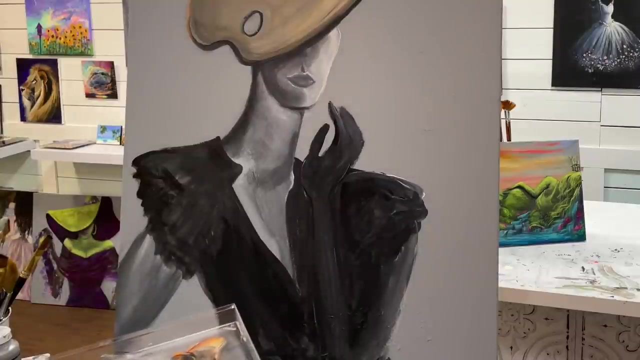 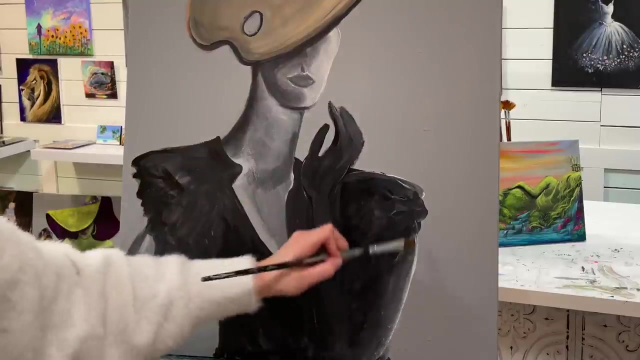 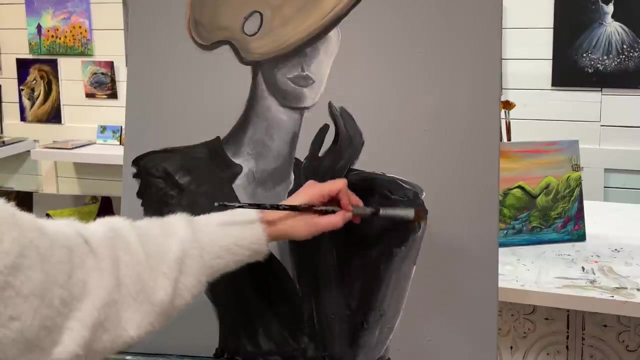 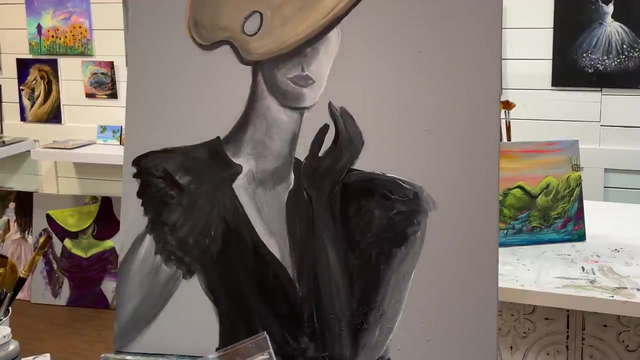 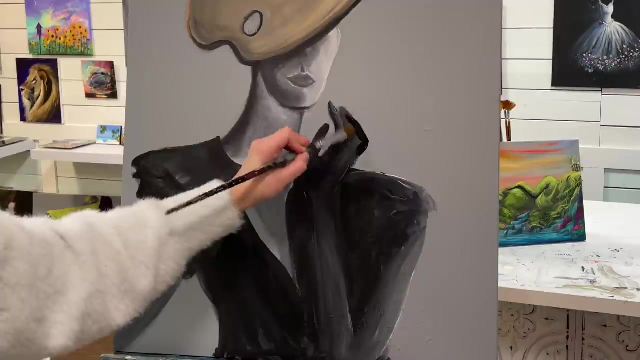 elbow you. even though the proportions are not perfect on this, there's still something so artsy about this that I'm liking. so you really don't have to be perfect with your proportions to like your painting. you can add your own. bring your hand out a little bit more this side. 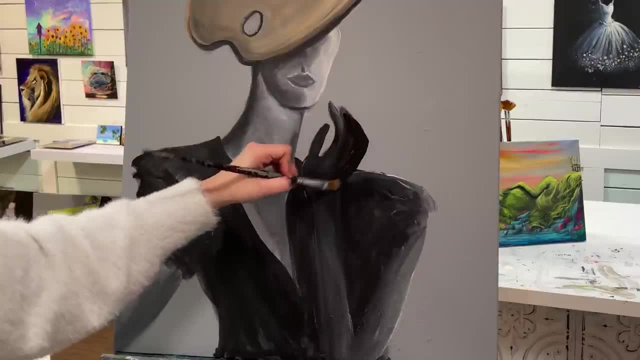 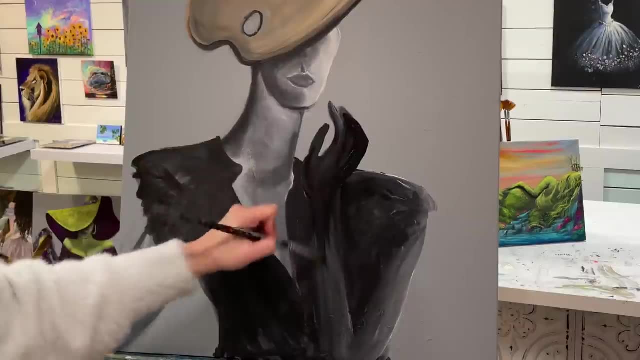 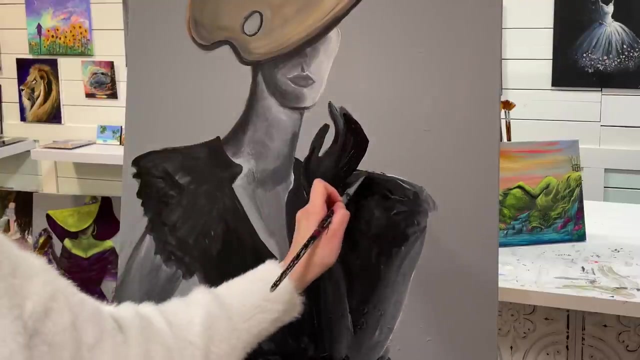 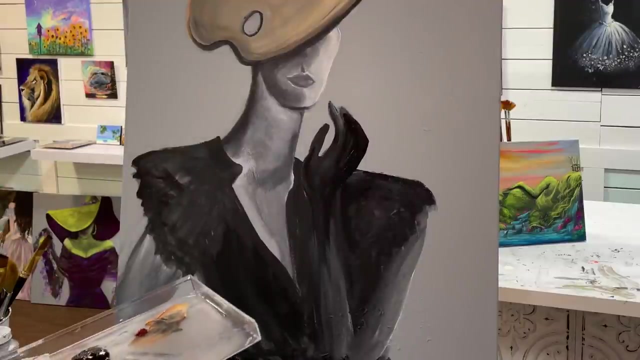 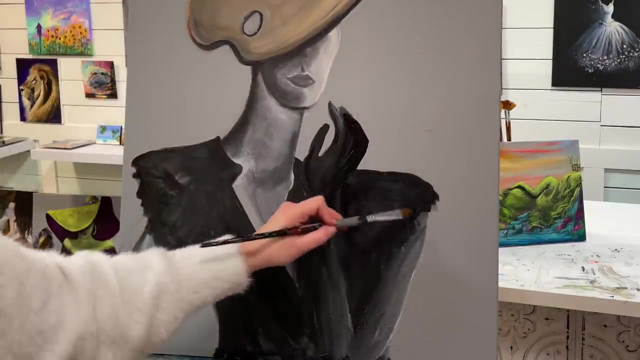 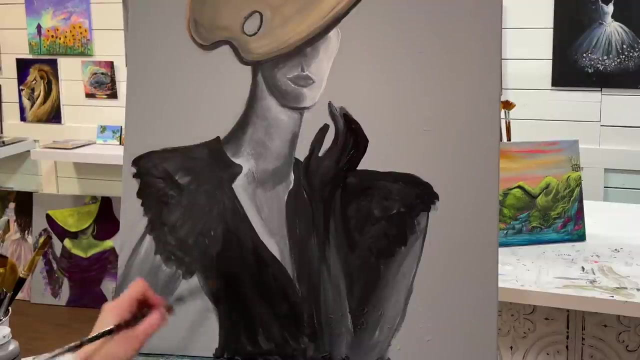 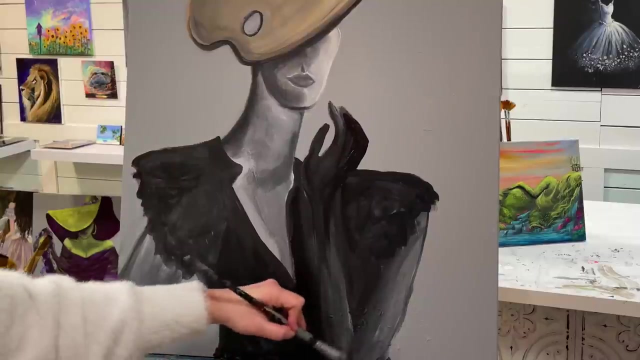 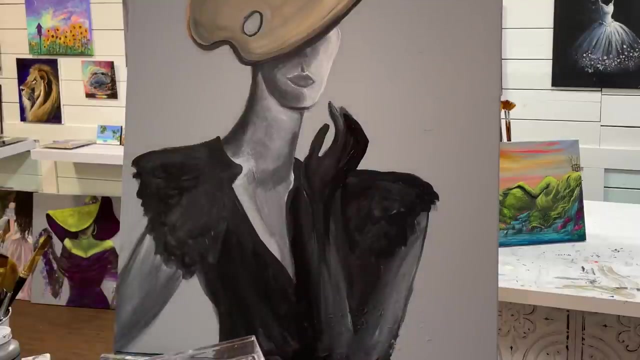 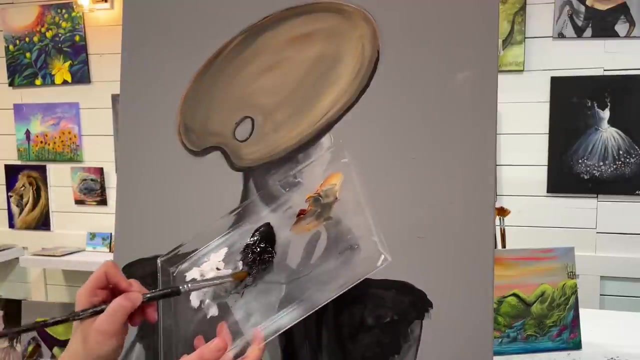 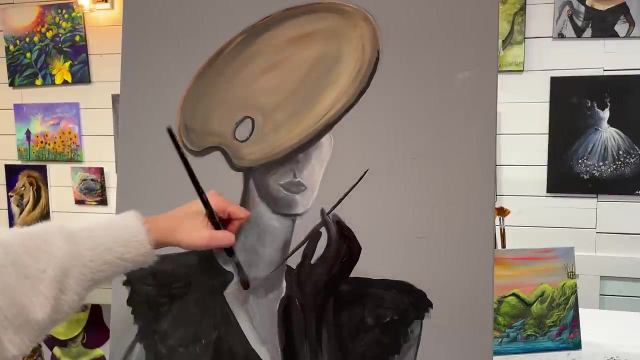 1 left 3 1 1 1 1 1 1. All right, And I'm going to add the paintbrush now, So I'm just going to take black and just loop through here. Just a simple line. 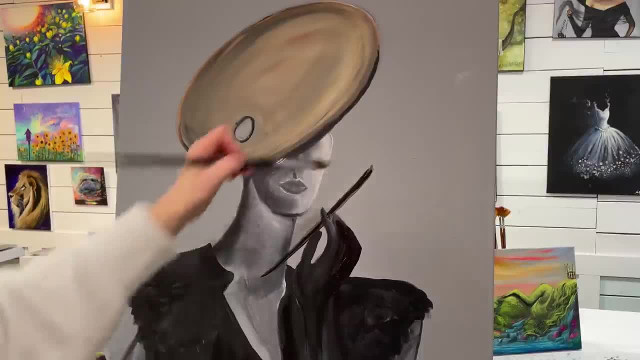 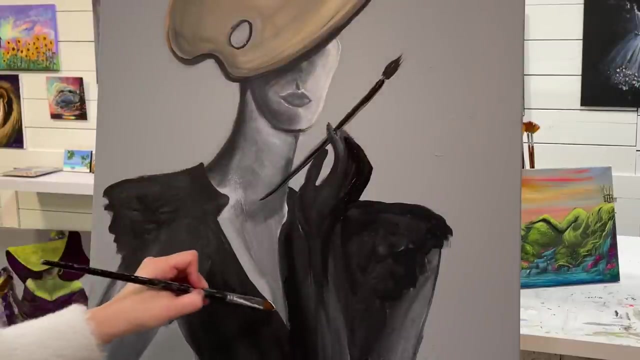 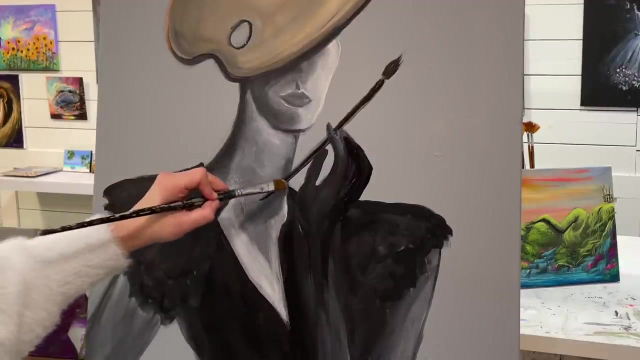 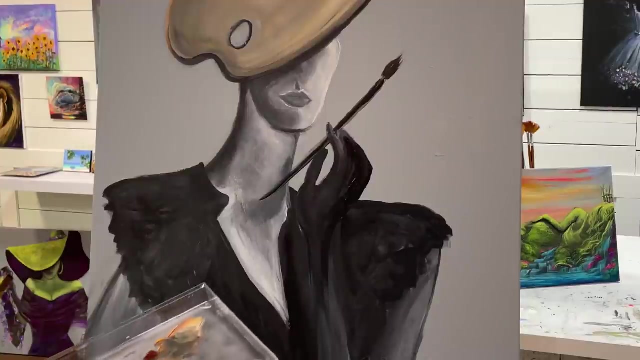 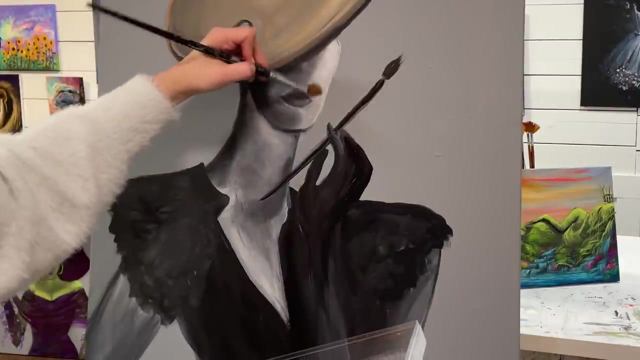 You can get a little bit narrower at the bottom And then a little flick. Okay, washing my brush out, I'm going to take some more white now And I'm going to come right down here And add some more highlights. So just the same places that I already have and want there to be some highlights, okay. 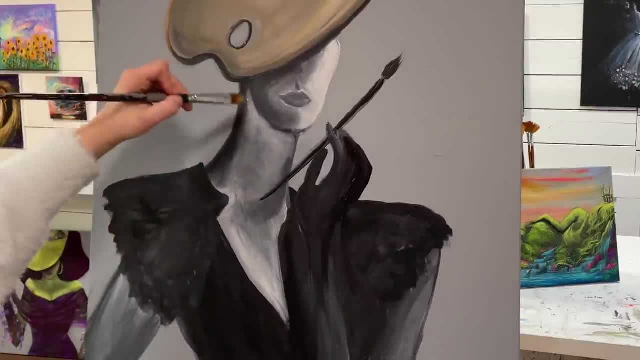 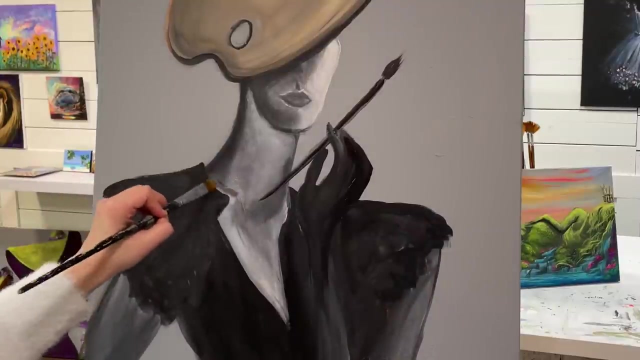 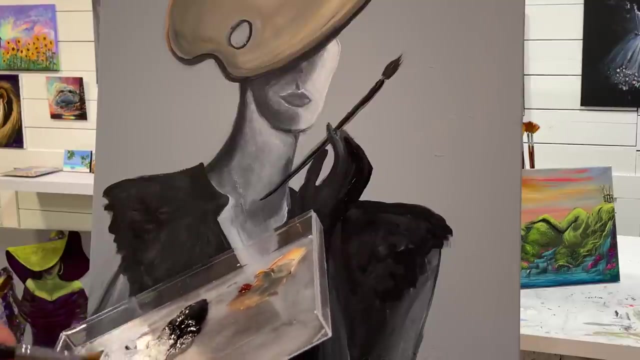 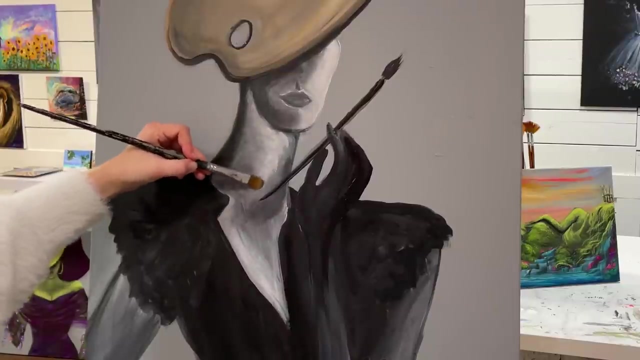 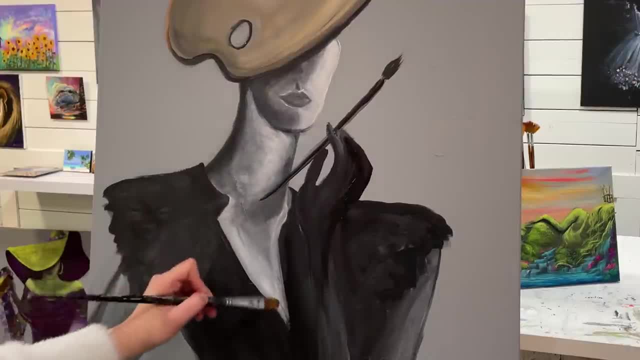 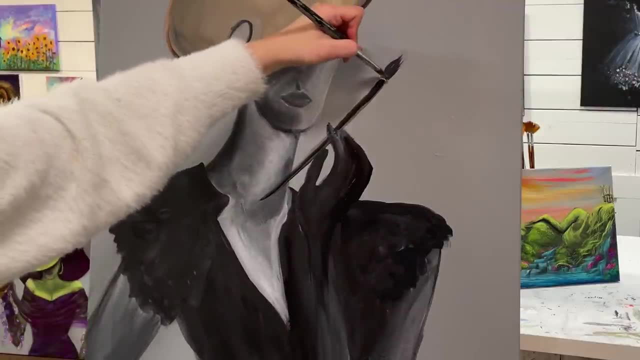 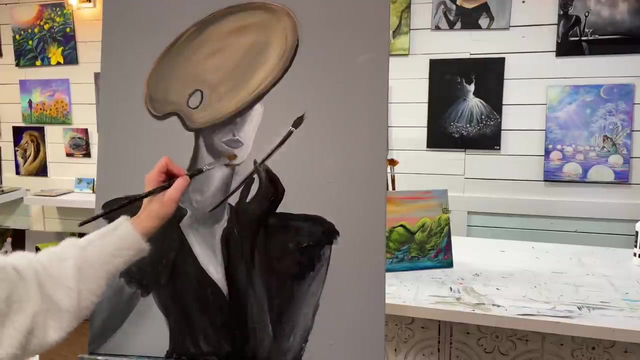 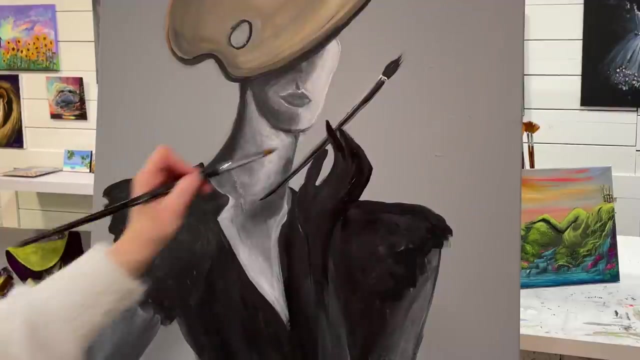 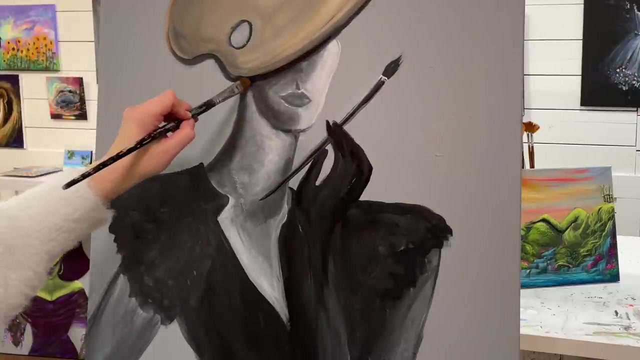 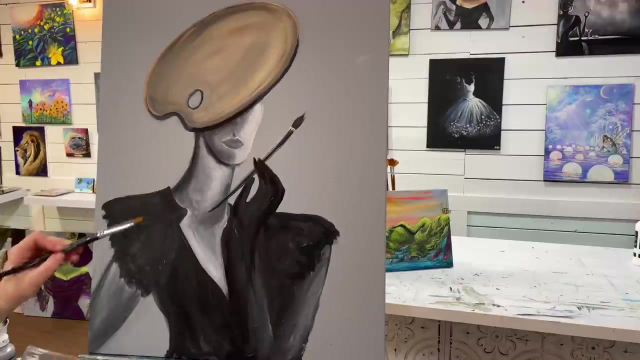 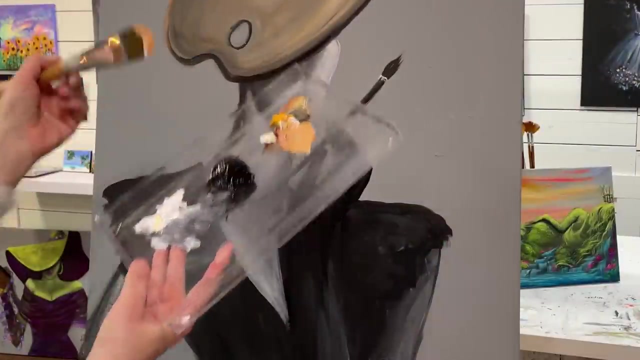 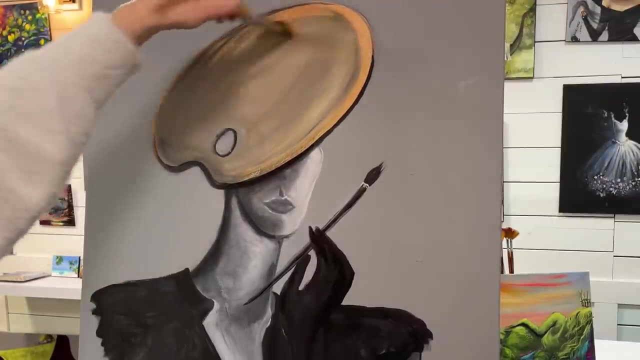 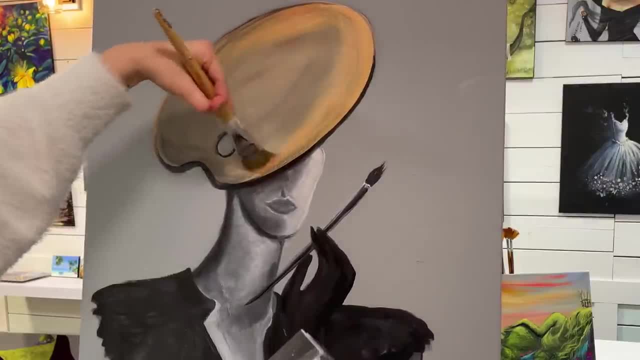 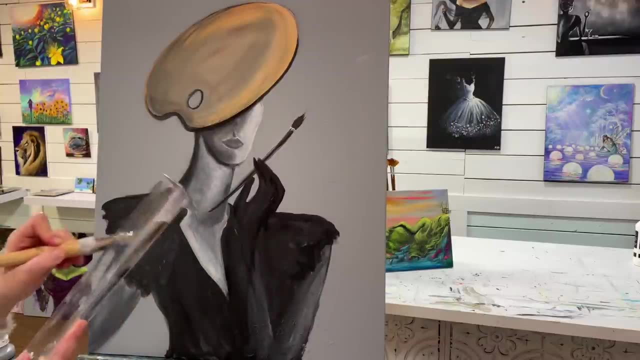 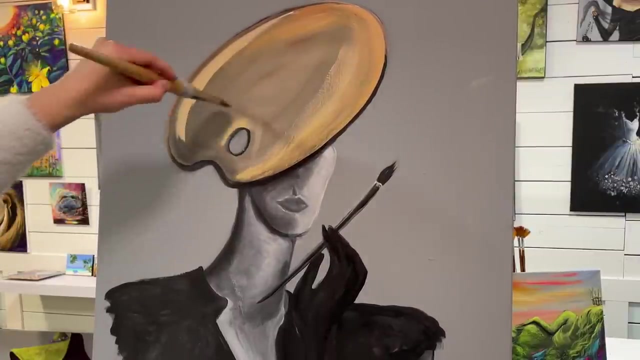 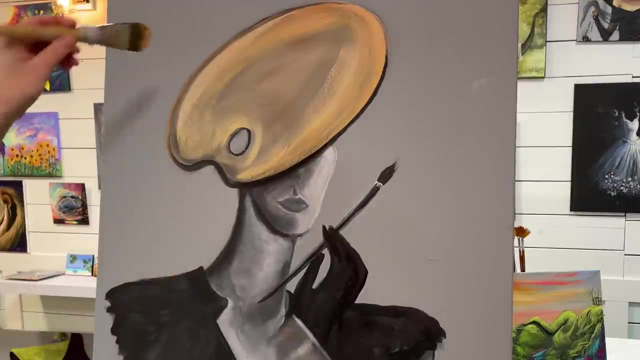 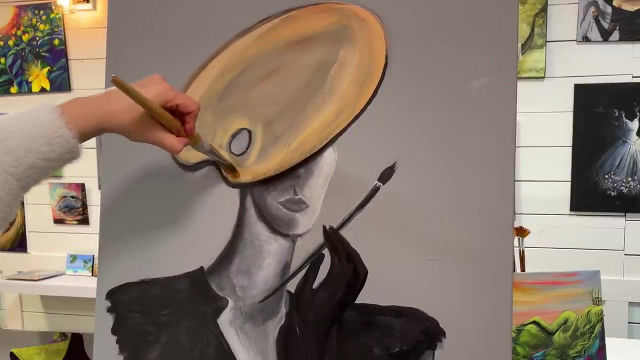 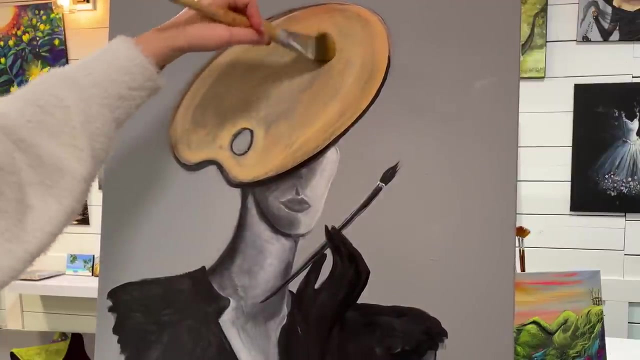 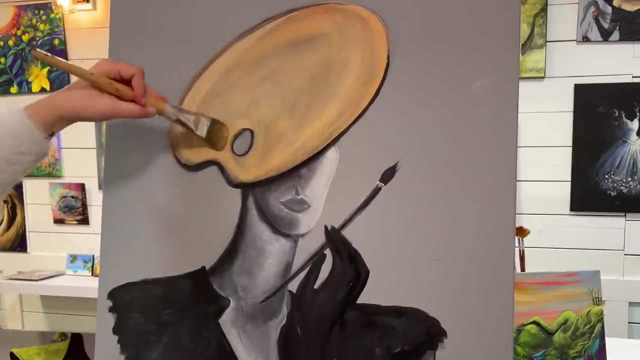 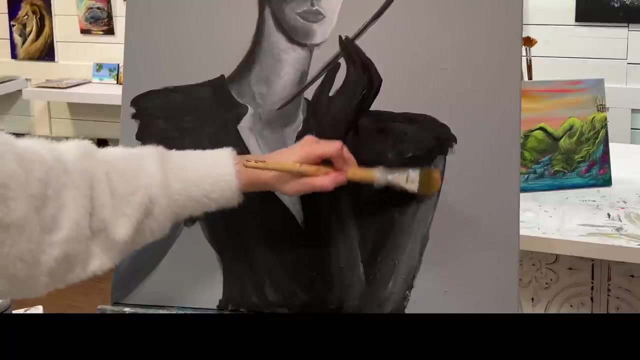 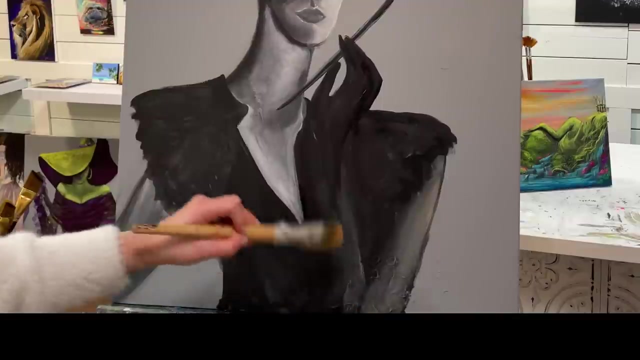 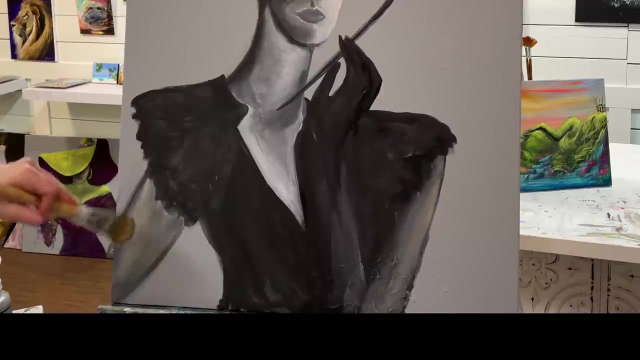 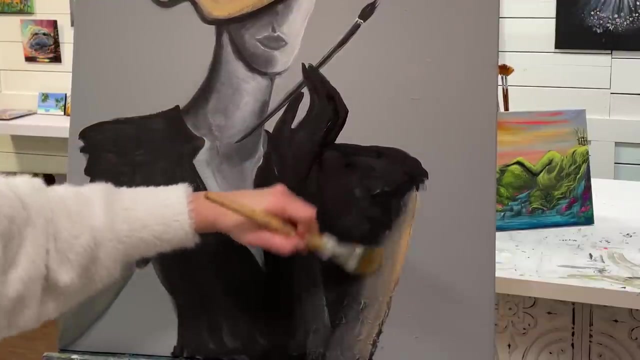 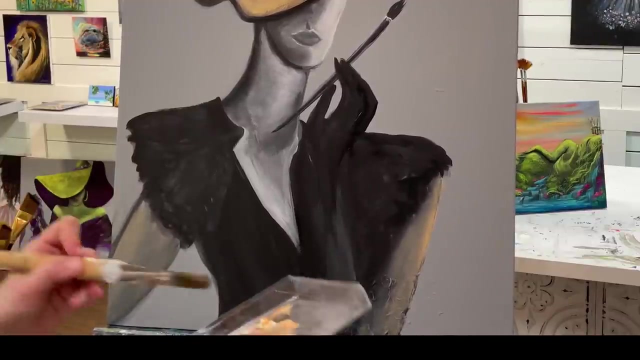 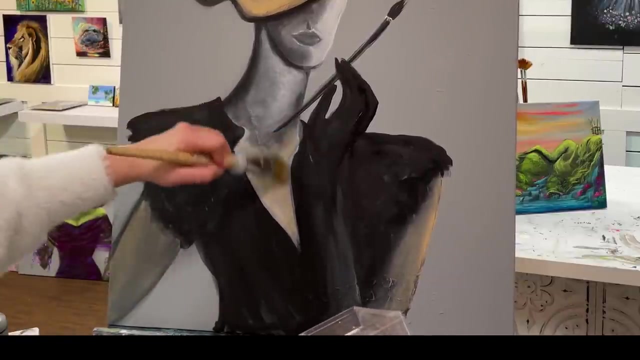 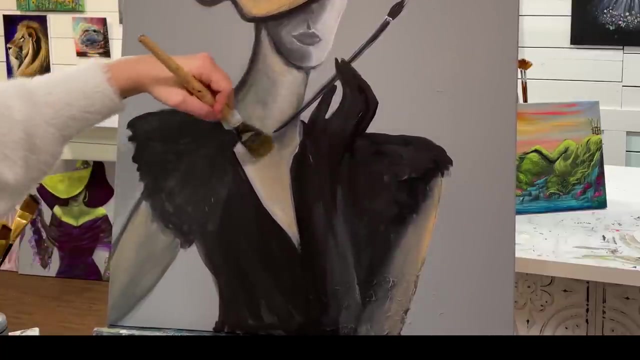 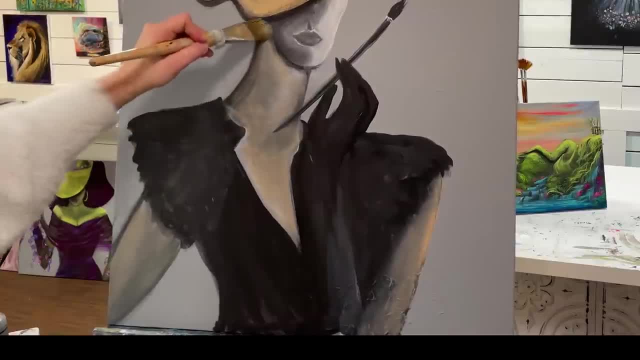 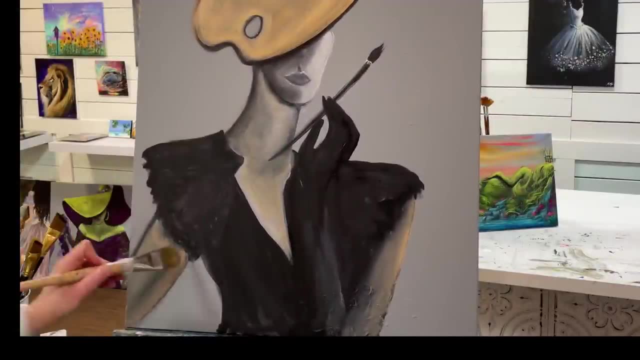 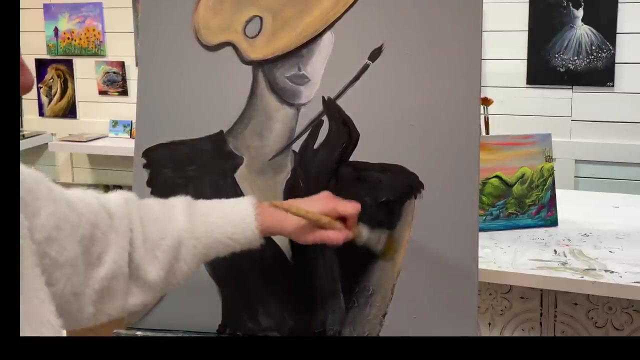 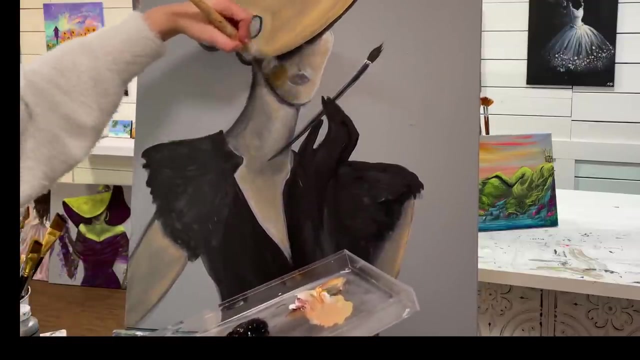 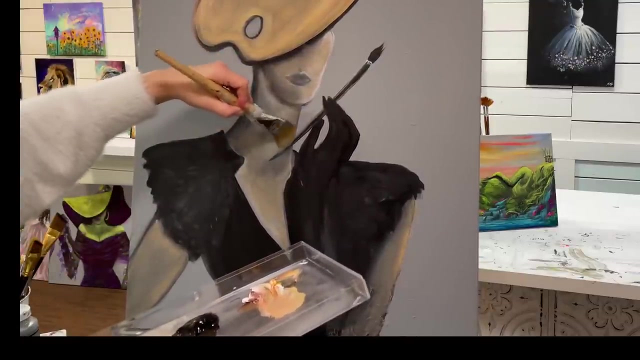 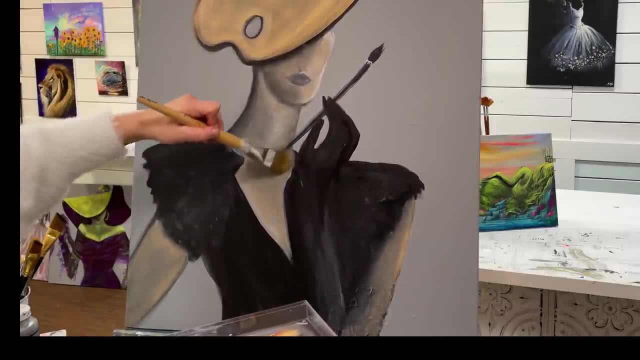 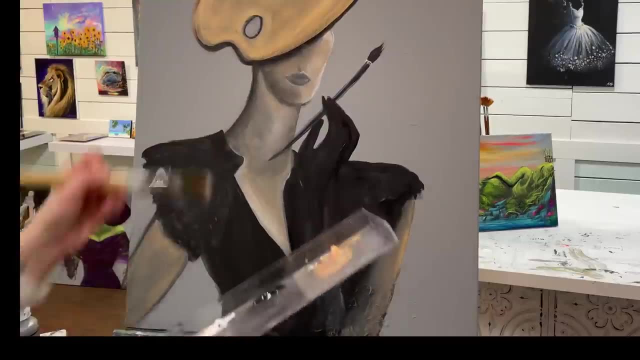 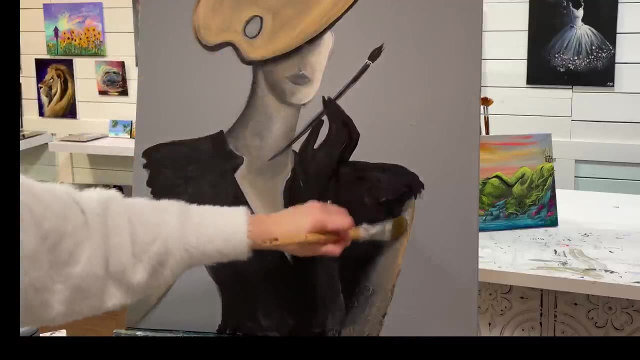 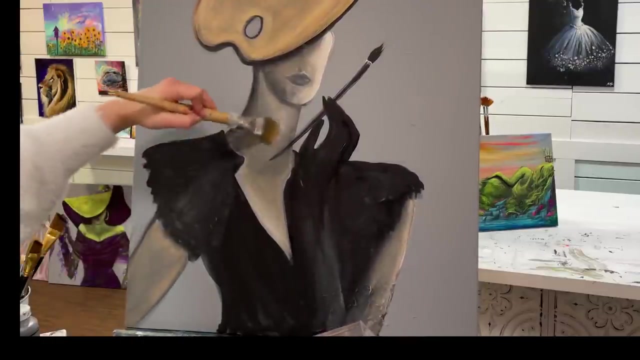 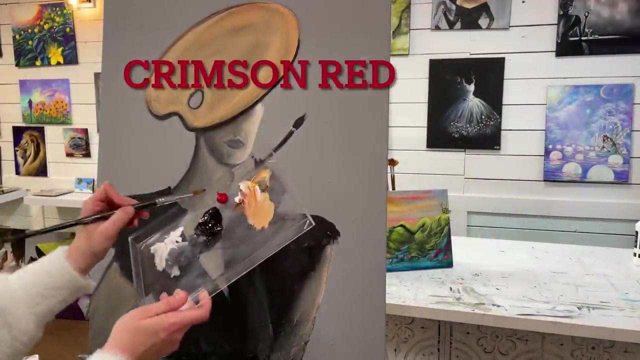 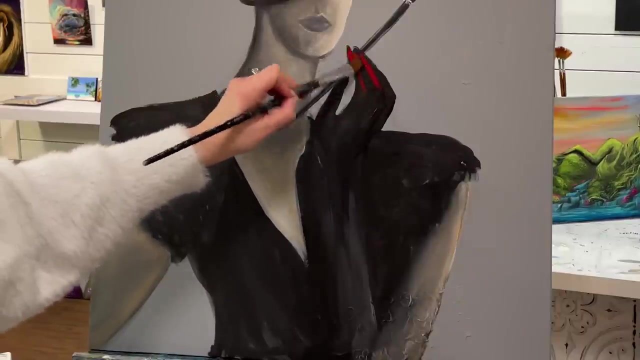 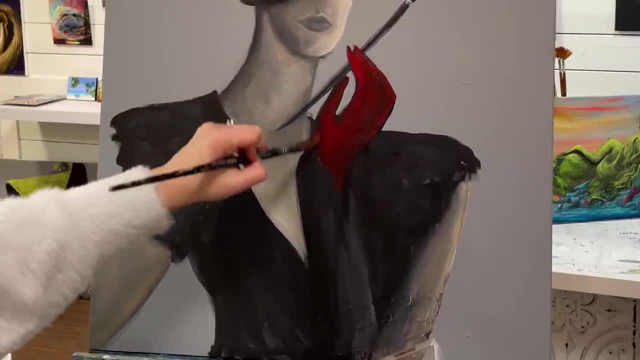 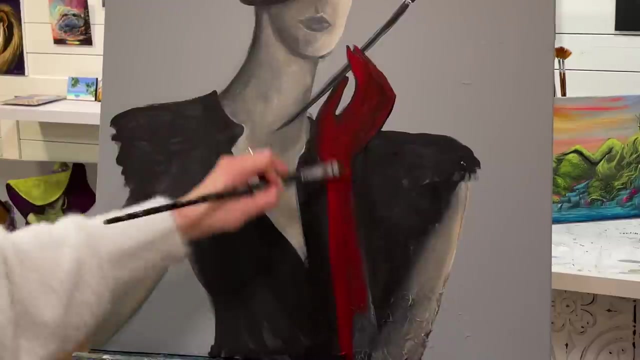 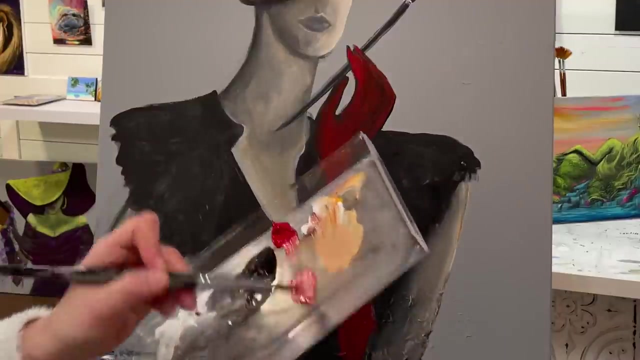 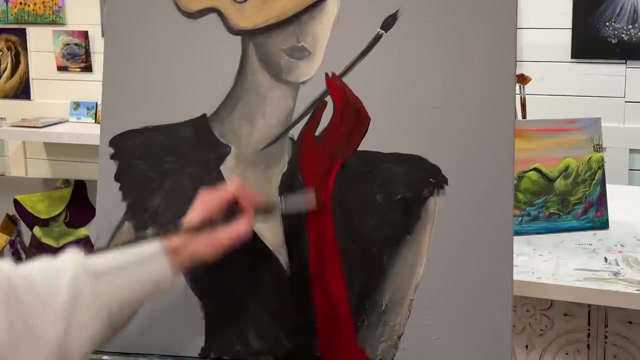 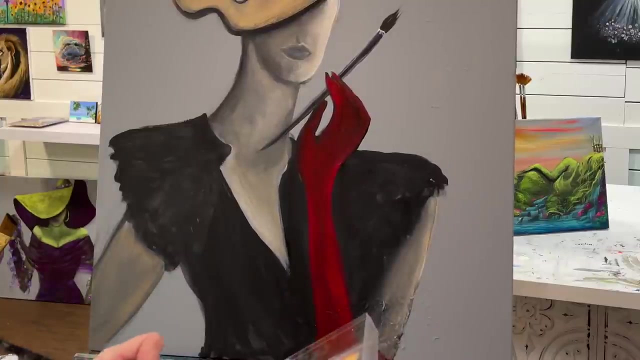 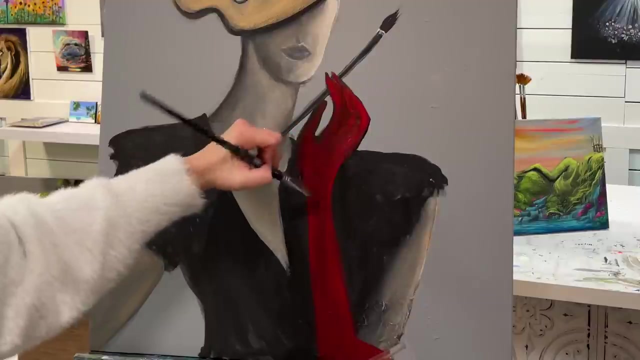 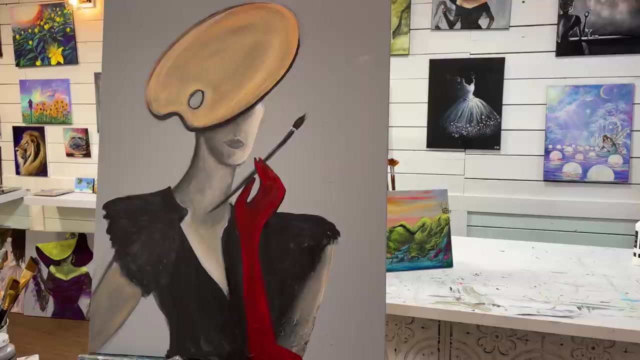 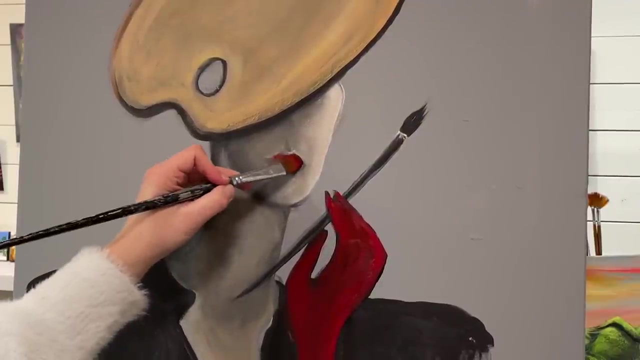 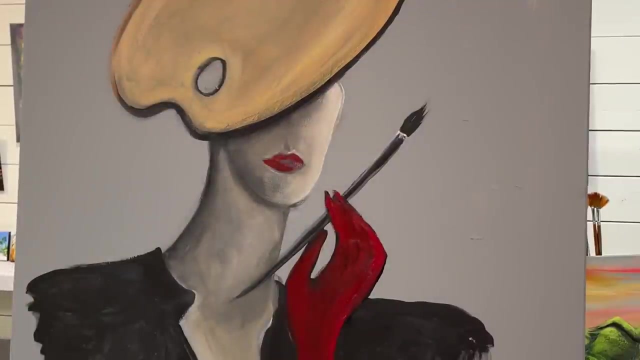 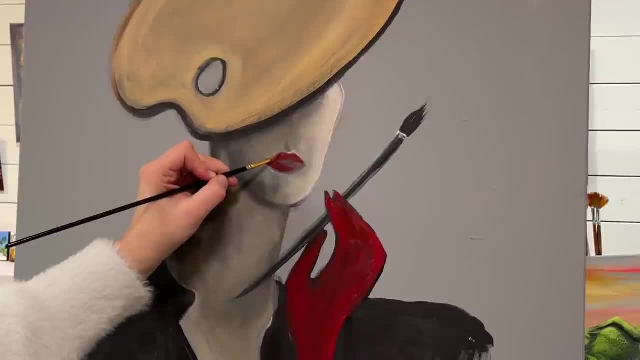 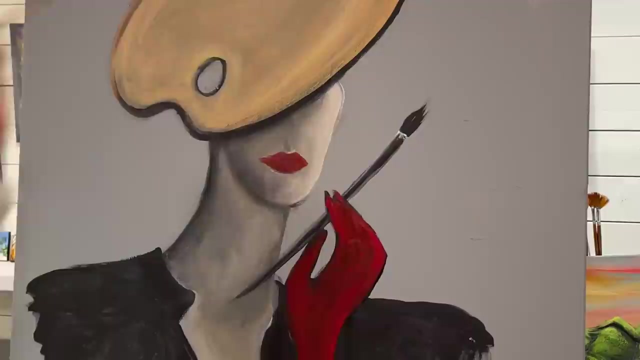 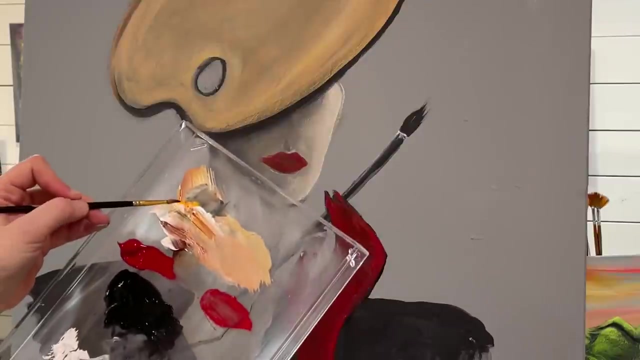 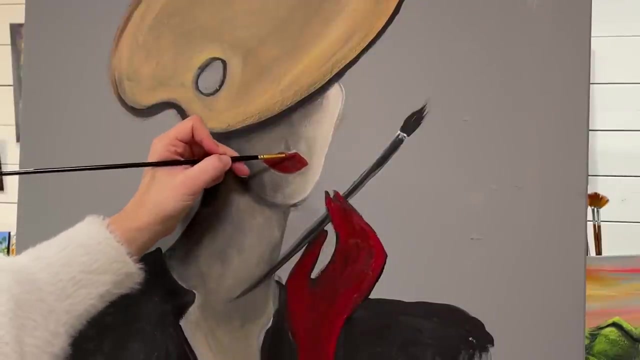 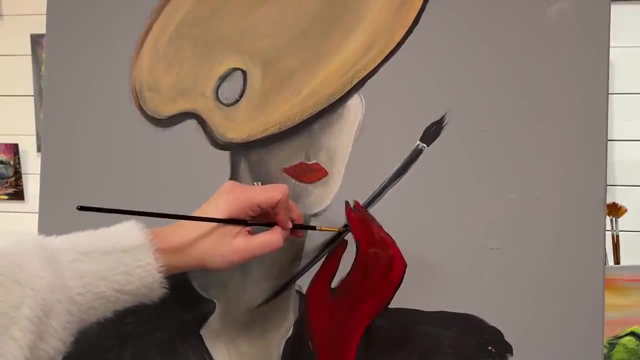 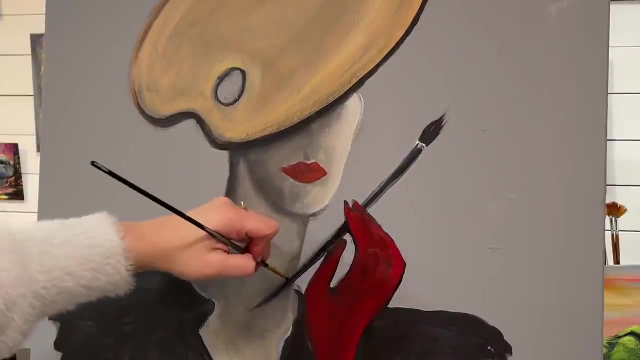 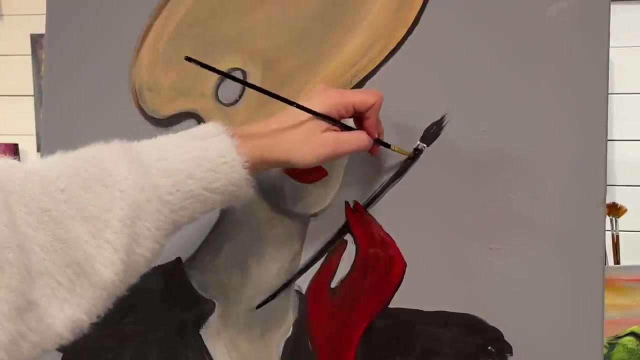 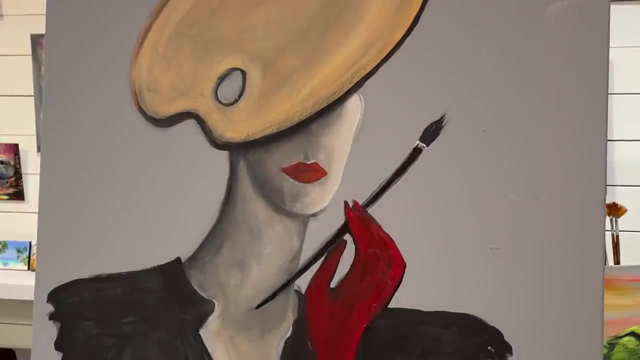 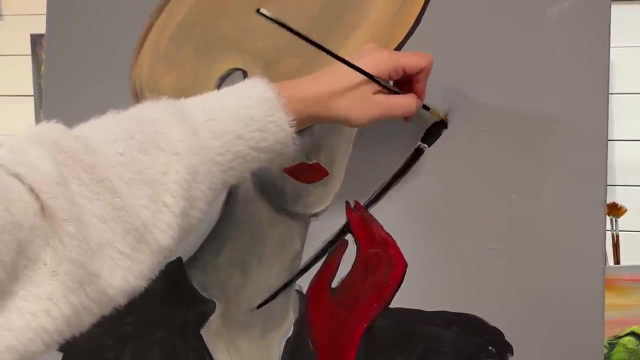 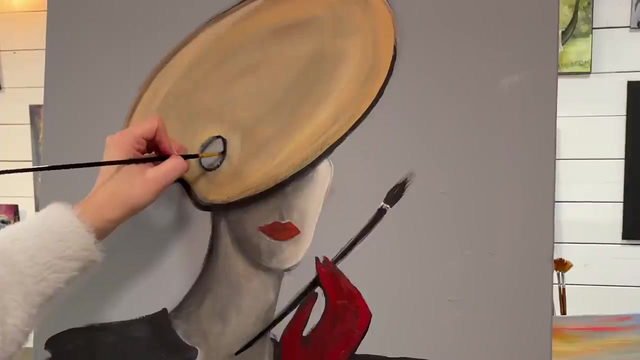 my number two round brush. I'm going to pick up a little bit of that yellow warm with my red and and and just slightly highlight this, just slightly highlight this, just slightly highlight this a little bit right there and and. All right, Okay, I'm just going to outline this little hole again. 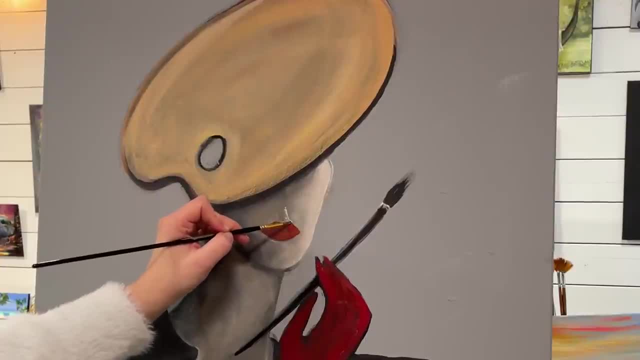 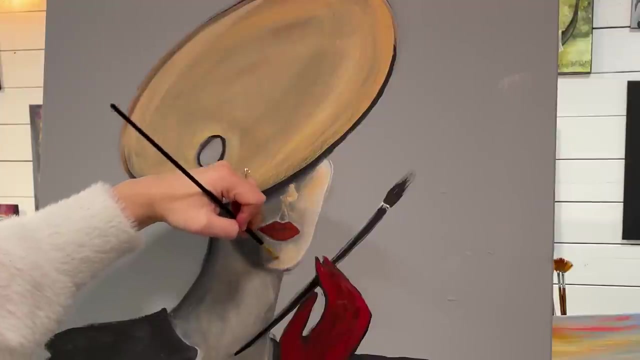 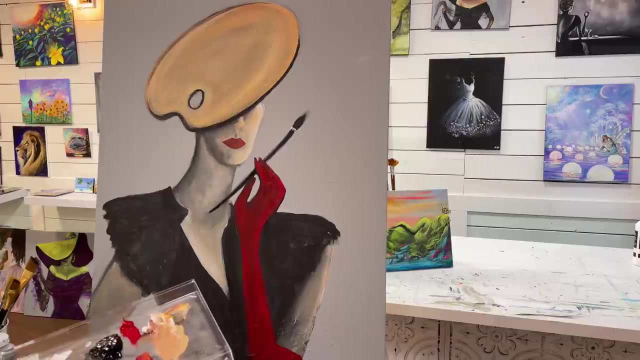 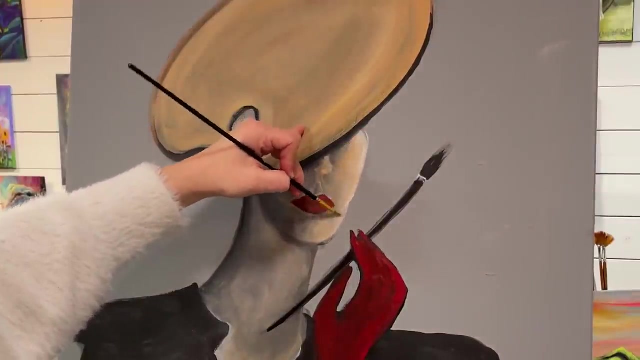 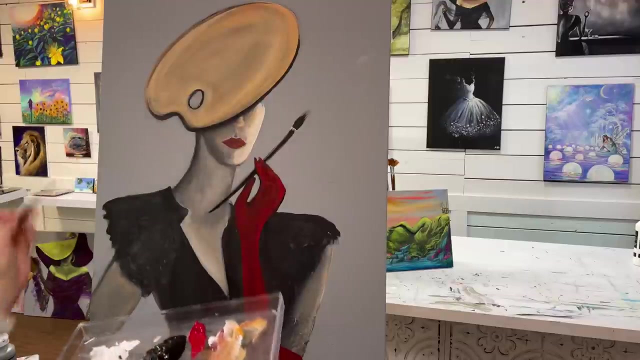 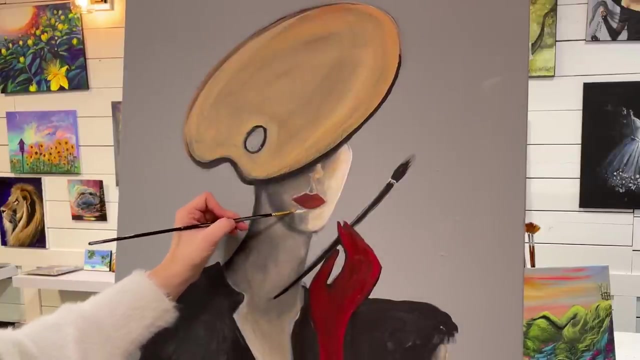 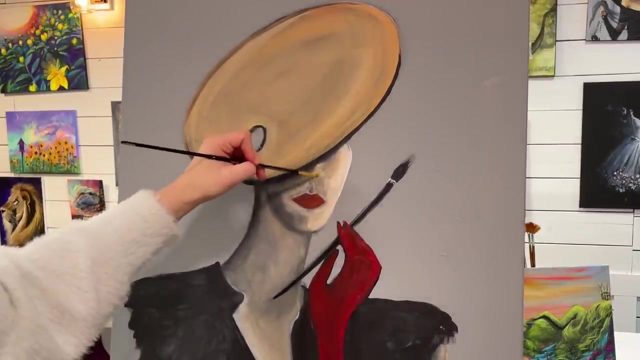 Another highlight right here around this little area around her mouth And then her nose. I'm just going to see a little bit of her nose. I'm going to slightly widen this, bring that out just a little bit. And then I'm just going to bring that out just a little bit. 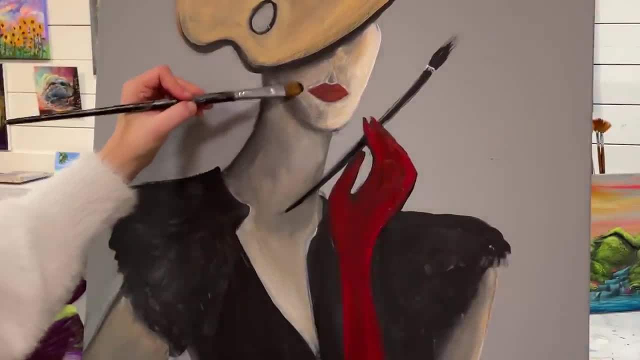 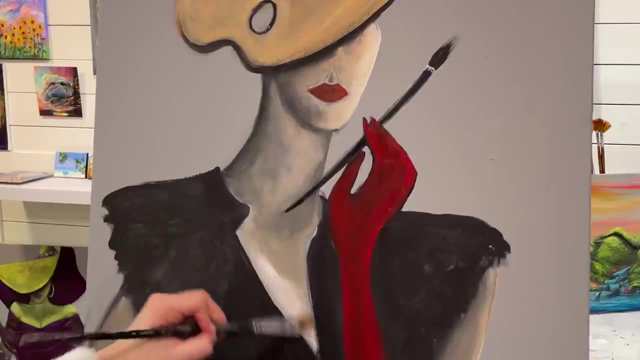 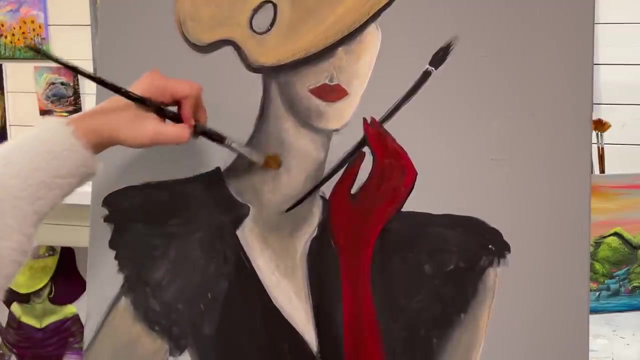 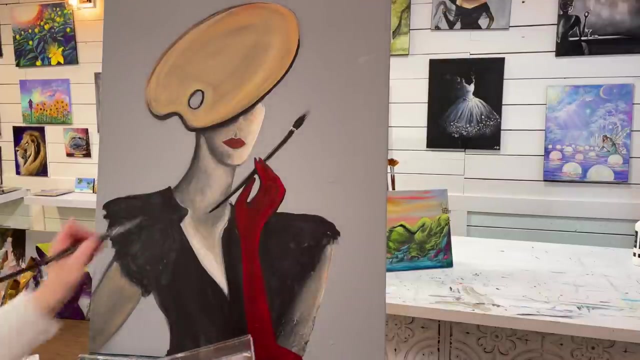 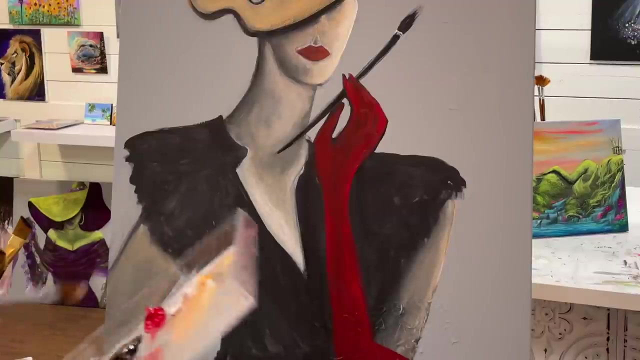 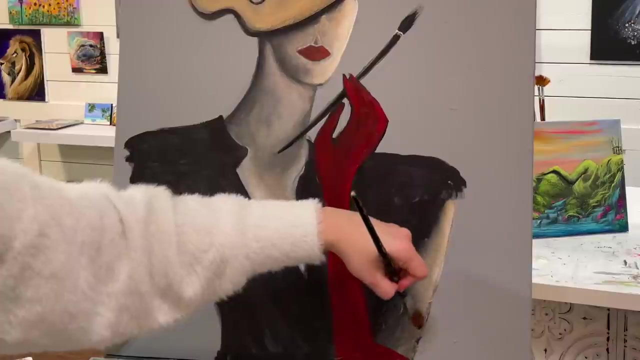 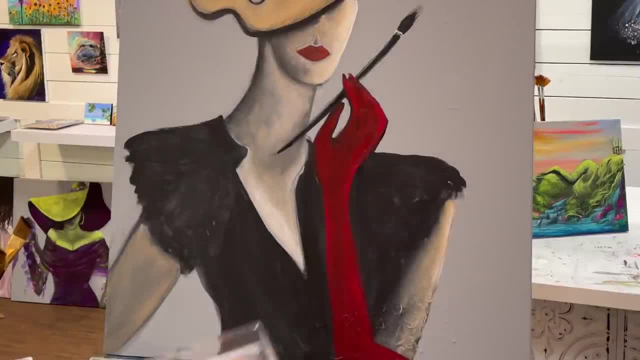 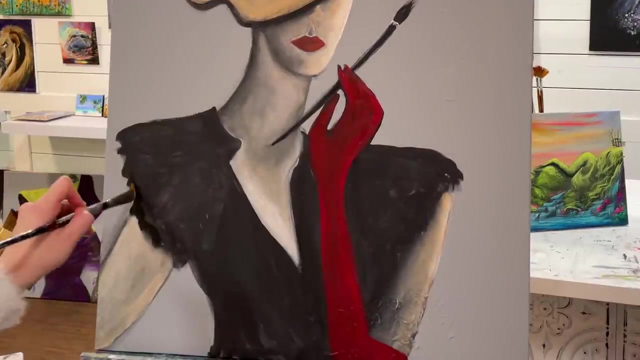 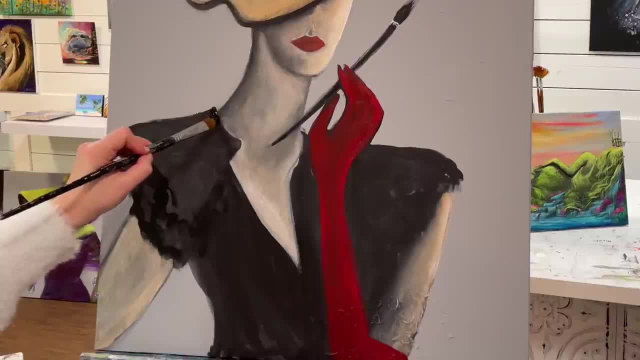 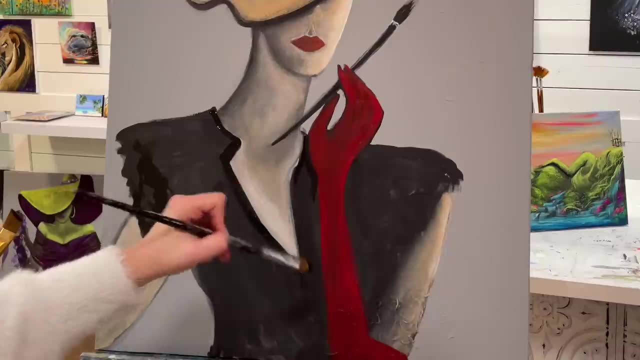 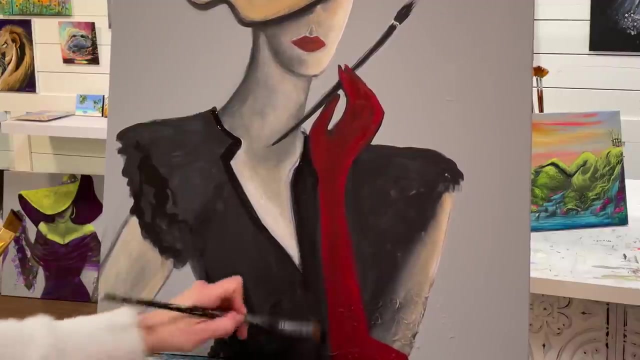 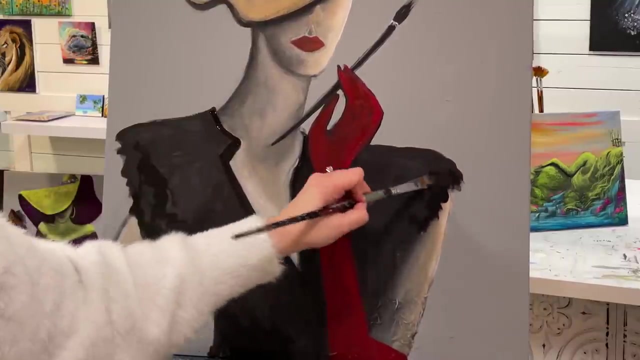 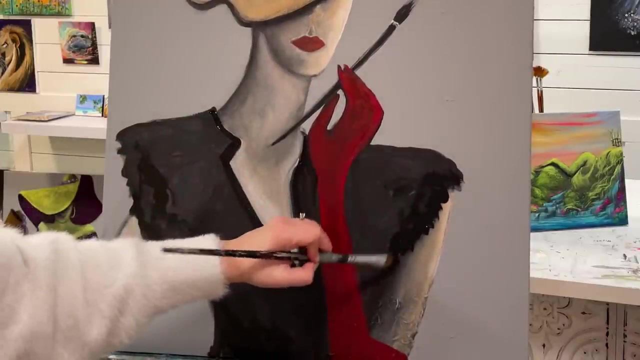 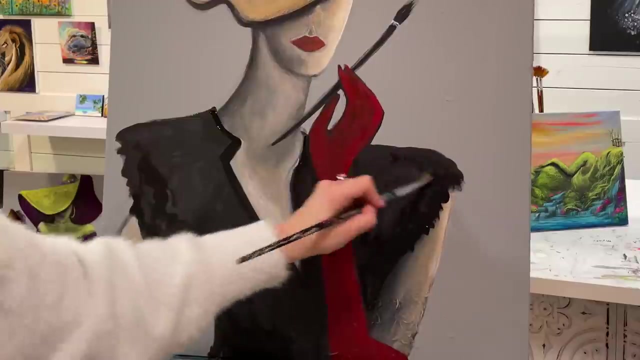 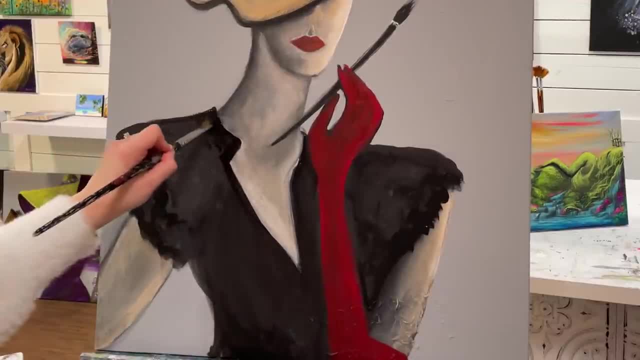 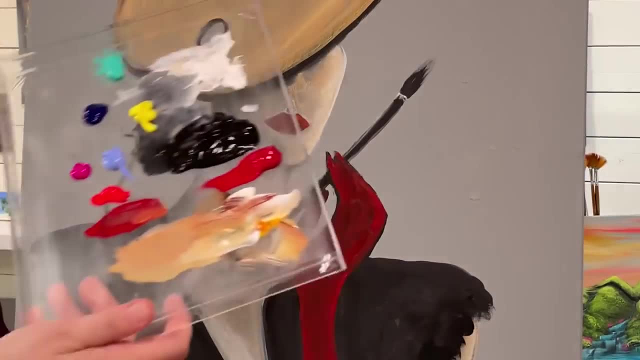 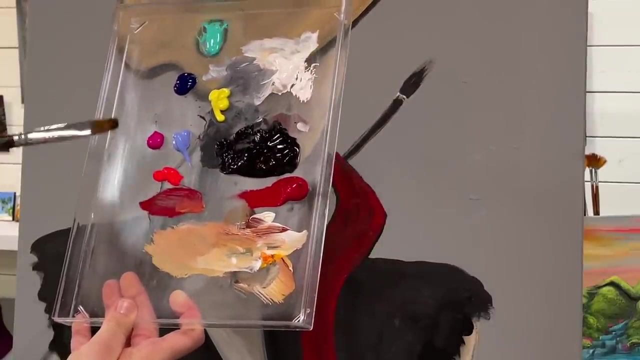 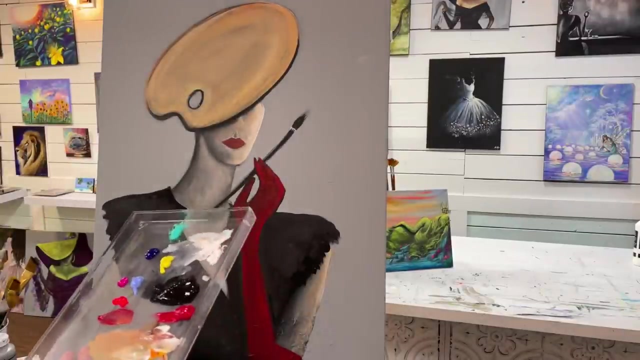 Okay, Okay, Okay, Okay, Okay, Okay, Okay. so I've got a few colors here that I'm going to add. Okay, Okay, Okay, Okay. I want it to look 3d, so I'm going to add the paint thick and I think I'll just 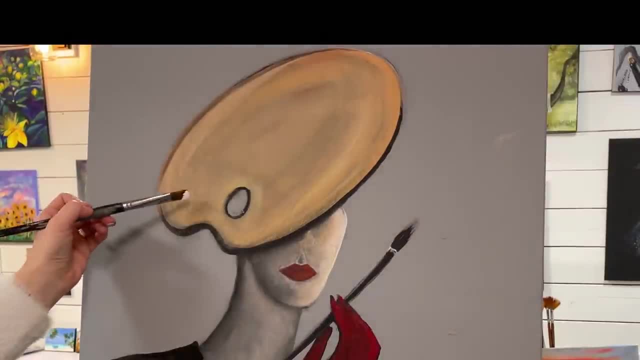 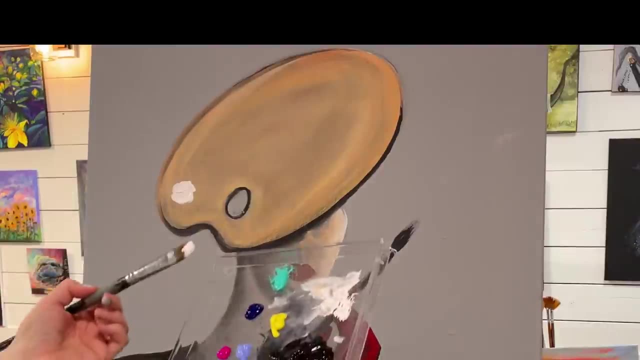 start with a little bit of white, and I'm going to add it really thick on here, right, I want it to look real. and then, with a little bit of white, I'll take my red, add some of that. then I'm going to take my yellow with a little bit of. 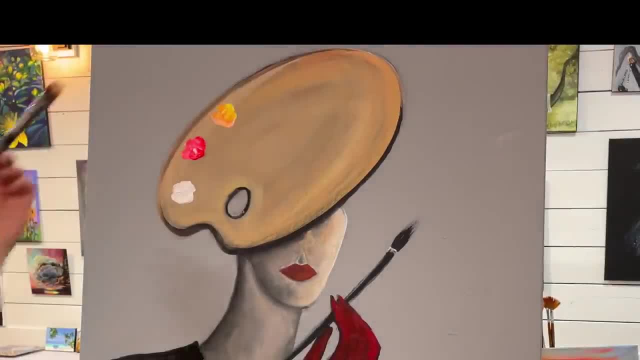 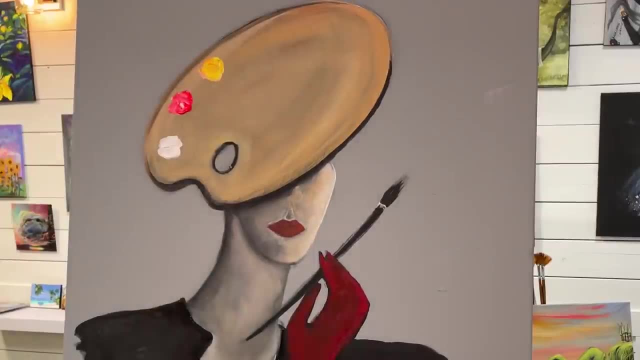 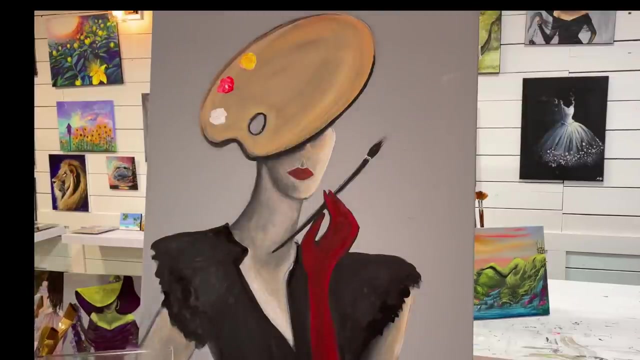 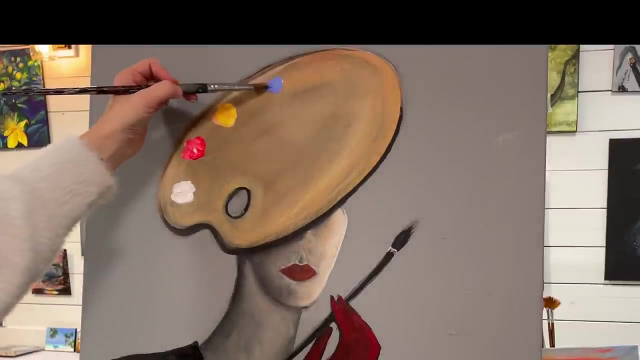 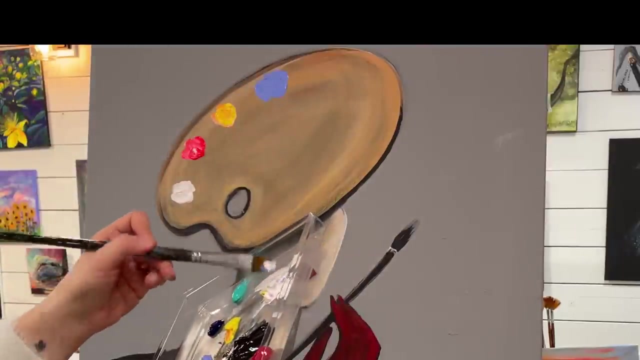 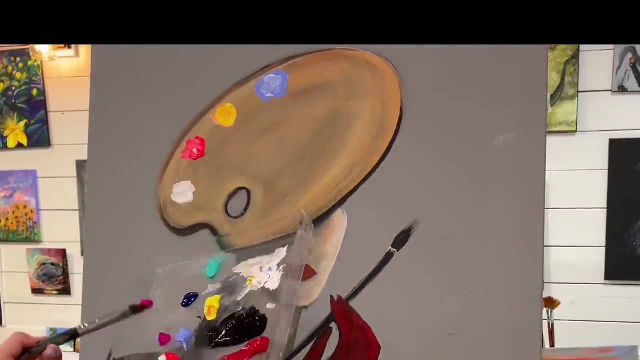 white and that red on there, a little bit more yellow and white, so it's going to have a texture when it dries. okay, then I'm going to take my blue violet. a little bit of white I'm going to take. I'll take my neon violet next. 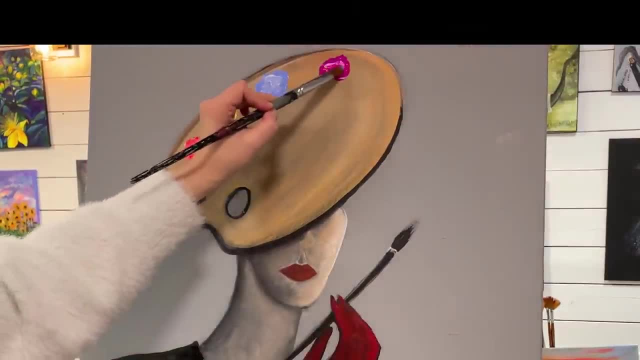 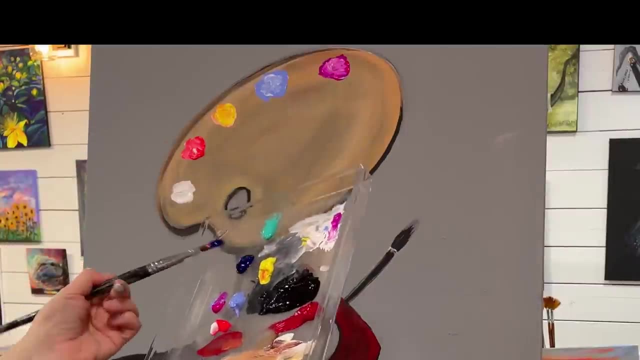 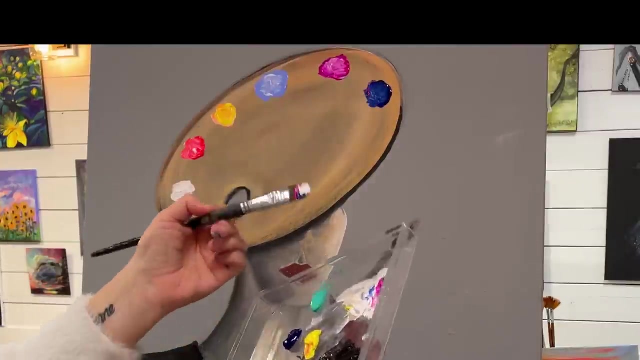 a little bit of white. and then I'm going to add a little bit of red on there, little bit of white with it, and kind of stir that in and mix it up there. then I'm going to take my phthalo blue, add that a little bit of white. I know it's. 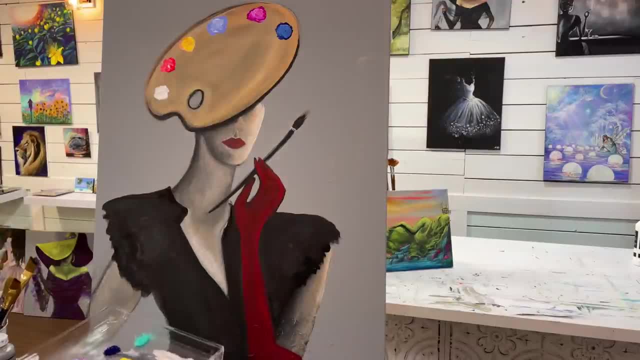 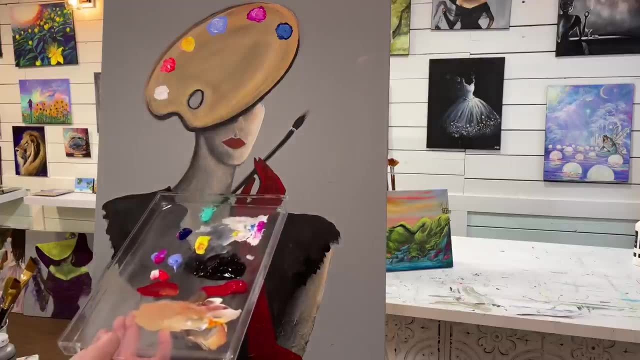 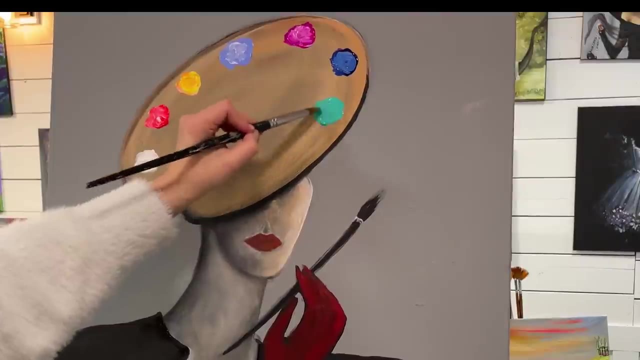 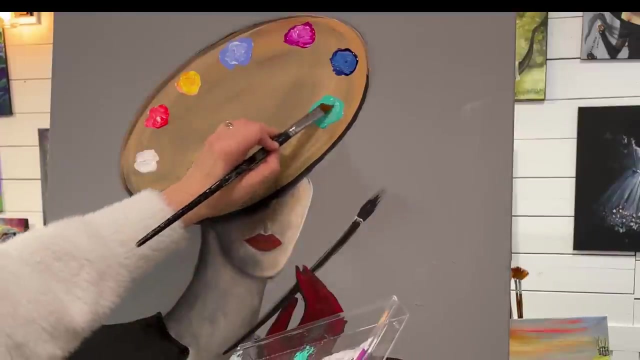 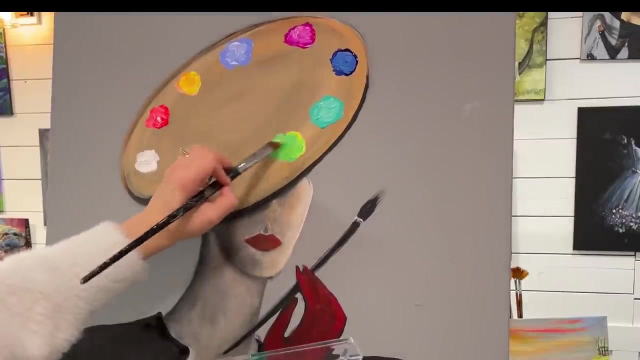 going to dry darker, so I want to make sure that it dries to a bright color. and then I'm going to take turquoise, a little bit more turquoise and a little bit of white, a little bit more. and then I'm going to take yellow. with my turquoise we'll make another shade. I'm 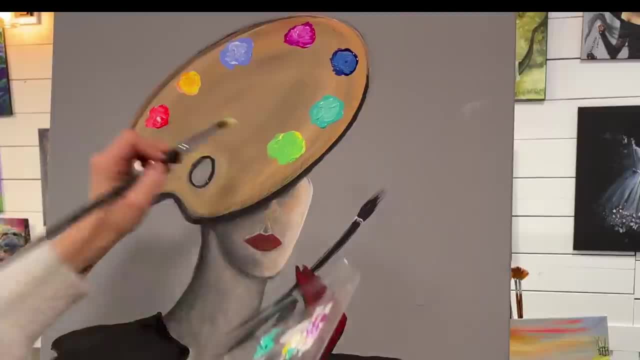 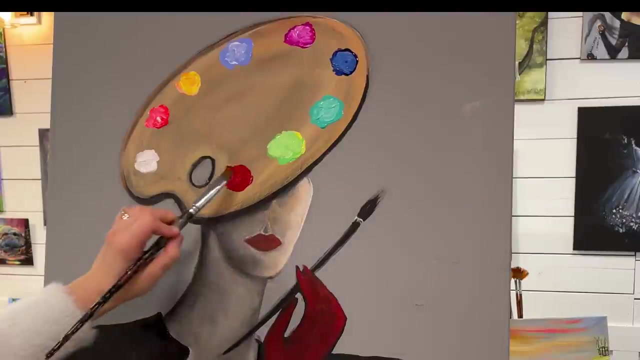 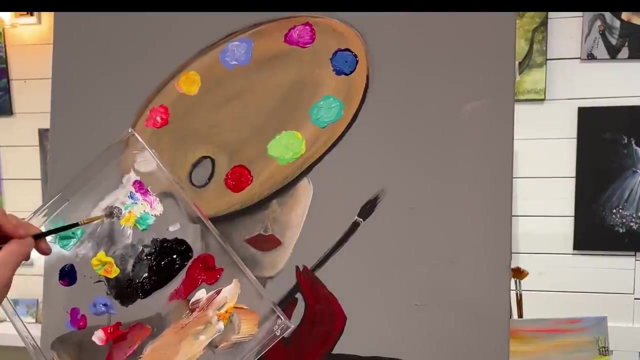 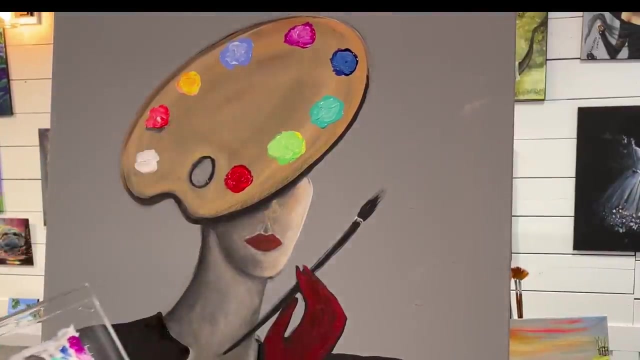 shade could have red. i'm going to add my neon red in there as well, okay, and then the next thing i'm going to do is add just a little bit of a shadow around them all. so i'm just going to make some gray. i'm going to just kind of go around the edge. 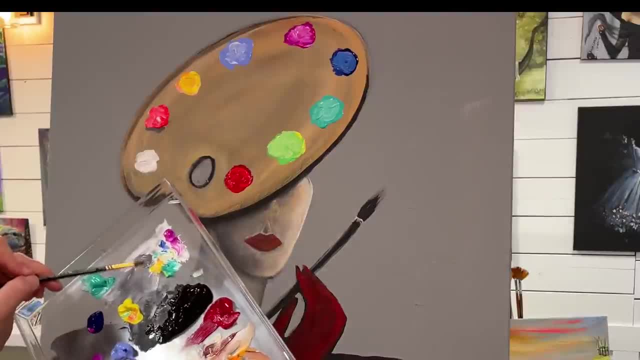 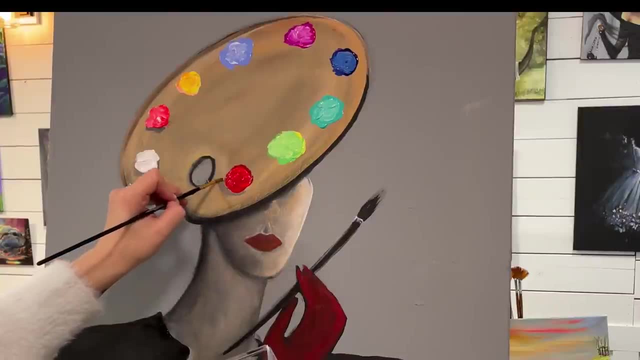 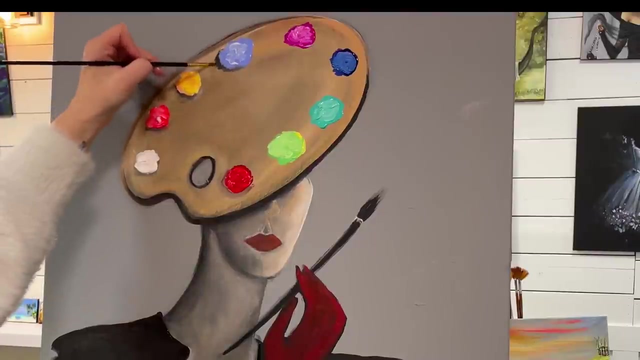 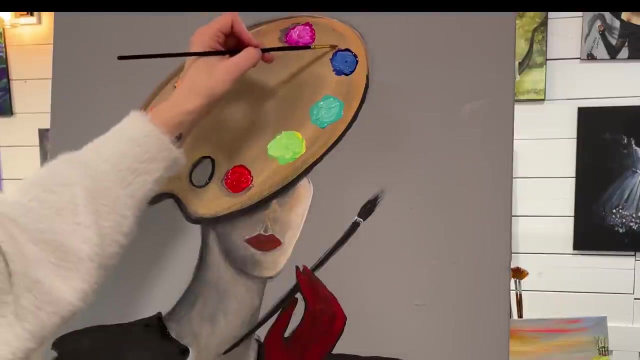 so, uh, you know a little bit more black here, and i'll just scumble around the edges here, loosen some of it off and blend it around, and then i'm just going to add a little bit of a shadow around the edge. same there. so so so. 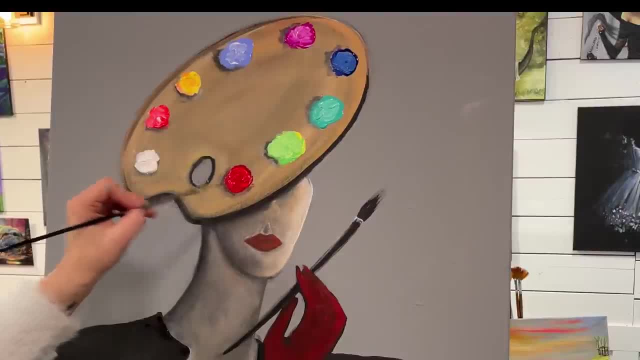 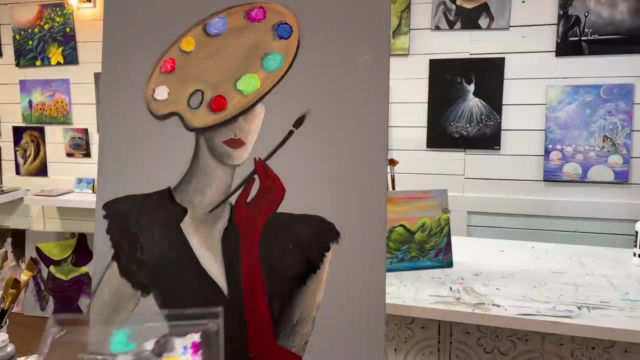 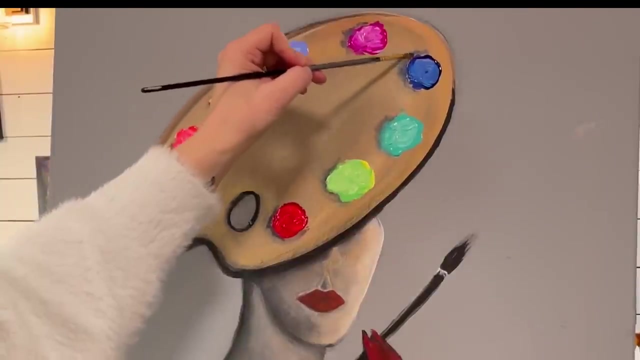 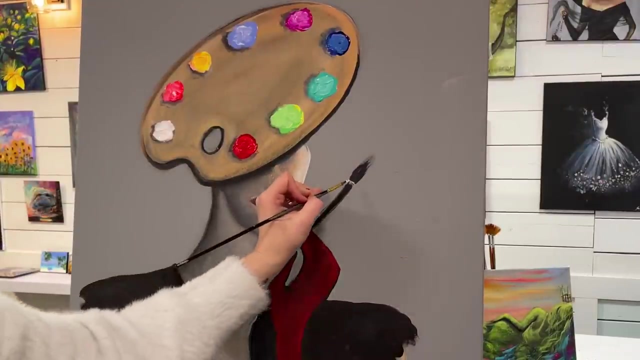 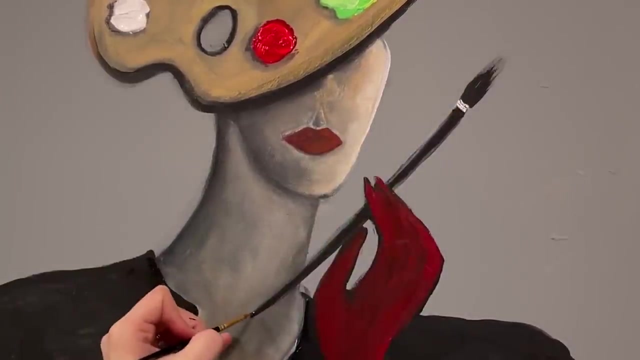 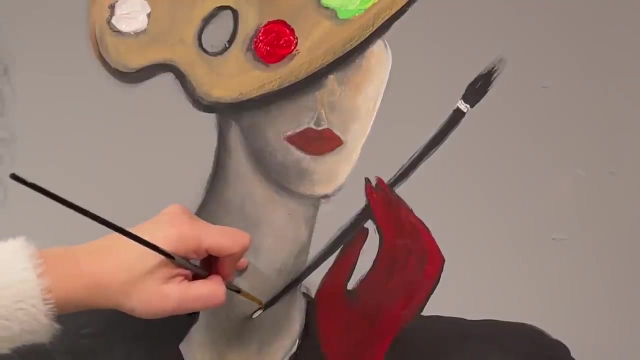 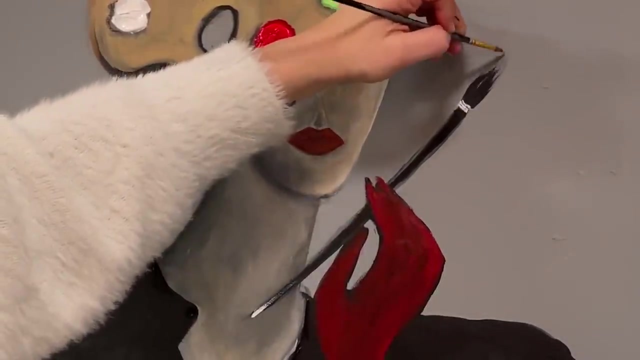 i'll just loosen this up a little bit where it's a little bit too thick and dark. okay, i'm going to take some white now and i'm just going to add a little line here and then a little little dab on the end. so, and i think i'll add a few colors on my paintbrush as well. 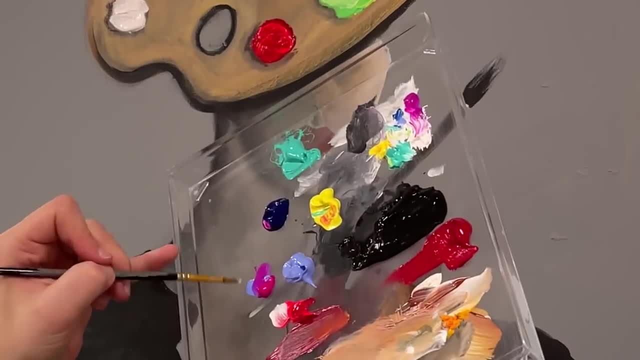 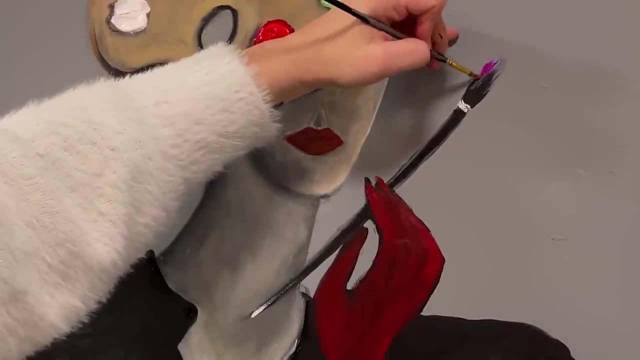 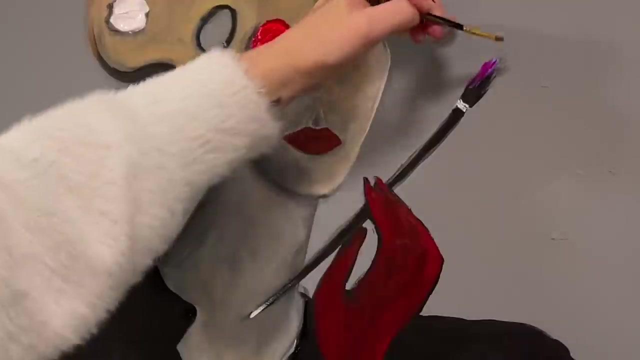 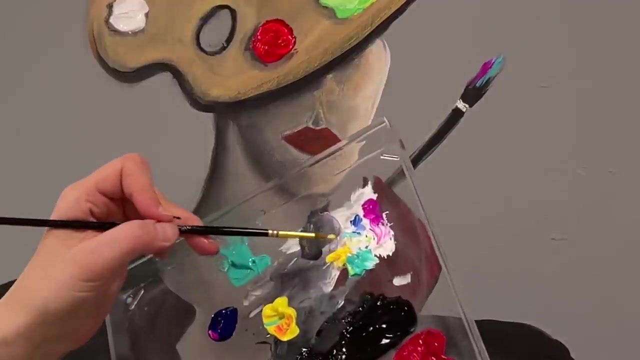 i think i'll take a little bit of that violet, both of those violets, and a little bit of turquoise, a little bit of yellow. so okay, a little bit of yellow. i've got a bit of white in here too with the yellow, just so that it dries. 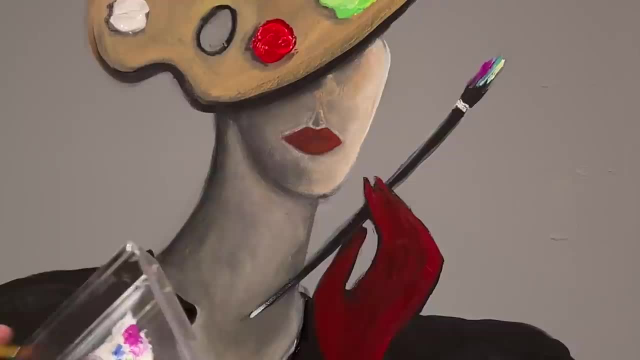 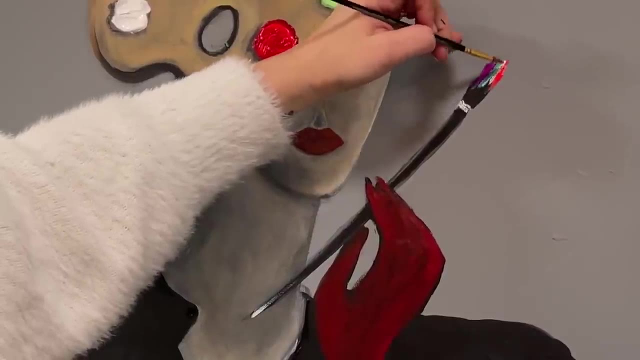 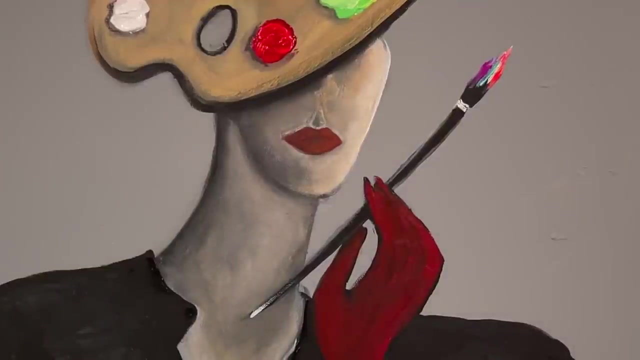 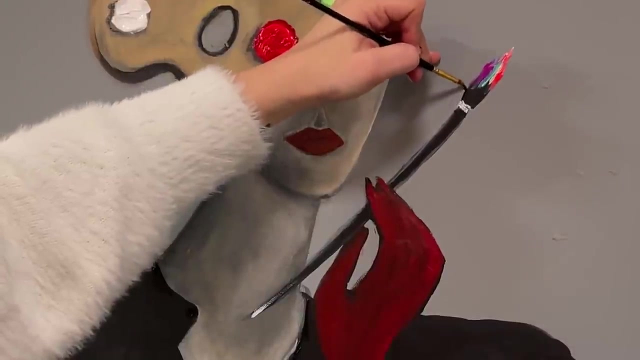 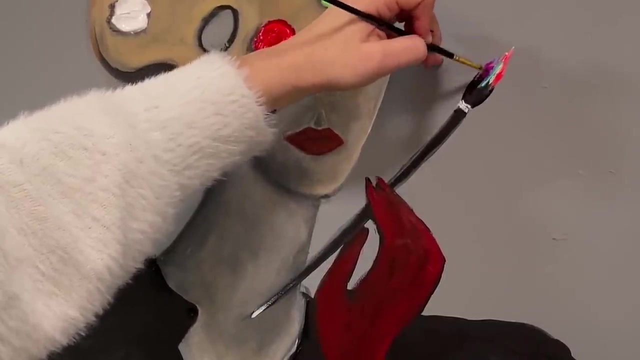 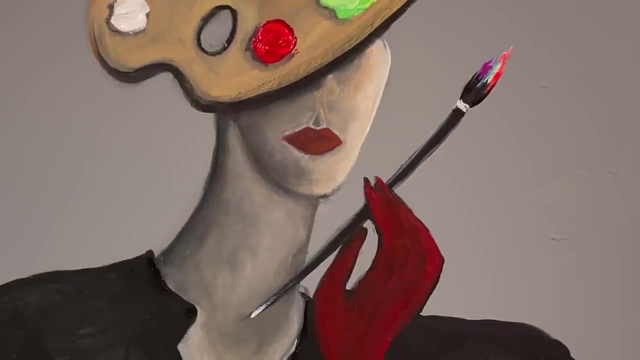 to a nice bright color, and then i'll take a little bit of my red. i'm just going to take my black and bring it out a little bit, and here i think there would be a little bit of a shadow right in here. so i'm going to take my red with a little bit of black. 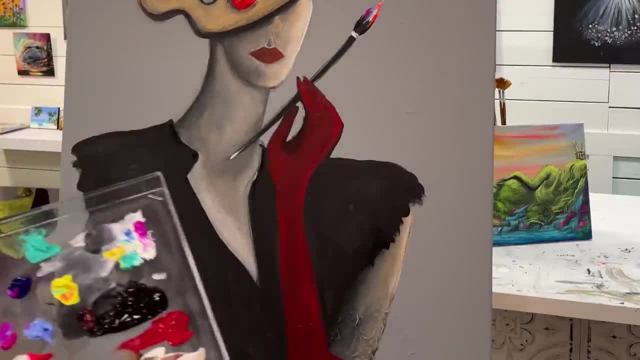 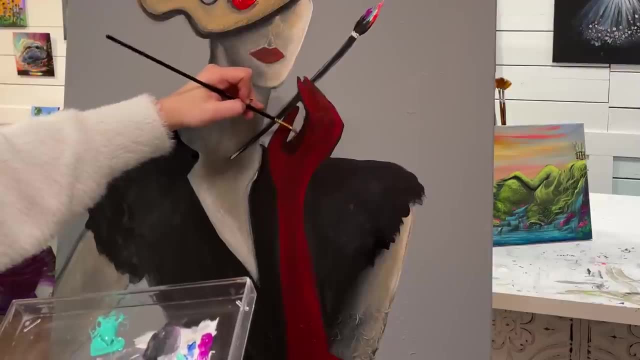 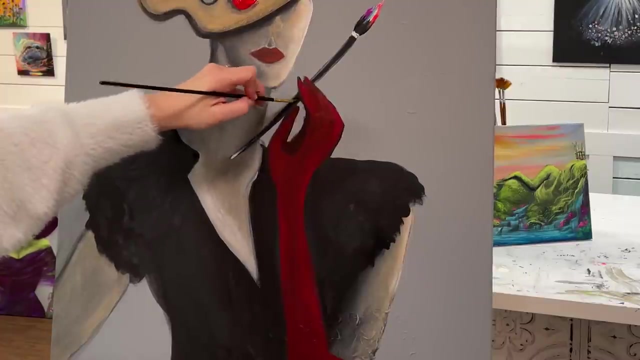 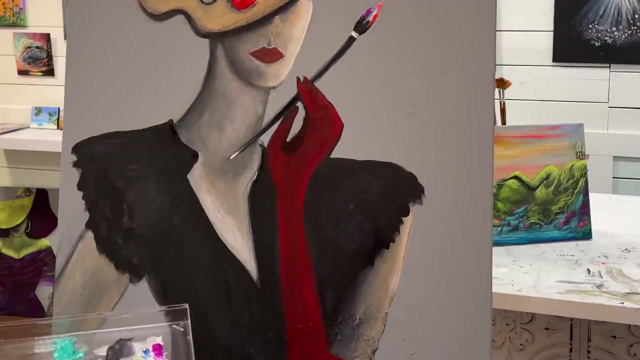 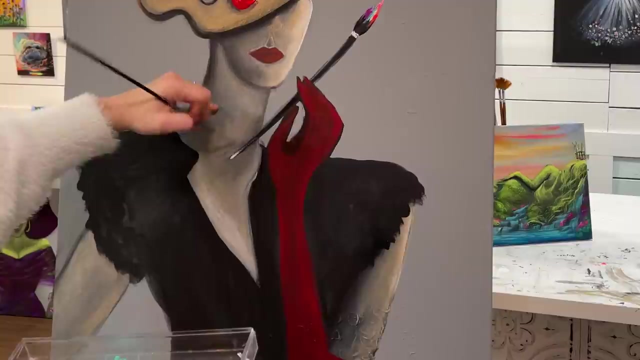 so we're going to have a shadow on her neck from the paintbrush. so i'm just going to do a little black line, light, very light. i'll just make kind of a dark gray color here. it's going to be shadow here from her hand on the side of her neck. 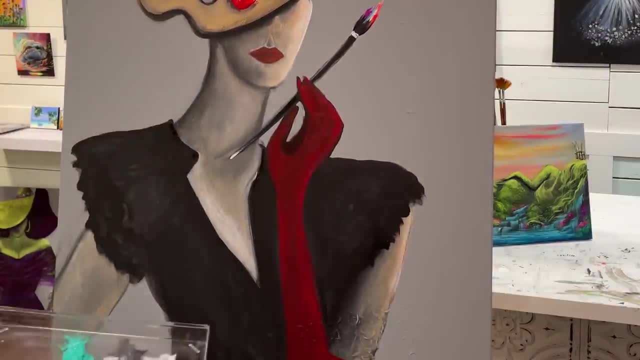 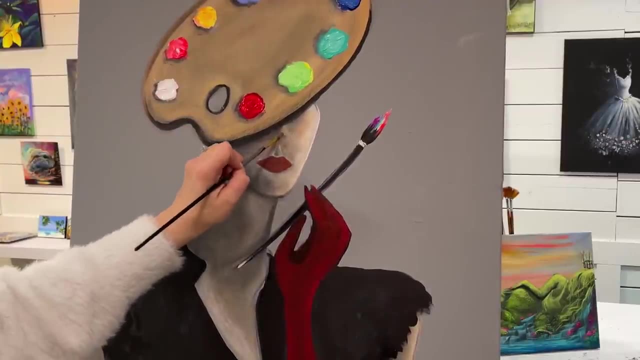 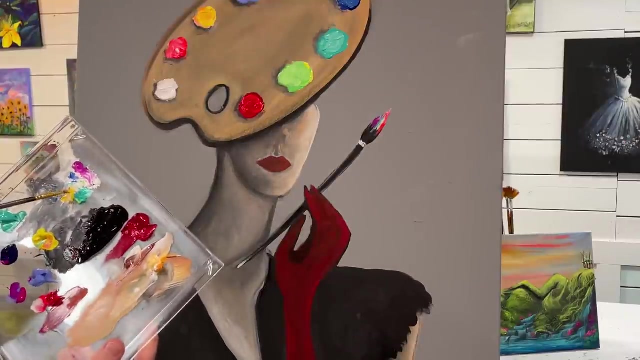 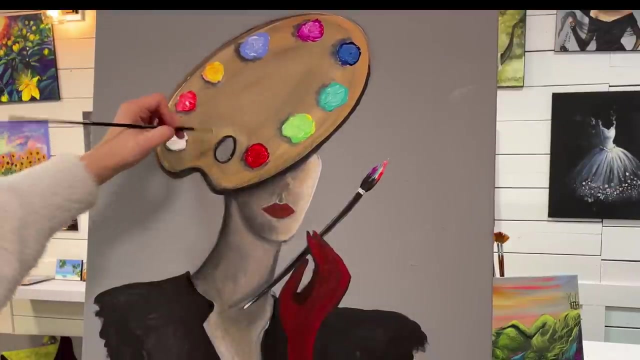 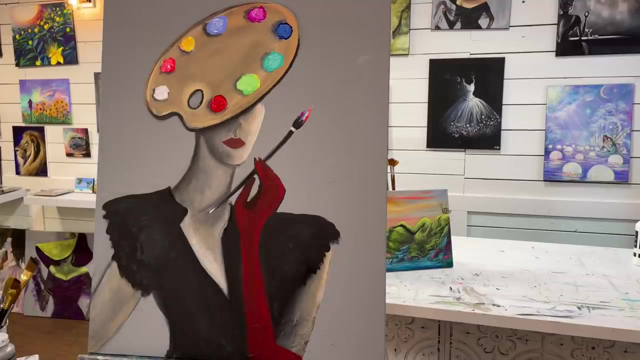 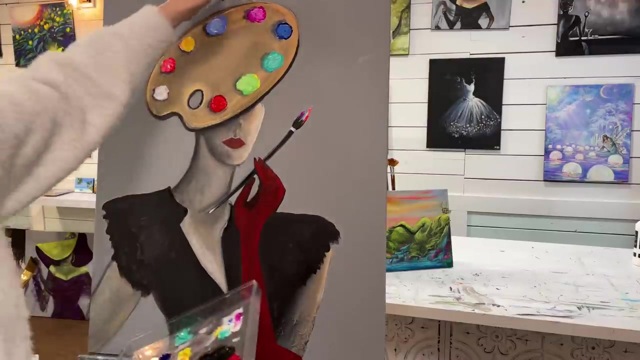 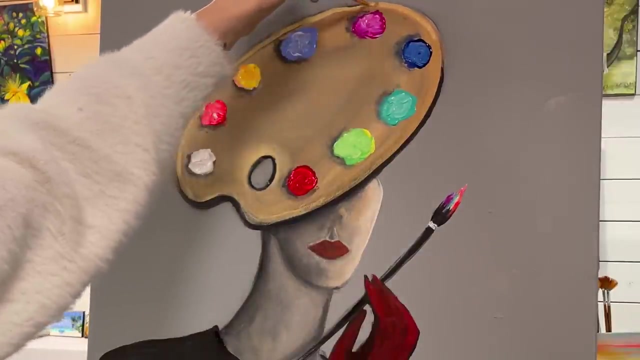 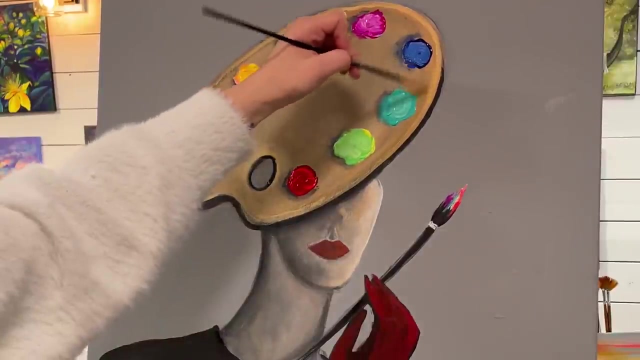 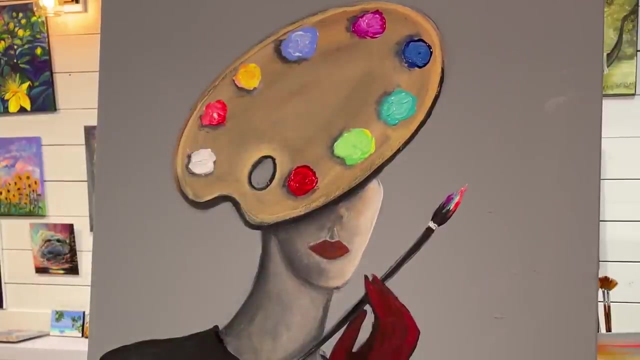 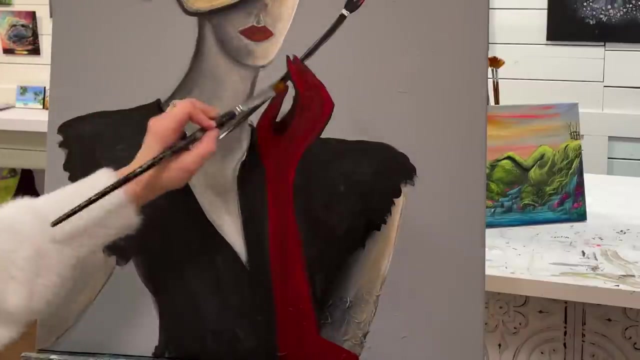 and then the paintbrush and i'm going to go around the edge of the palette. okay, and i'm going to go around the edge of the palette with my highlight colors. so so I'm going to add a little bit of color. I'm going to add a little bit of my neon red here for a highlight. make it look a little more velvety. 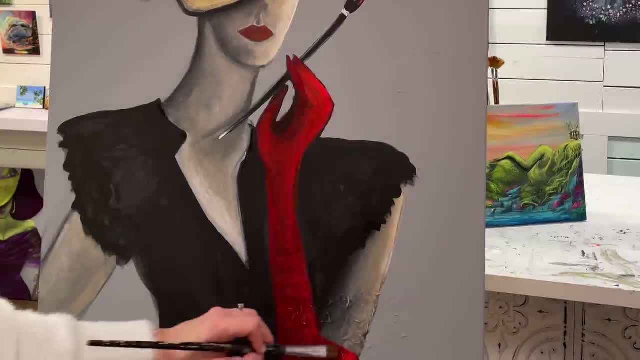 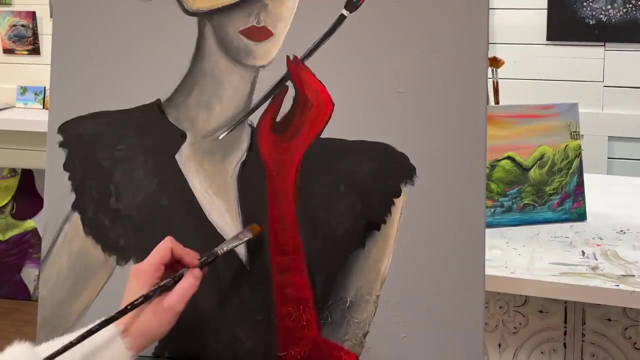 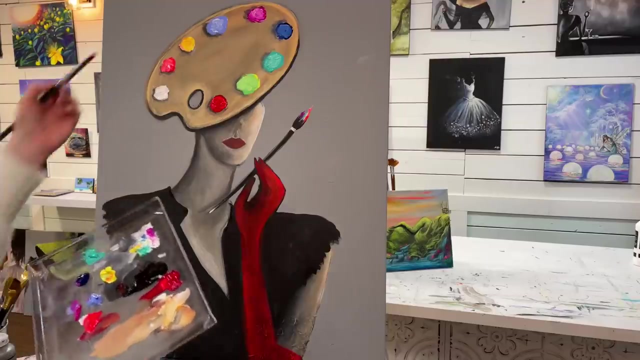 So I've got this underpainting. I can't remember what it was, but it almost looks like. I have roses that I previously painted and I love the pattern it's creating on the glove. I think it would be neat to make it look like there's some drips coming down. 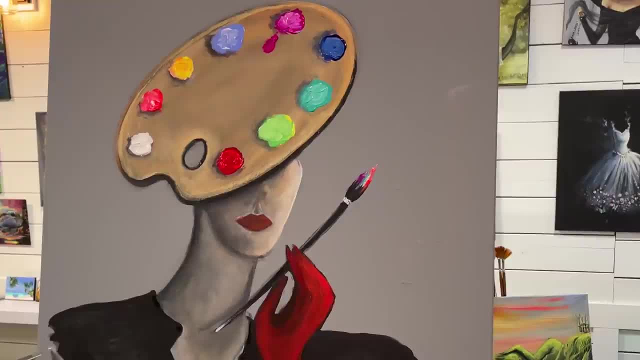 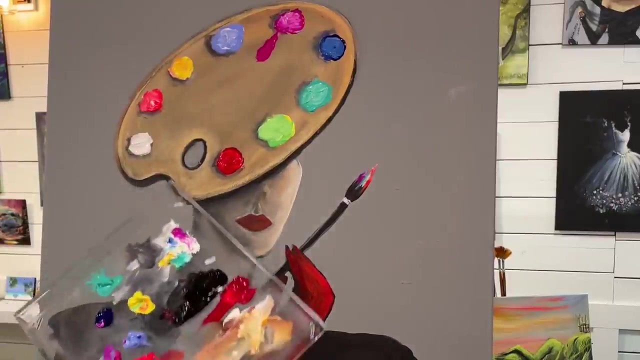 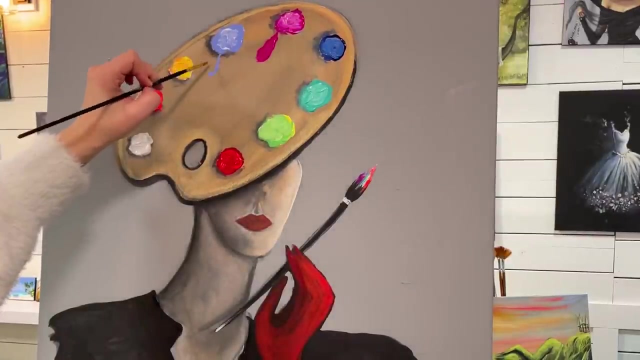 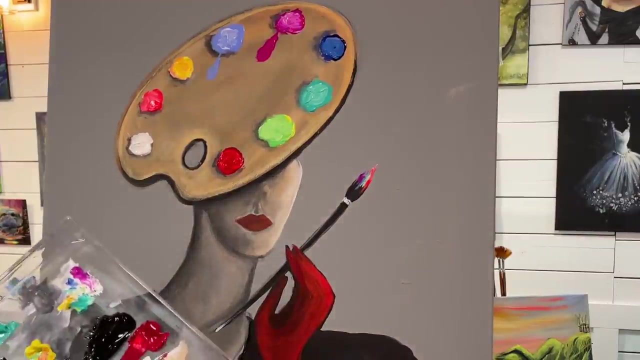 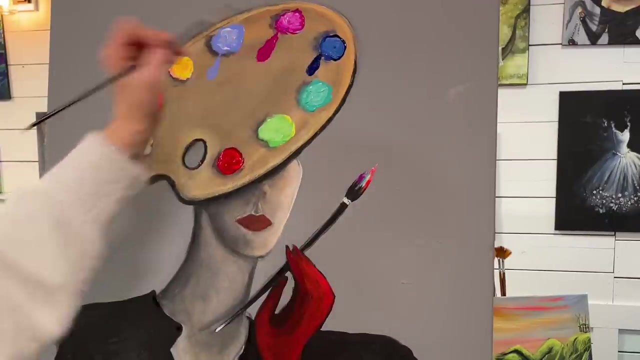 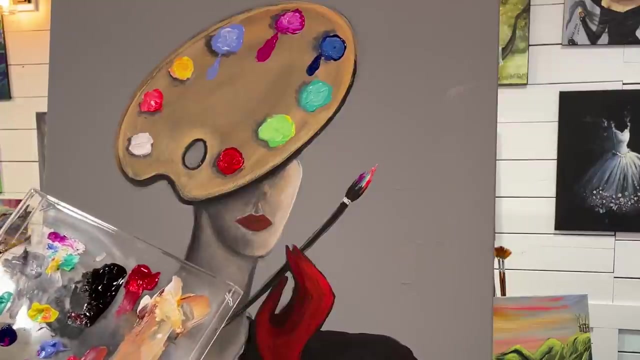 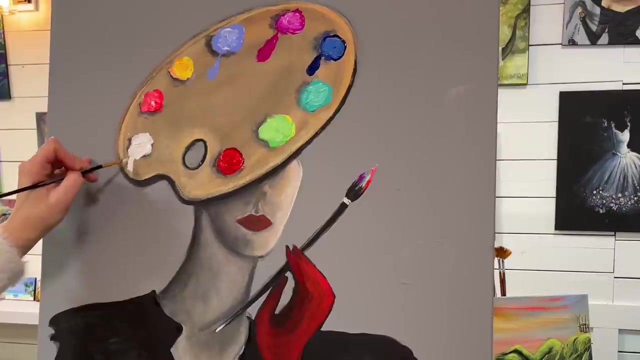 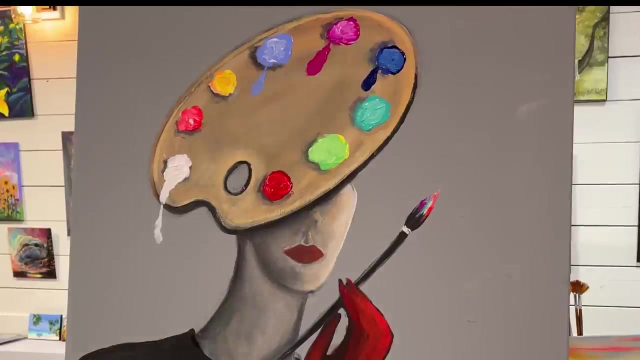 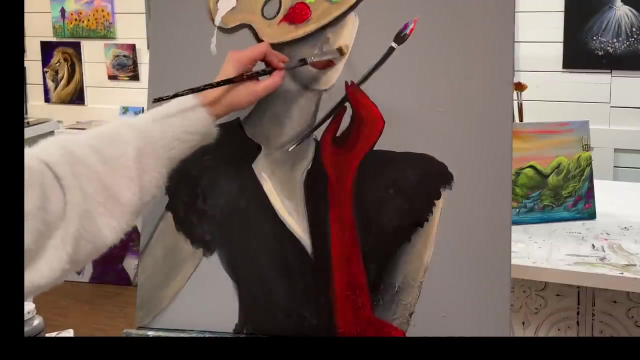 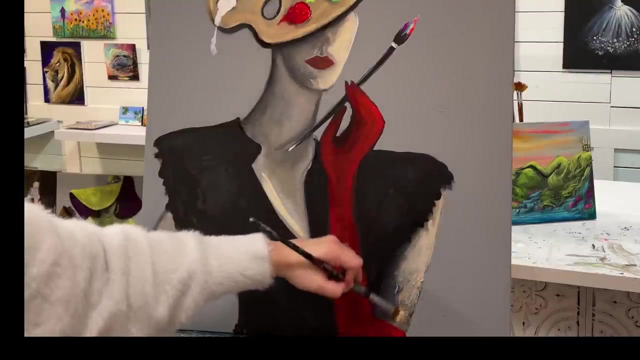 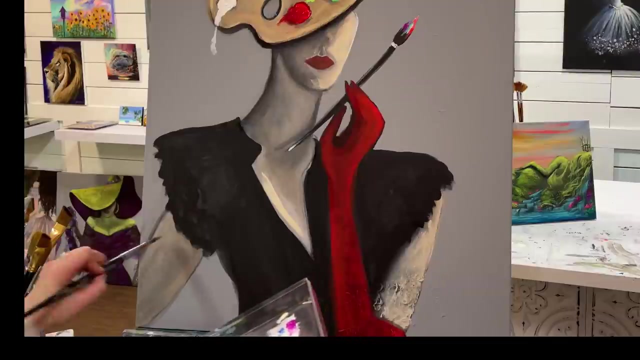 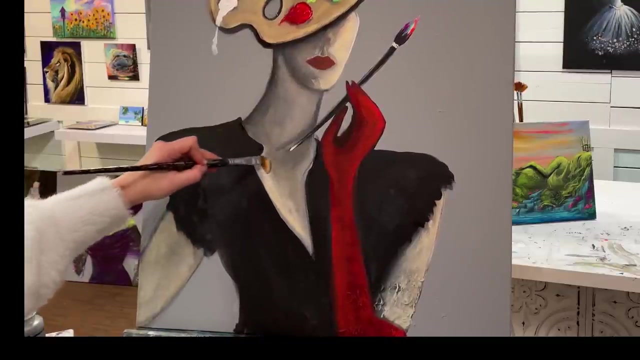 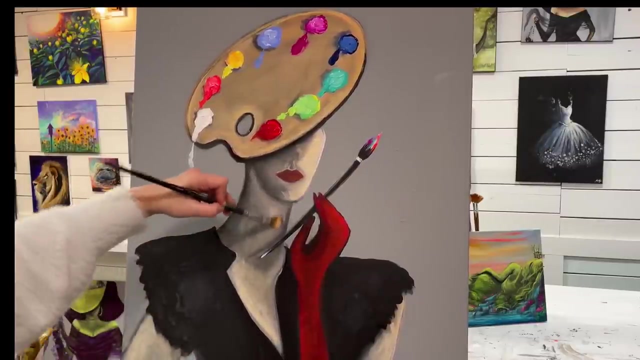 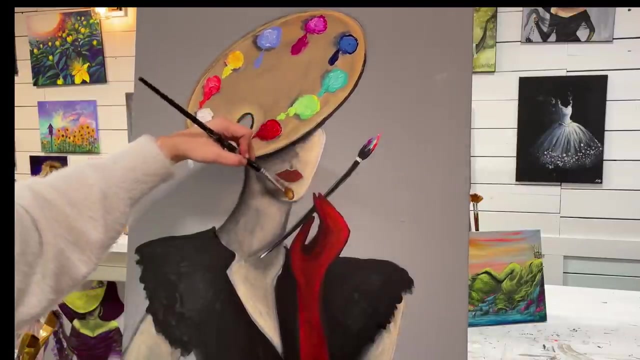 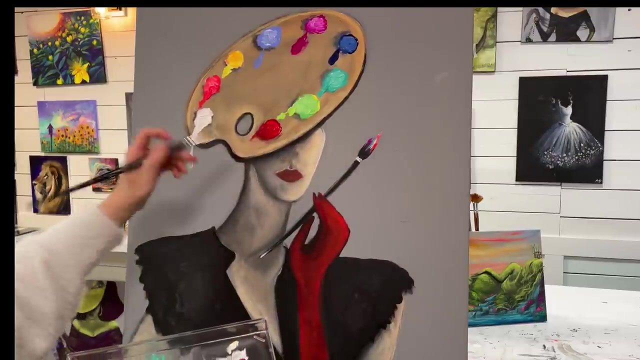 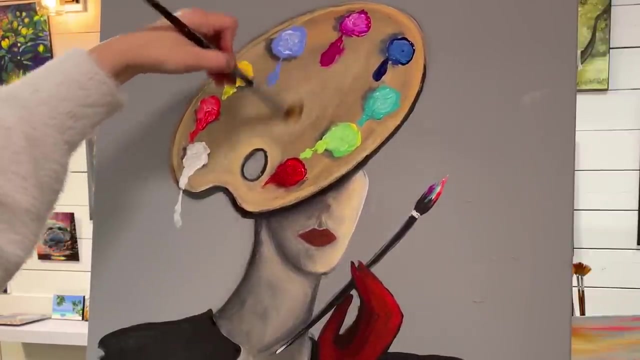 So I might do that on a few of these. I will take my number two round brush again and make it look like starting to drip down here, and then I'll take my blue, violet and do the same, my white, a few more highlights. I'm just going to get a little bit of a highlight here to make it look shiny, and I'm going to 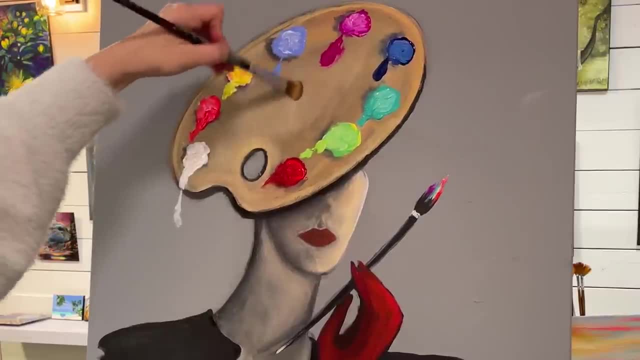 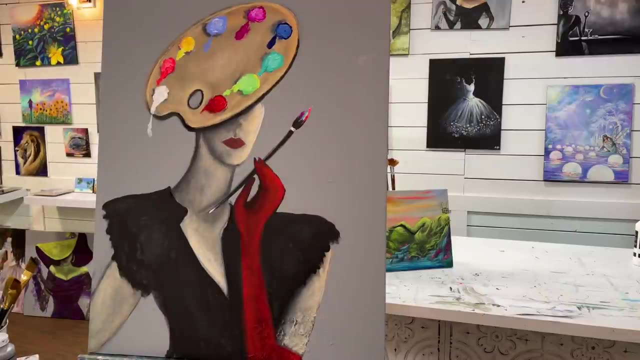 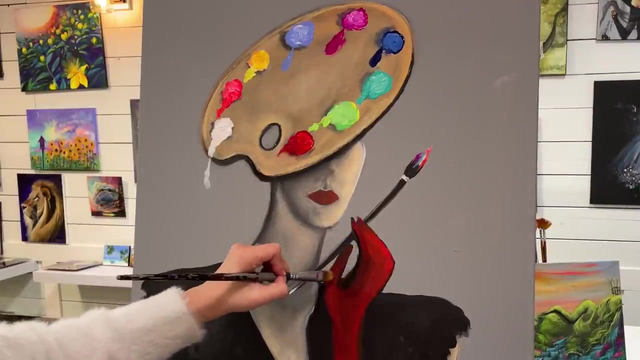 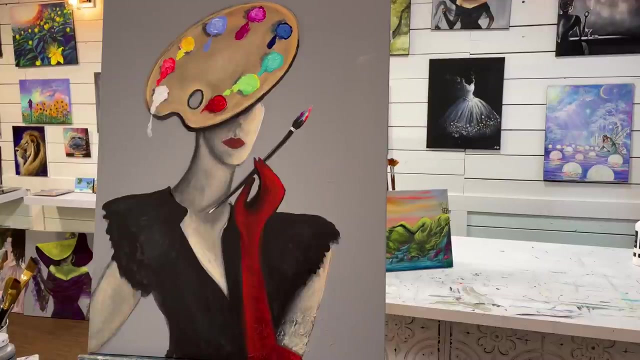 do it on a slant like this, and then I'm going to go ahead and take my blue violet. okay, I really really love painting this. this was fun. I kind of just did this out of my head, so it's probably why the proportions are a little bit off.